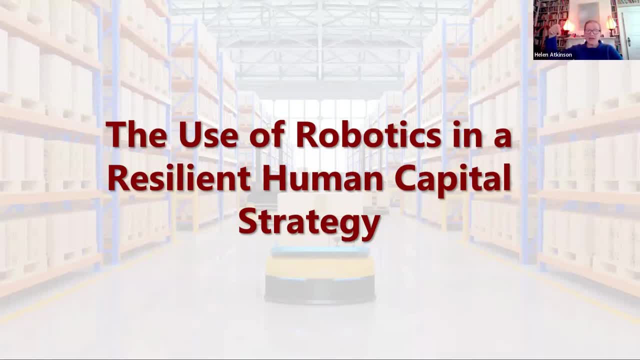 the audience. Please submit questions at any time using the tab at the bottom of your screen. We will not be using people's titles or company names, so go ahead and ask anything you like. If you don't see your question come up during the webinar, please be assured we will reach out to. 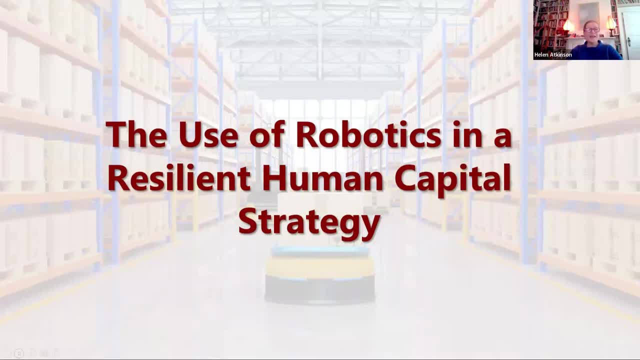 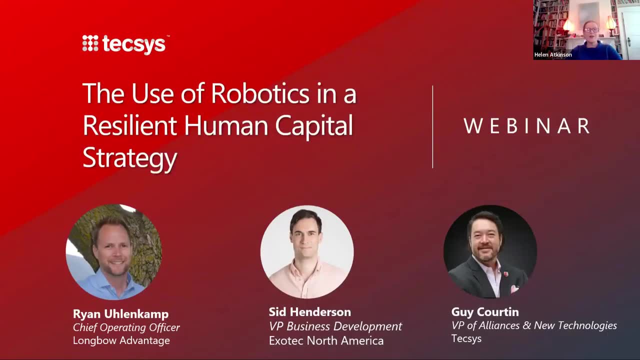 you offline. See you Liszt, right. let's get to our panelists. Guy Cortin is Vice President of Industry and Advanced Technology at Texas, an omni-channel supply chain technology provider, where he leads Texas's advanced technology and automation go-to-market strategy. In addition, for a long time he's been an industry. 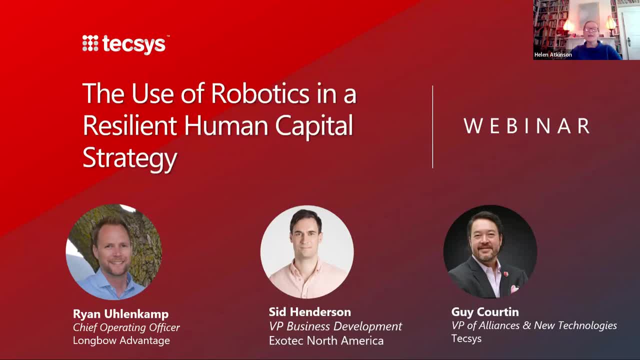 analyst covering the supply chain and retail spaces for SCM World. Sid Henderson is the Vice President of Business Development for Exotech North America. He comes to Exotech from robotics provider Osaro, where he oversaw international sales, And then, finally, we have Ryan Ullenkamp. 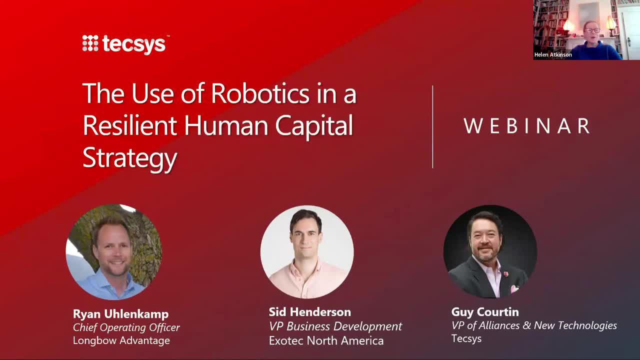 who is Chief Operating Officer at Longbow Advantage. Ryan works closely with customers and WMS providers to create innovative solutions that help warehouse operators define and execute on both their near and long-term development goals. Welcome, gentlemen, Let's get into the panel session. 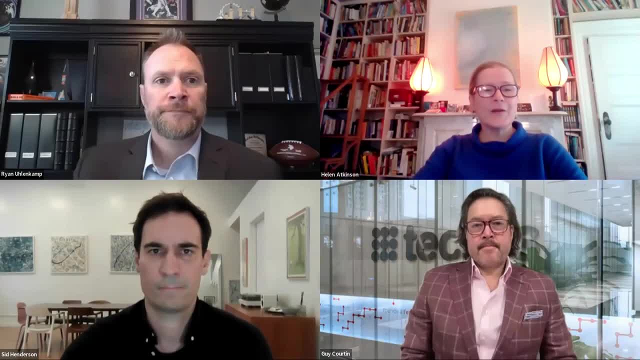 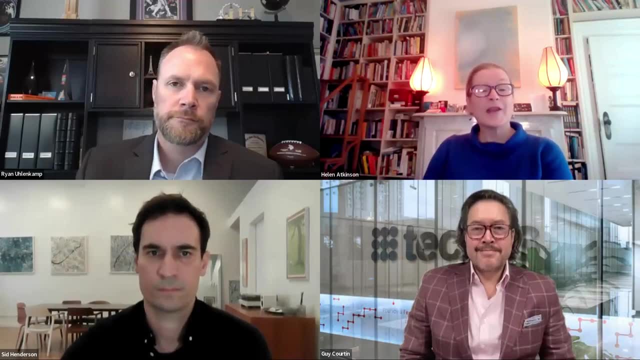 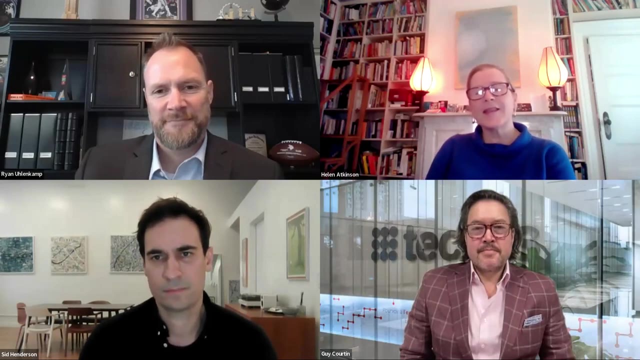 So, Sid, I've got a question for you. Looking back to the beginning of this year, automation was definitely all the rage, especially in the media, like supply chain brain- I know I've been writing about it a lot Now- it's tended to take a bit of a backseat to things like AI and machine learning. 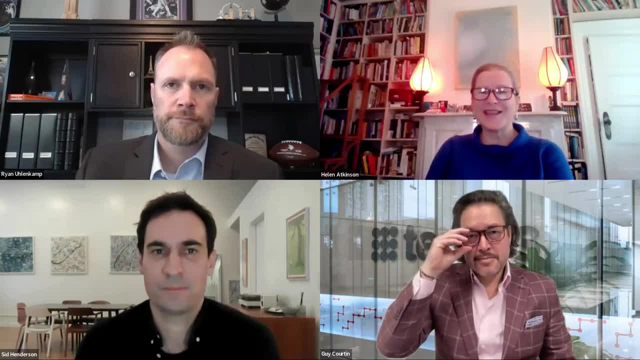 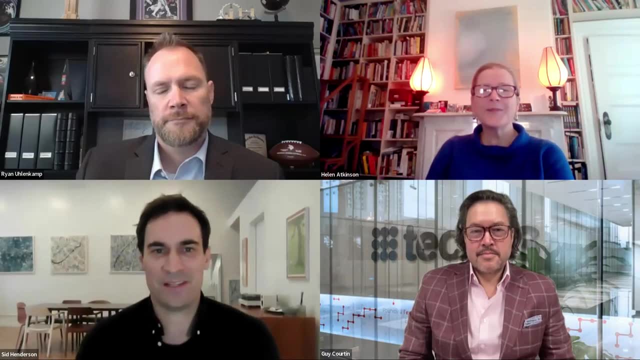 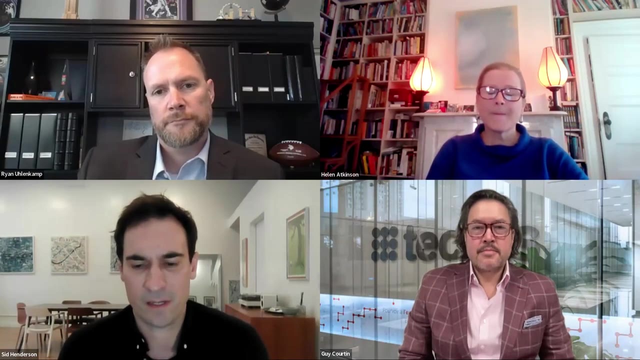 Was it all just hype? What's happening with automation and distribution? Very good question, Helen. No, automation is definitely not hype. I'd say the demand in our space is really based on the steady macro trends that have been continuing to move in the same. 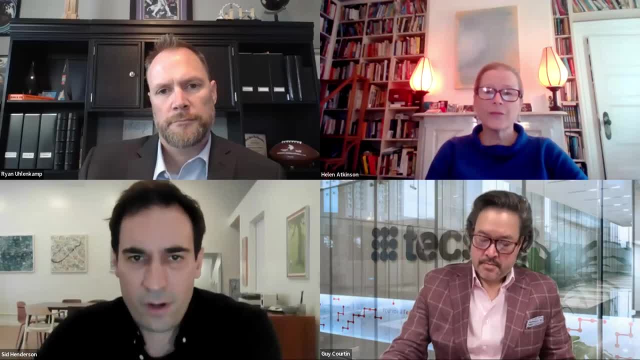 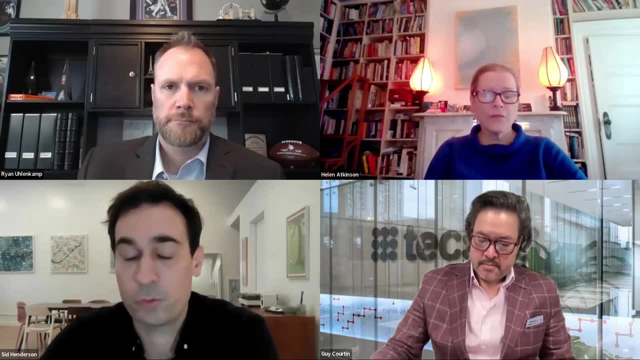 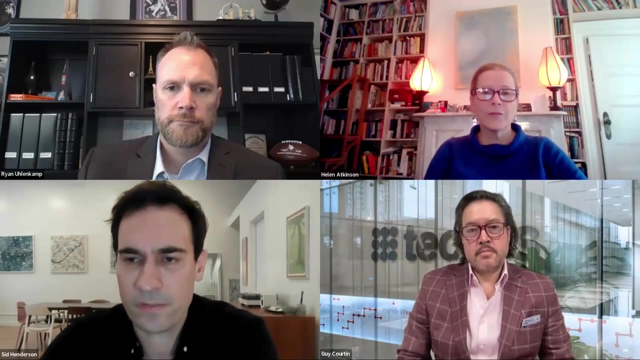 direction for a while now. These are trends like rapidly aging population, rising labor costs, growing cost of industrial space, higher customer expectations. So I think it's really these trends, more than anything, that are really driving our customers to invest in automation. So the underlying demand it isn't going away. 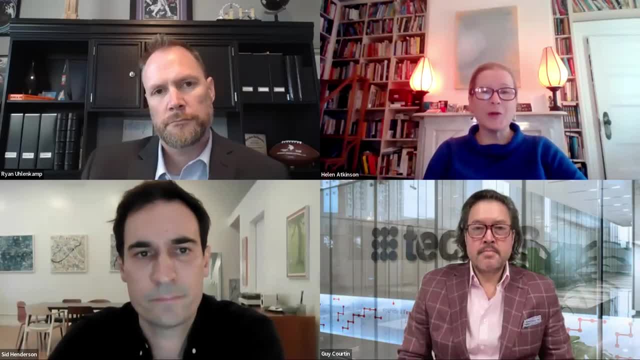 Right, So that's interesting. So not only do we not have enough people, but we need to be packing more distribution. So we need to be packing more distribution. So we need to be packing more automation operations into the space available. Is that right? 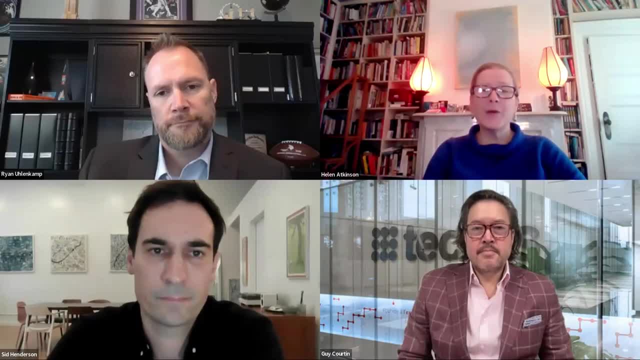 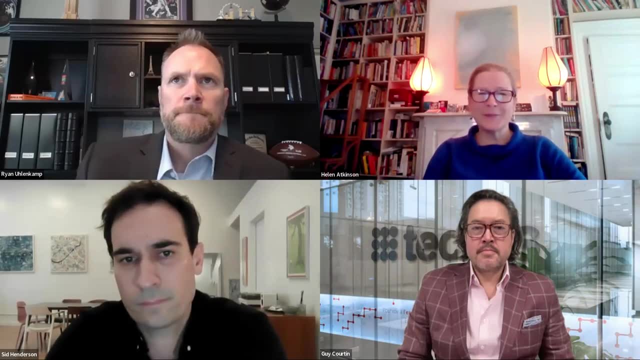 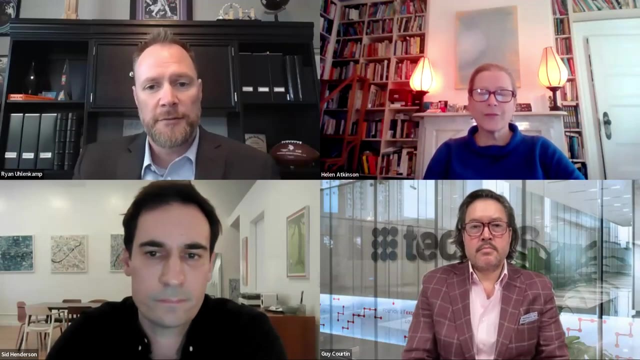 I couldn't agree more. Yeah, Yeah, Ryan. what do you think about that? Is the demand for automation increasing at present? I think, yeah, the demand for automation is increasing. I think it's a hybrid, though, to bring automation and the workforce together for sure. 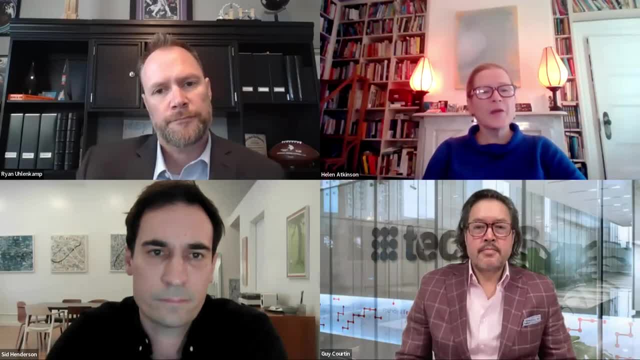 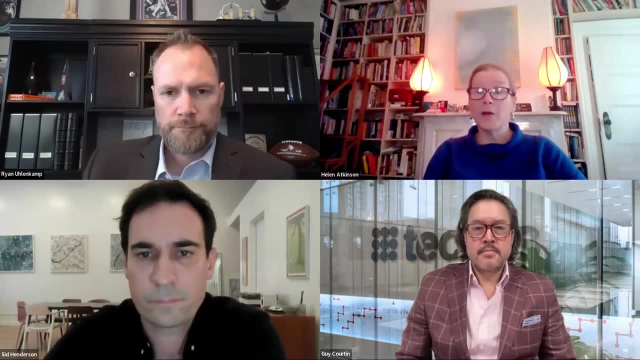 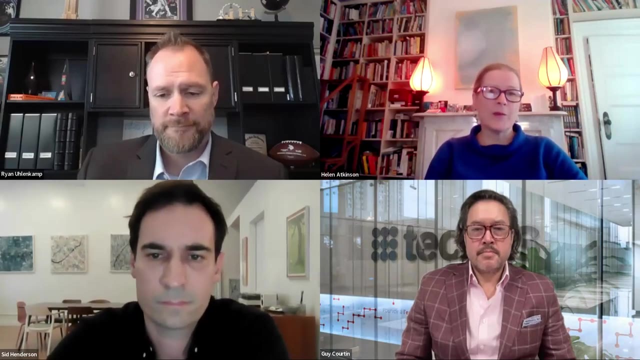 Right, Right. So one of the drivers of the automation discourse was the fact that labor was expensive and getting more expensive, And I know we've just had the United Auto Workers agree a huge pay rise with the big three, And I see Toyota has now followed suit. So 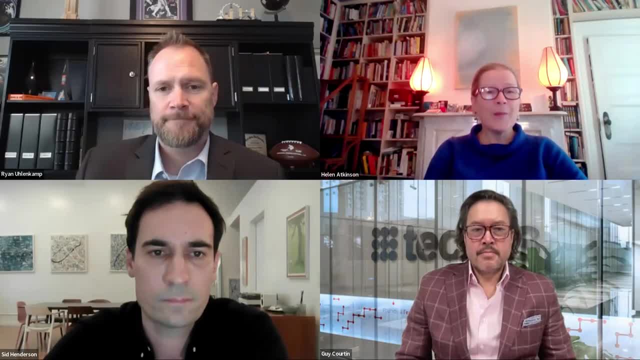 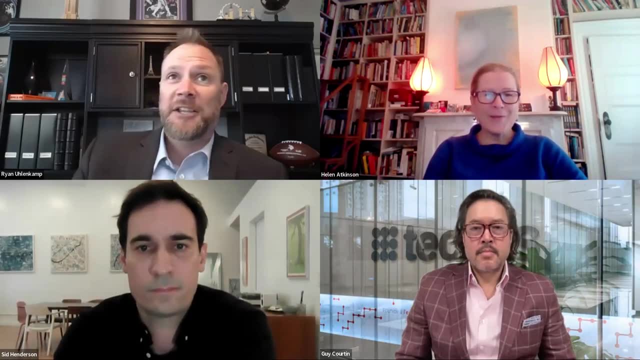 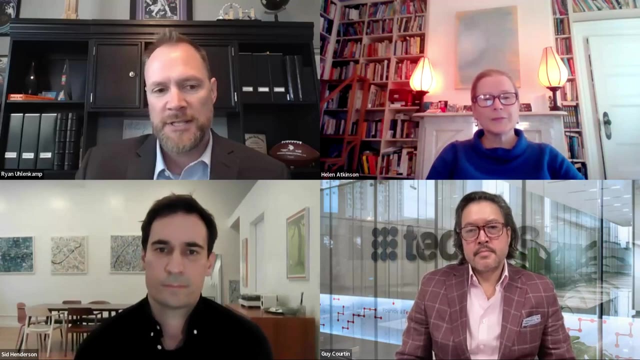 wages are definitely going to go up. So, since this is the case, how are warehouse managers coping? Yeah, I think the- I mean that labor challenge still exists. To your point, like the market is still very expensive, very competitive, right? So? 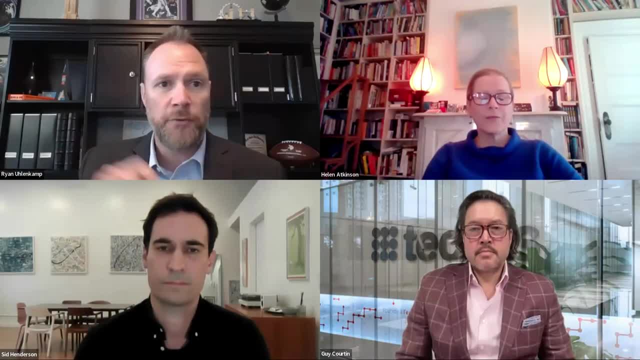 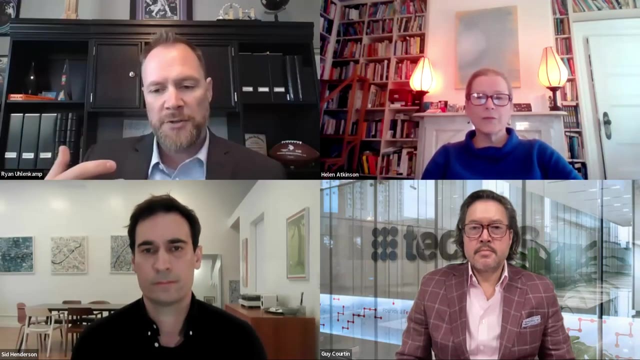 engagement with your associates, I think, becomes critical for a warehouse manager, showing that you're understanding their job and able to coach right. So engaging with associates, coaching them not just to retain your current workforce but actually, as you bring in new hires, to set that cultural differentiation. 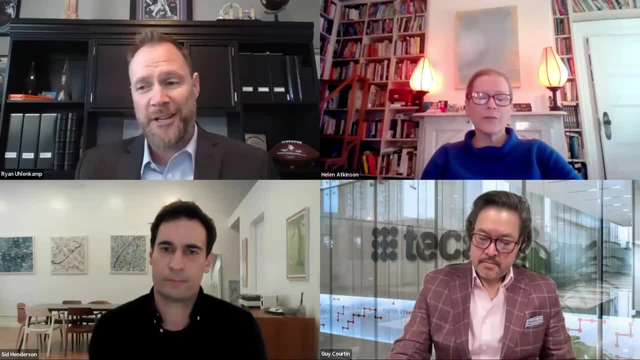 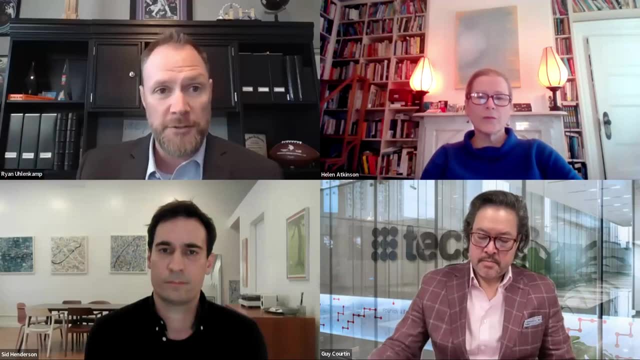 that new hires see: oh, this, this is different. You actually care about what I do, You understand what I'm doing. So I think the role of a warehouse manager over the last few years, but even 10 years or 20 years, 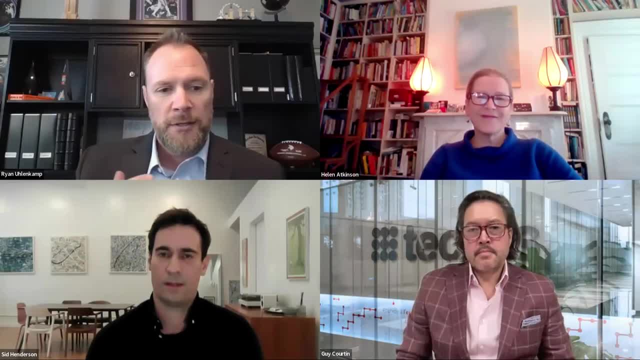 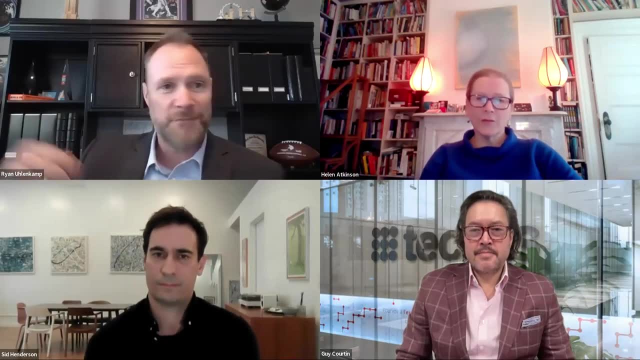 has really changed. I mean, when I first started 20 years ago, you would have standards and performance management And if you didn't meet it you were fired. And I had a backlog of labor resource that I pull up and I train and I just keep turning through. Clearly not the case anymore. 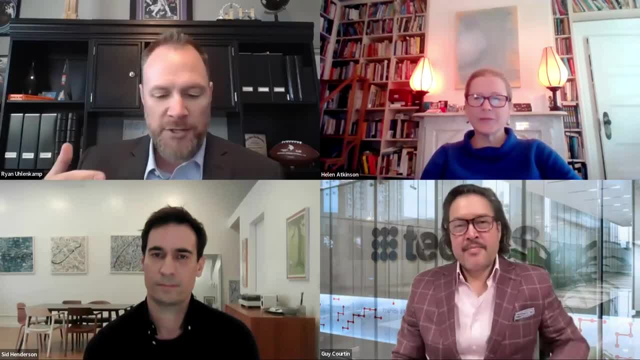 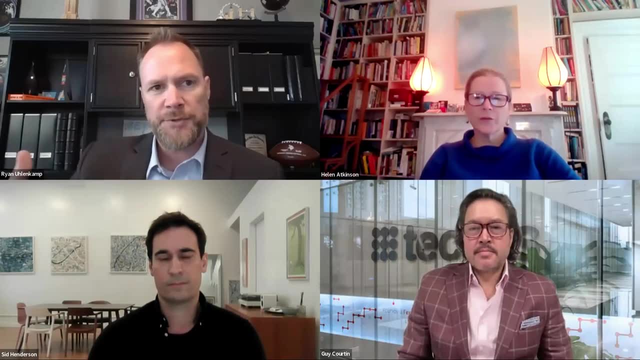 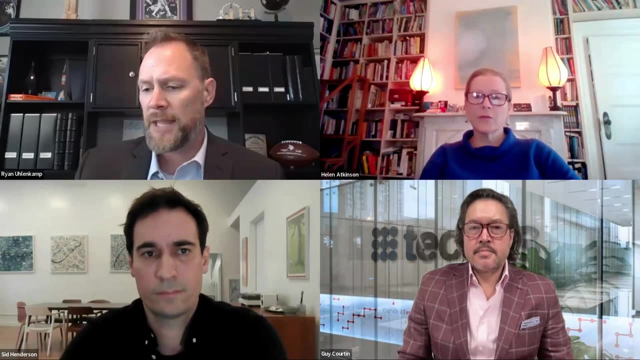 So I think your warehouse managers are they're becoming more engaged leaders. I think they're becoming better coaches. I think they're working to understand their people's challenges more, And they do that through better data, better tools, better visibility into the operation. I think bringing 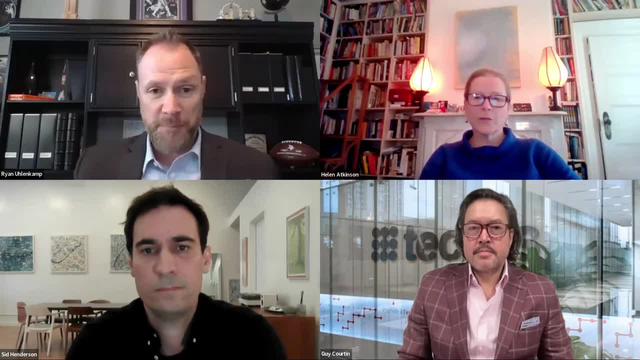 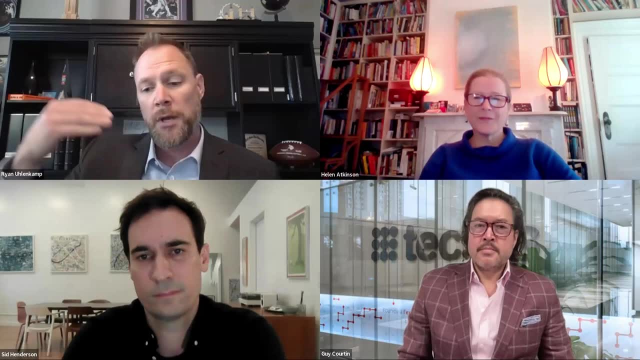 that to the forefront and getting managers out of Excel spreadsheets where they're trying to crunch numbers and figure out what the problem was, bringing that right to them saying there are issues here. go, be more proactive, get out on the floor. That's the unlock And I think that's. 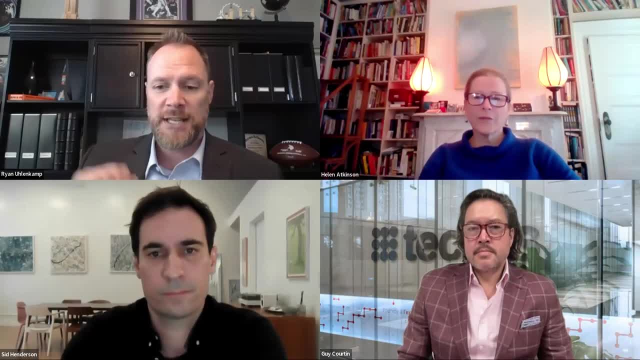 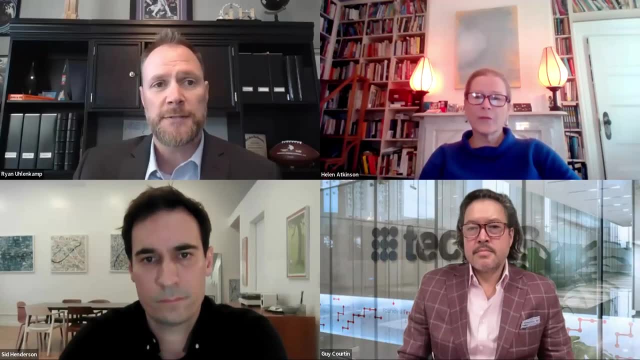 what warehouse managers are trying to do to cope with it is get out of spreadsheets, get on the floor and have data at their hand to better coach and train and engage with their associates, Right? So dare I use the term emotional intelligence? Is that what we're looking at? 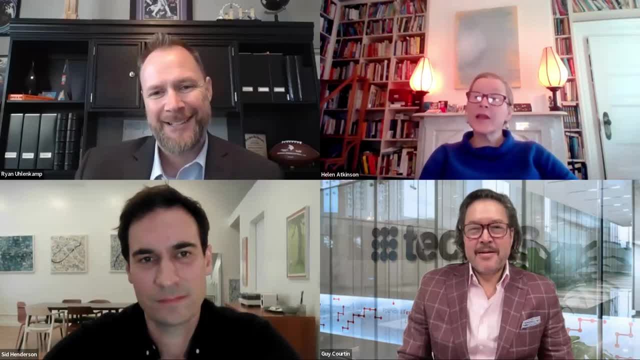 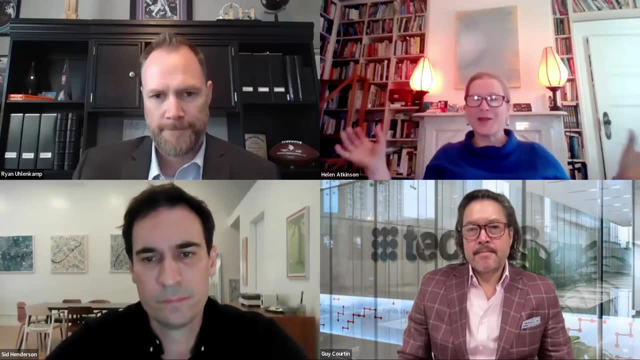 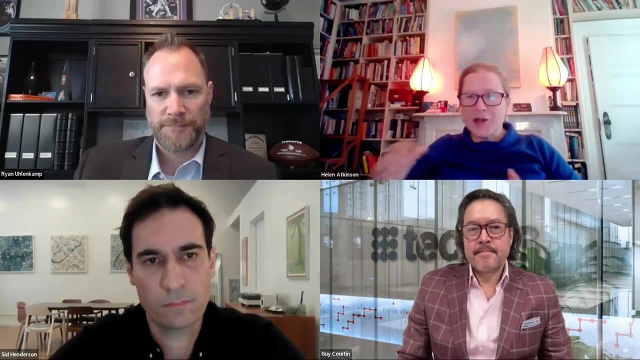 It's a good term to use, Yes, Fantastic. But also this idea of being able to access data in real time while you're on the floor, not just sitting in. you know typical. the typical warehouse manager has this sort of bird's eye, you know sort of nest where the manager looks through a. 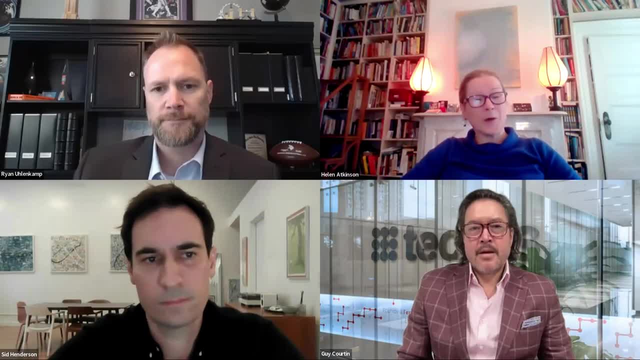 window at what the workers are doing And that sounds like that's just not going to fly anymore, As it were. That's great. I was going to say to Bill what Ryan was saying- I think it's spot on- and to what you just said. 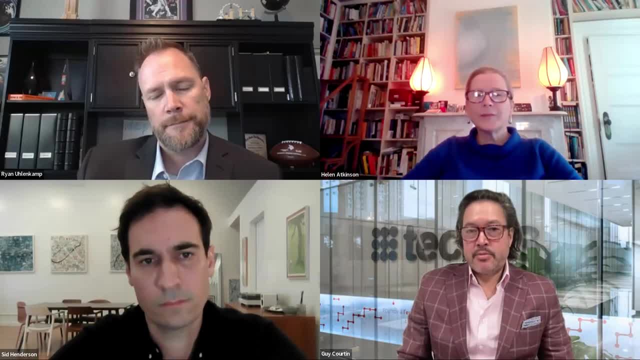 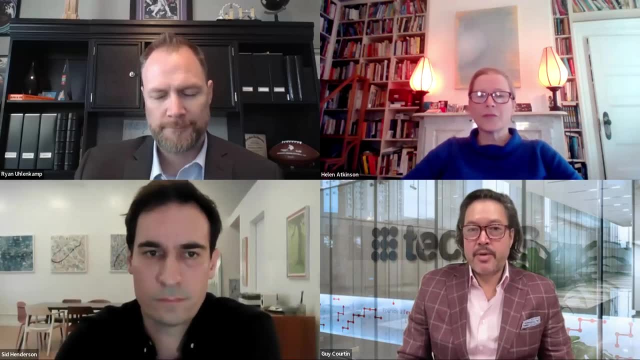 there about the data and that bird's eye view. I think what we're seeing- at least what I'm seeing too- is, you know, warehouse managers. it sounds cliche, but have to be people, right, They have to manage their people. 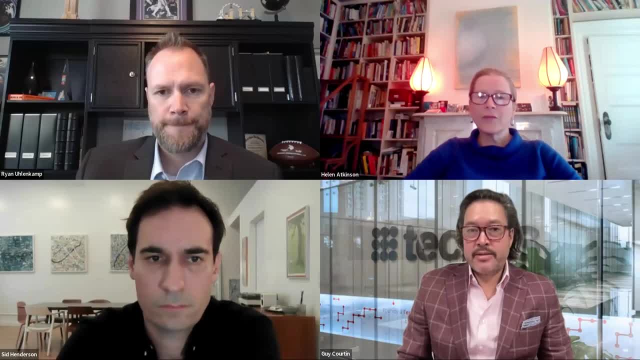 as they would want to be managed. And I think what we're seeing more and more- and back to what Sid said to begin right- the shortage of labor, but also the strain being placed on warehouses. that is not the same that it was 10,, 15,, 20,, 30 years ago, for a whole host of reasons. So now we have 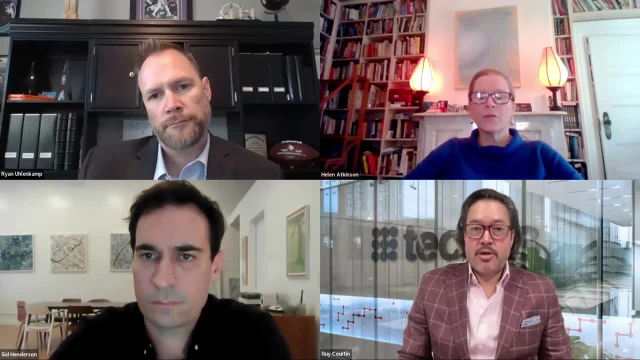 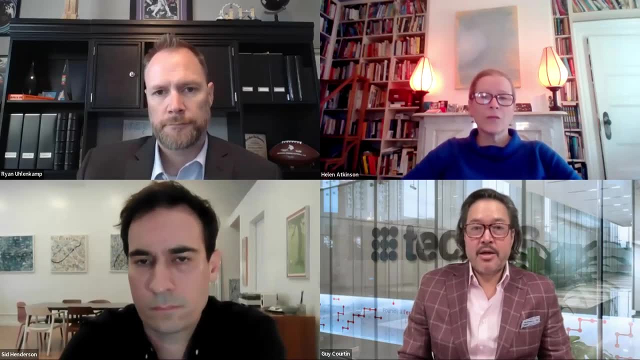 to manage as we should as a human. So, yes, use data, because data is important. but also to what Ryan said: walk the floor, be approachable, be personal, understand your people and how to manage them and how to get the most out of them. I think those are, you know those are. you know those are. 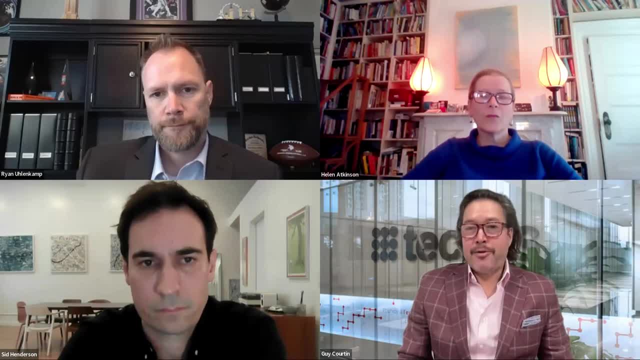 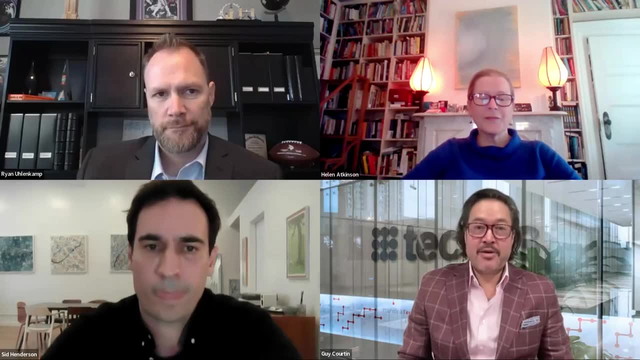 some really key trends we're seeing more and more, because you know what Ryan said: right, this is not 20 years ago, where you just you've got labor, you've got rules, you've got expectations. they don't meet it, you get rid. you get someone else, you train them up, you, you know, rinse repeat. 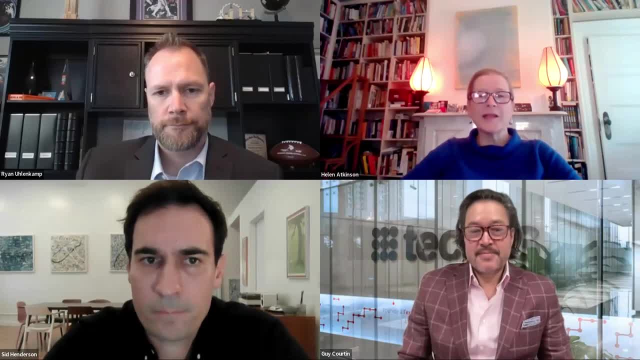 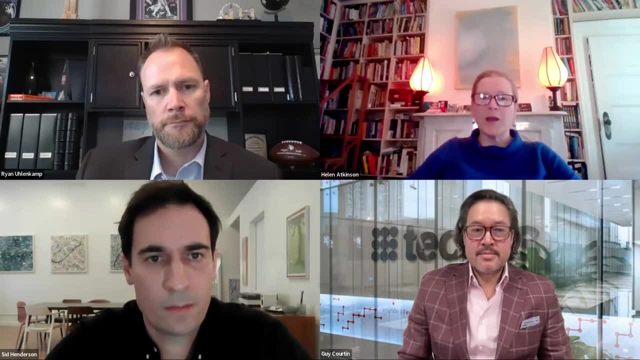 That is no longer the world we live in. Yeah, yeah, no, indeed. And just coming back to the space thing, briefly, Guy, you know that, I know that. you know when I used to go in a warehouse there'd be some vast area in the corner where all the Christmas stuff was. you know that didn't get. 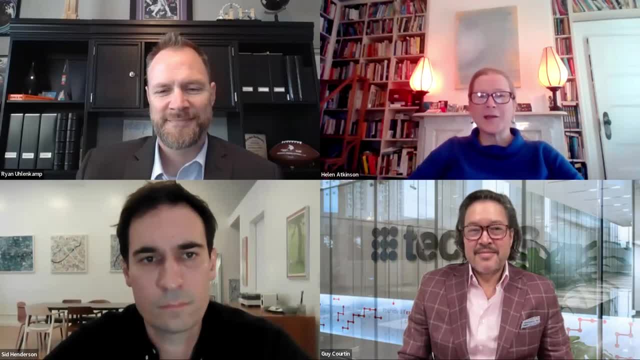 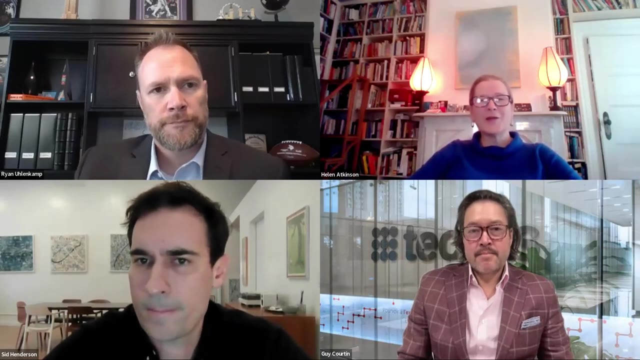 used the rest of the year And that I those days, I think, are, are gone. Guy, based on what Sid and Ryan were saying, what you said, what should be the trigger for a warehouse manager or supply chain leader to start considering automation, And who should they talk to first? 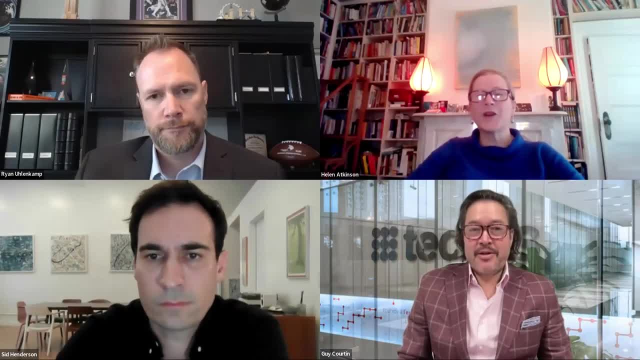 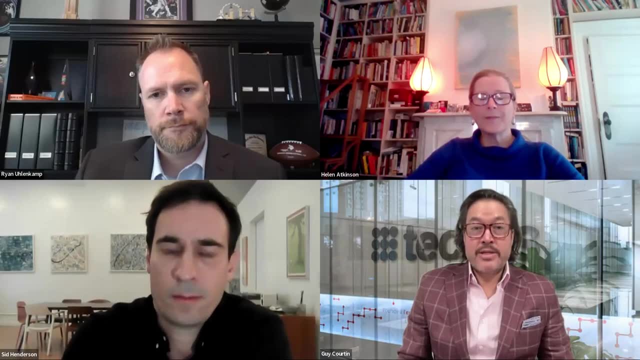 I think the trigger has has already happened, right, I think. to build on again what Sid was saying in terms of what he's seeing: the shortage of labor, that's a huge one. What Ryan was saying, the retention of labor right, Making sure that you not only get labor but you. 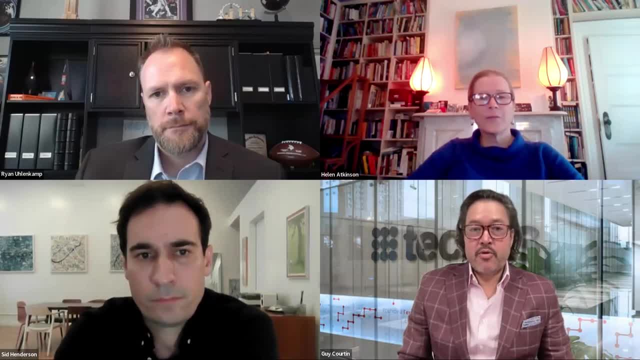 keep that labor. I think that's very important. And the third big one is, of course, the changing dynamics of the warehouse itself within the fulfillment network. There's a really interesting study by Gartner And also, I think, by Ernest and Young. it showed, you know, if you look at the top. 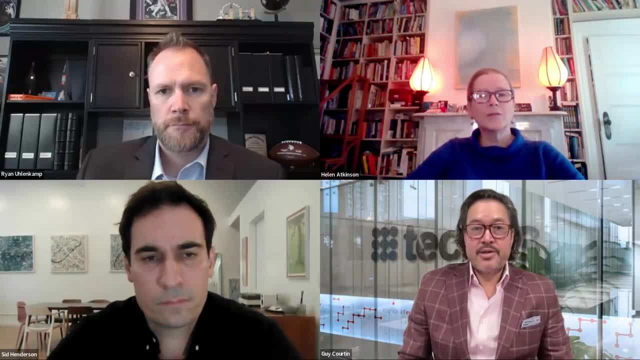 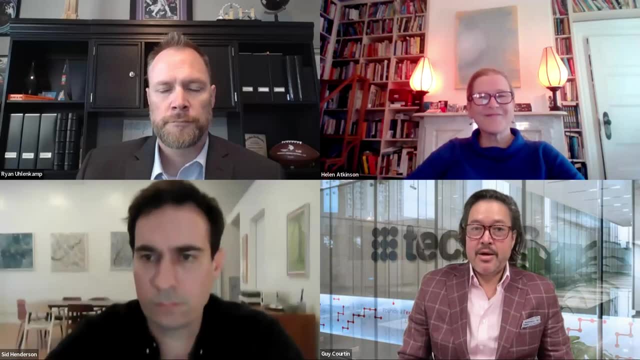 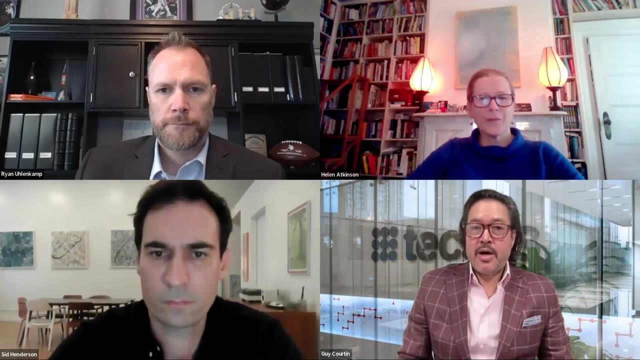 three drivers. those are, that's it. you know: labor, labor retention and new warehousing. So the trigger's there. So I think anyone who isn't already thinking about it I'm not saying run out of automation and put robots yet, but you need to be thinking about it. To your question about who 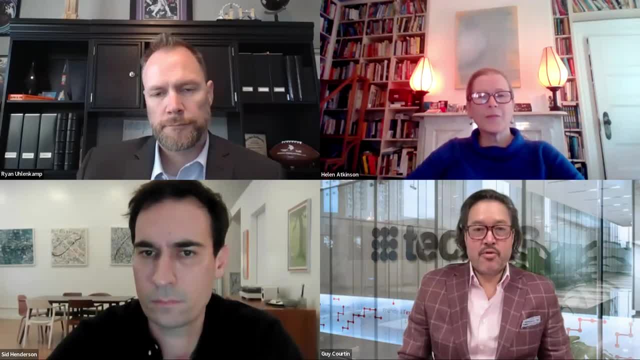 to speak to. I think that's the. that's the interesting part. I know we'll we'll dive into more of this, but I don't think it's a sort of a one size fits all where. okay, if you need robotics. 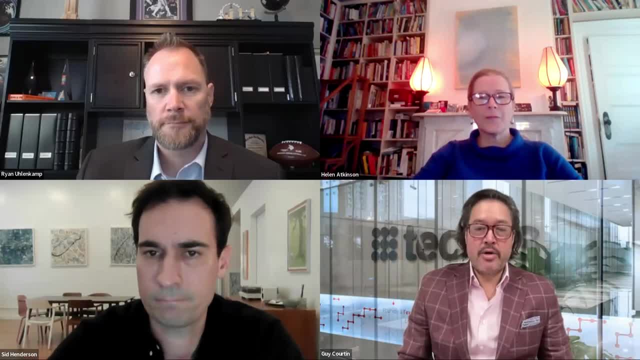 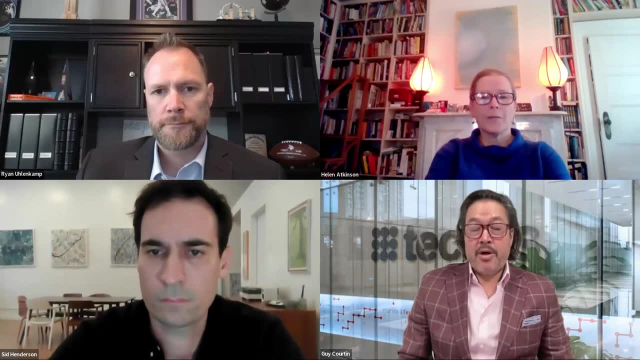 go talk to you know your chief supply chain officer or your COO and and get her to approve you know a million dollar budget to put X Y Z robot in there. I think you really have to, and I apologize, sound cliche, but start with the end in mind. you know where where's your 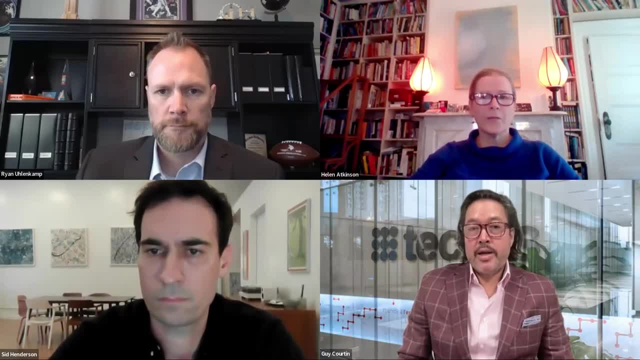 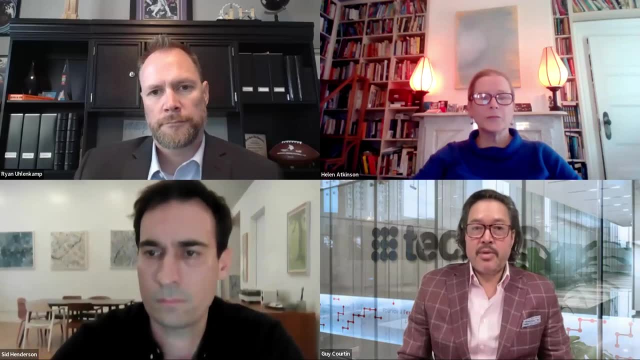 next year, two years, 10 years, 20 years? What is the type of inventory that you're moving through your warehouse? What is your labor going to look like? Is your labor going to be complimentary to the automation, or are you trying to replace some of your labor or 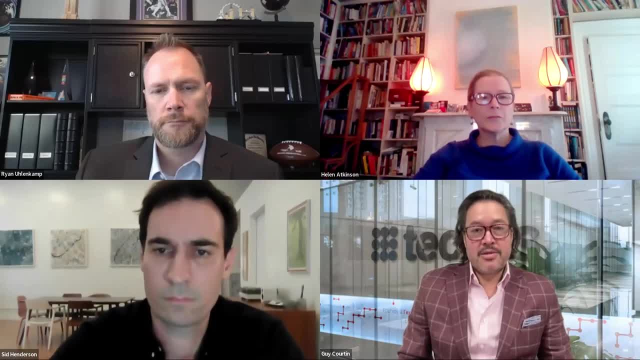 supplement some of your labor. I think those are the questions you need to start thinking about before you then start diving into. okay, well, which automation do I want to look at? Who do I want to speak to? But you, of course, have to have to absolutely get buy-in. 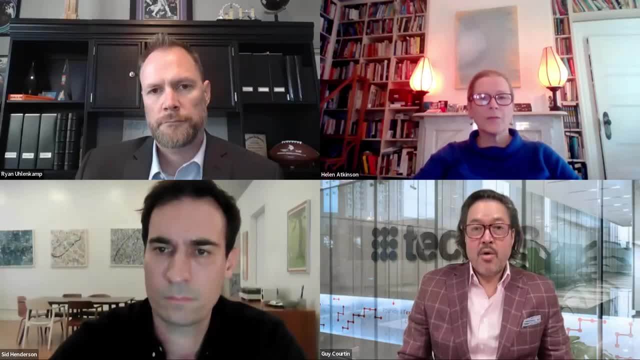 from the you know the C-suite, because at the end of the day, these are, whether it's a, you know, a smaller version of an AMR, where you're just going to rent the robot, or a larger infrastructure play. These are physical items you're putting in your warehouse that you need to understand from. 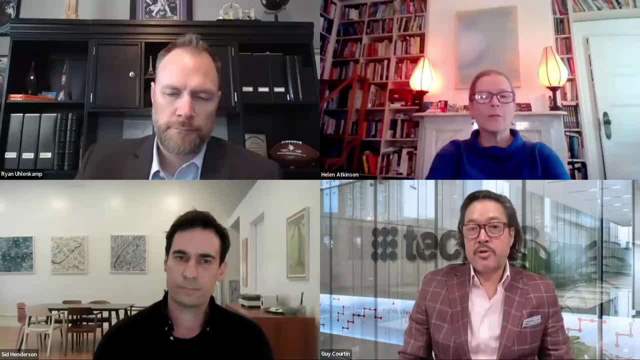 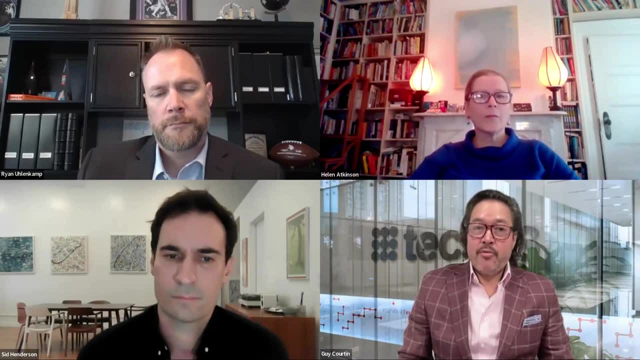 the overall strategy. How is it going to play to your long-term goals with regards to your fulfillment, your supply chain, your warehouse? But that triggering question- anyone listening to this- you know you need to start thinking about automation. I'm not saying 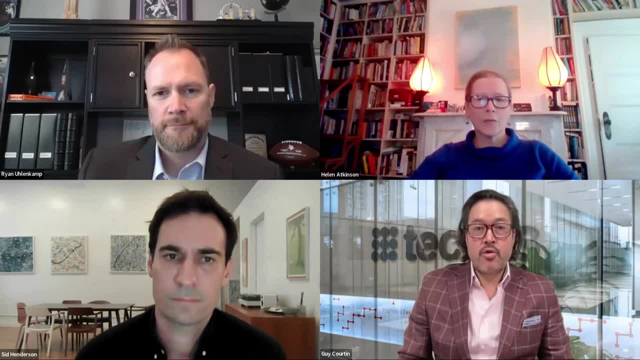 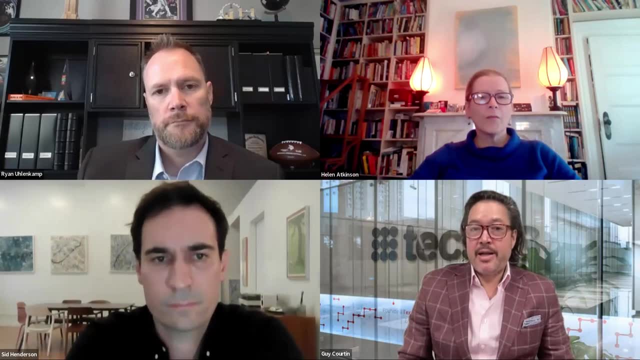 rent out and buy automation, but you need to understand where does it fit in your long-term strategy and when do you need to start looking at bringing some in. or maybe you don't, but you need to be aware of it and understand what decisions you will make around that, Right, Yeah? So basically, 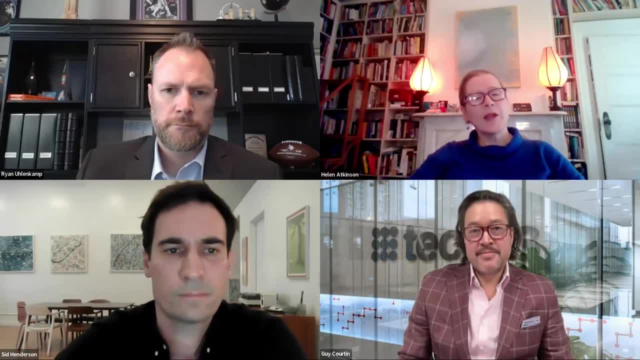 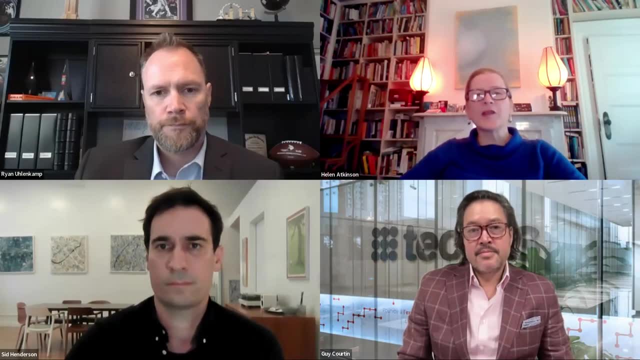 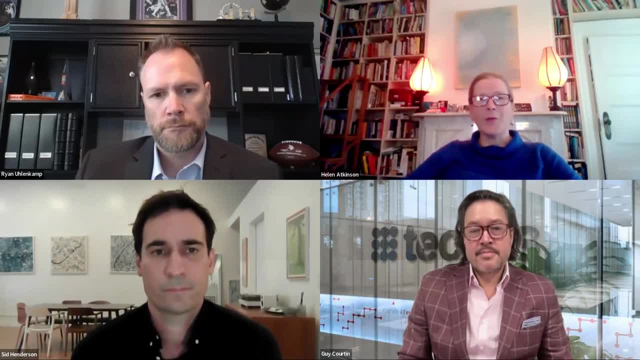 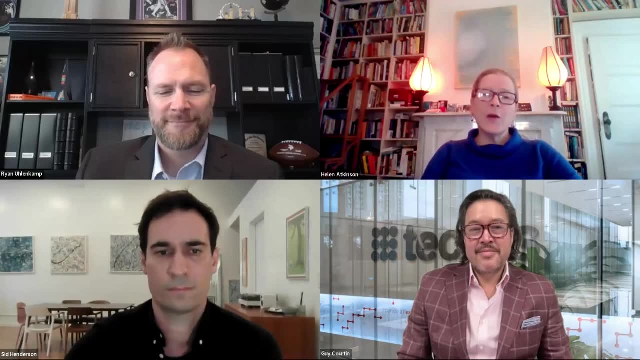 to think of these bigger picture things that you know, frankly, are going to be a pain to implement or, at least you know, daunting in some way or other. Do you have a sort of typical story that somebody comes to you with goes: well, you know, we were trying to. 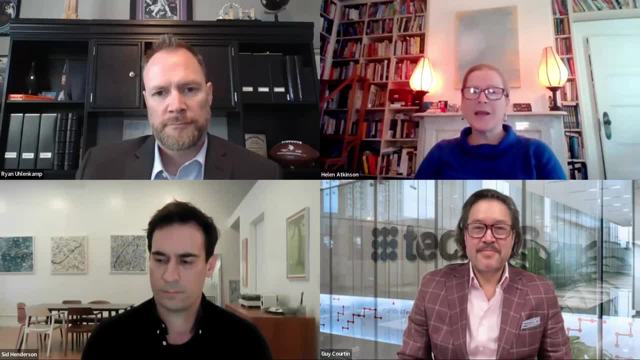 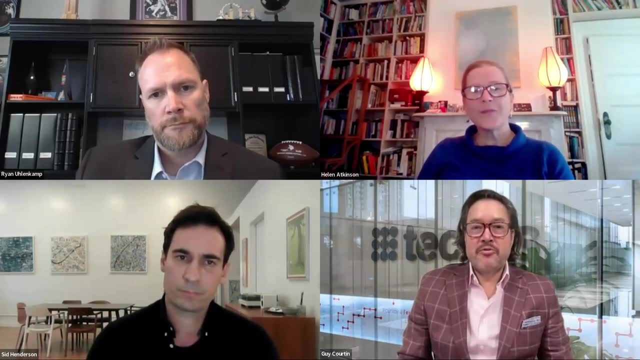 get Black Friday sorted and it all was a disaster. Is that? is that typically? is there a crisis? often that sort of prompts this Absolutely. There's obviously always usually sort of a burning platform, right. So I think there's a couple to think of. One is, you know, traditional sort of e-commerce world. Oh, you know. 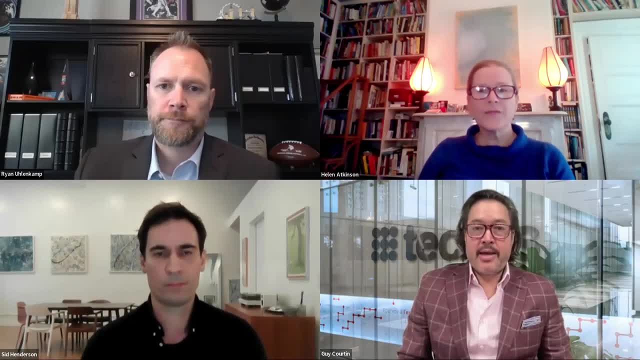 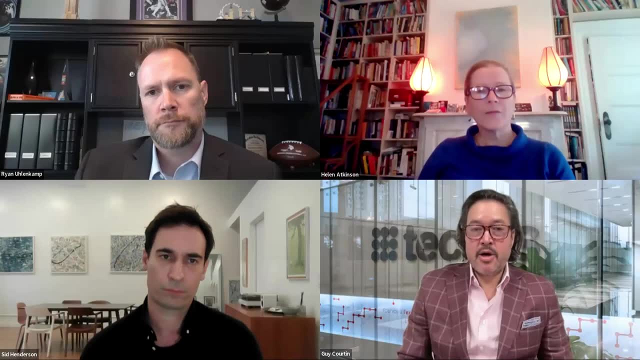 my, my e-commerce sales are going through the roof. I can't pick in my warehouse fast enough to meet those orders. What do I do? Okay, You know robotics, AMR solutions might be the right place to go. Or, for example, you know, my warehouse is being asked now to hold. you know. 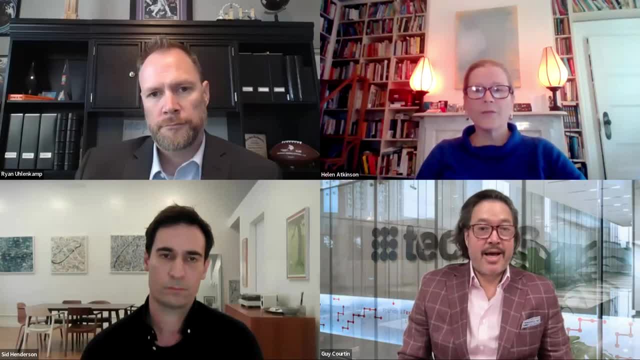 2X the amount of inventory I used to and I need to find a place to store it and get access to All right. Well, maybe there's something where you want to look at, you know, sort of an ASRS type system. 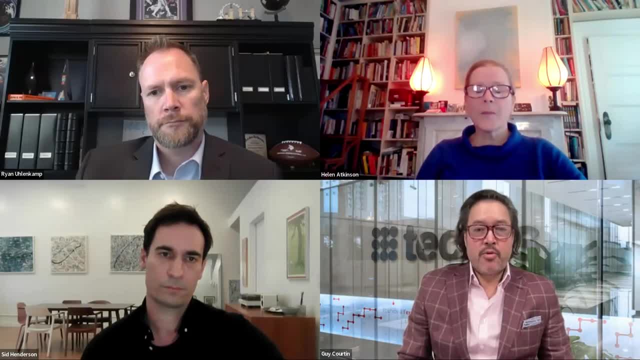 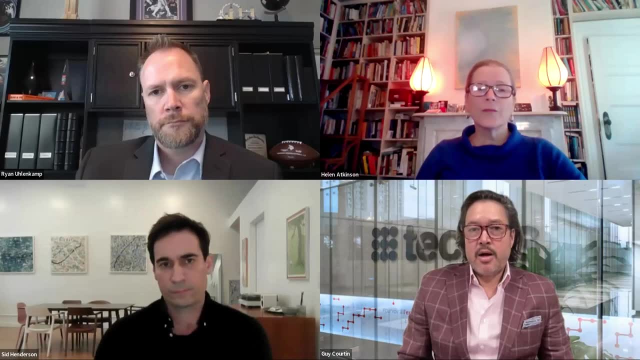 Where you can store, have more high density of storage, right. That's a trigger point. I even seen down to the point of you know people, we talk about labor. Some have come and said, oh, you know, I have 1.5 FTE. All they do is they move dunnage every day And all of a sudden, 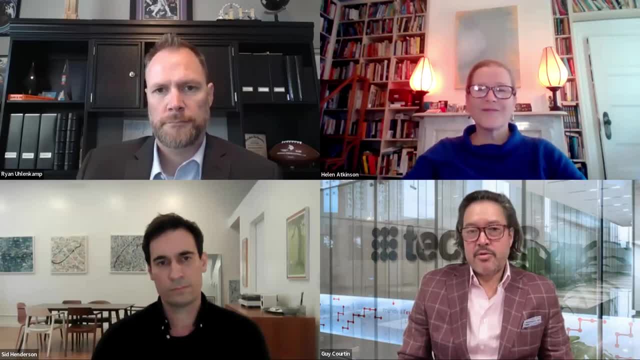 they realize: well, you know what. I can go out and actually get a robot that will do it for me. By the way, it doesn't take smoking breaks, It doesn't, you know, show up late to work. It will just do its job. So maybe that's a. 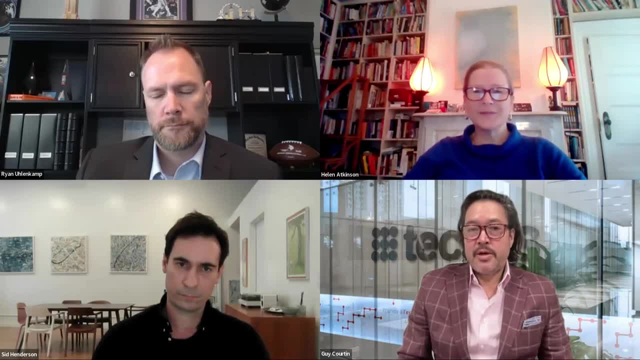 a smaller use case, But all of a sudden, it gives you an opportunity to focus in on specific use cases where- again to your point, Helen- there's a trigger event. Oh, I don't have enough labor to do this, Oh. 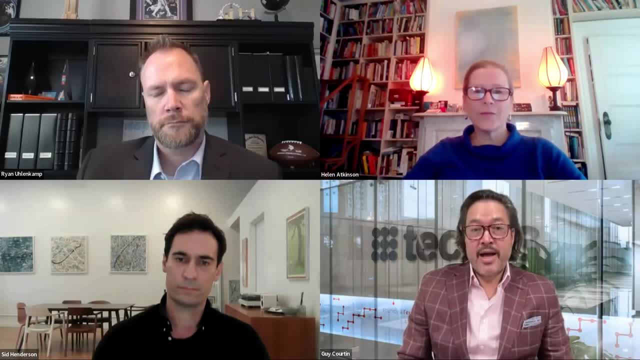 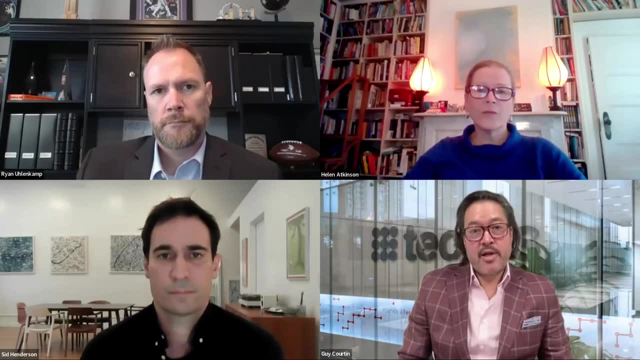 I need more storage. Oh, I need more velocity of moving items out of my warehouse. Oh, I need more precision of picks. right, I need to have my orders get to the five nines of reliability to pick. Maybe the robot's going to help me do that. So I think those are some of 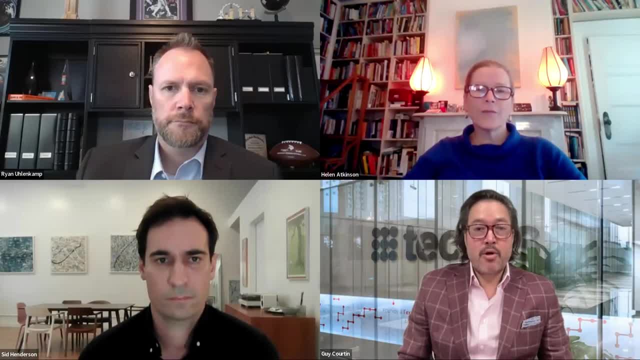 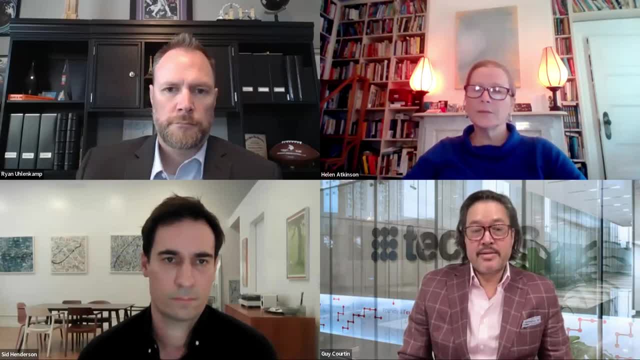 help me do that. I think that's going to help me do that. I think that's going to help me do that. So I do think yes, And, and you know, each warehouse is going to be unique, They're going. 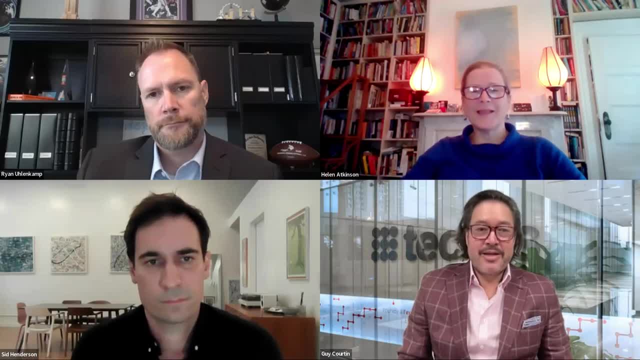 to be a thousand burning platforms. Let's face it right. You said we're always firefighting And it doesn't mean that it's going to be a robotic solution for each one of those, but it's really the discipline to look at those and then to identify which ones could be addressed. 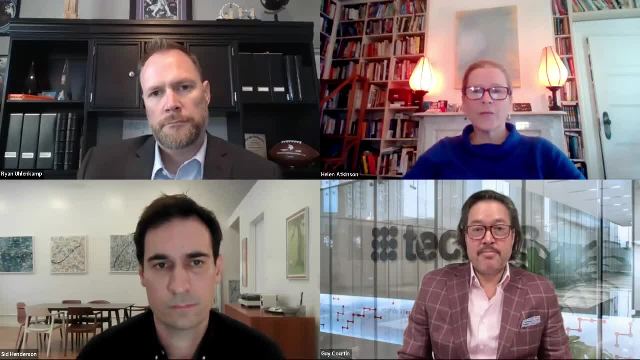 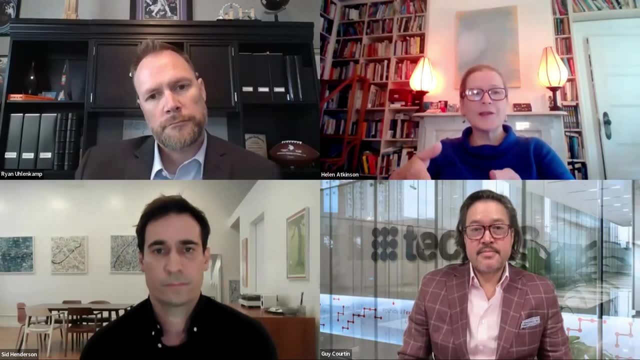 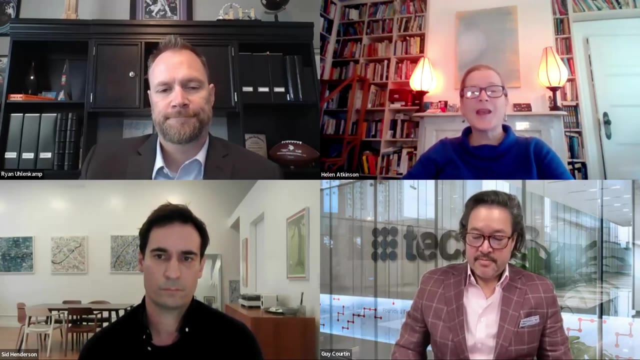 by automation and then to find the right solution to solve that problem. Right, Thank you, Guy. And so let's dig into that a little bit. you know, because there are all these different automation hardware types in the marketplace, from conveyors, pit bulls, AMRs, sky pods. 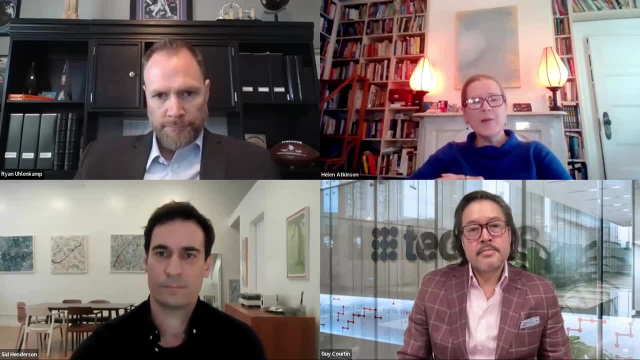 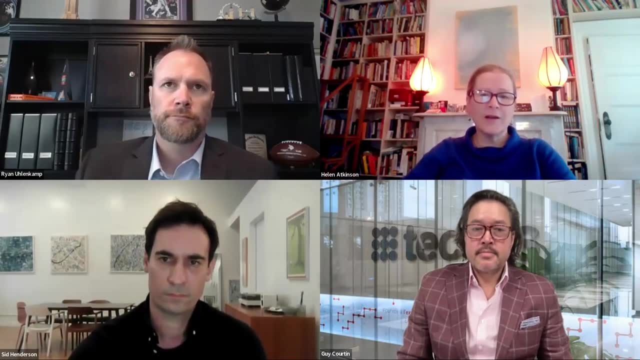 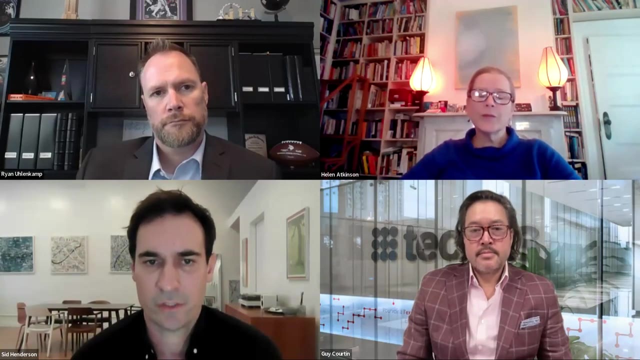 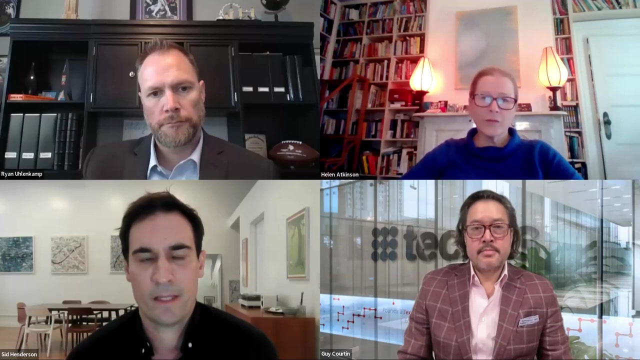 any combination of those Sid. can you tell me what drives the selection and implementation of a particular type or combination of automation hardware? Yeah, Helen, I think that the two main factors that typically drive the solution selection are performance and flexibility, If your warehouse requires a very high throughput. 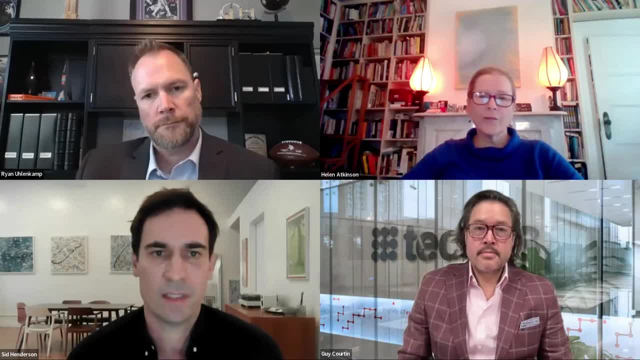 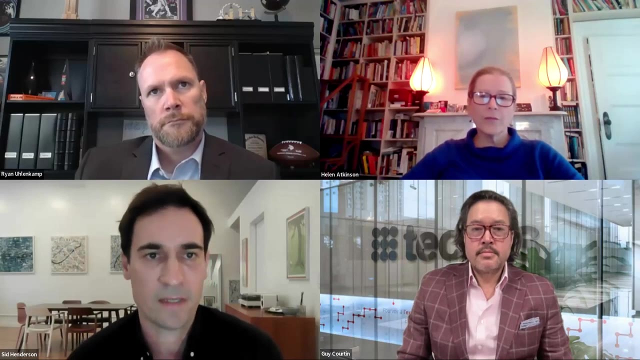 then a traditional source of automation like a shuttle system is probably going to be what you're going to lean towards. It's going to be a higher capex, It's a higher. you're going with a solution that you're going to have for maybe the next 10. 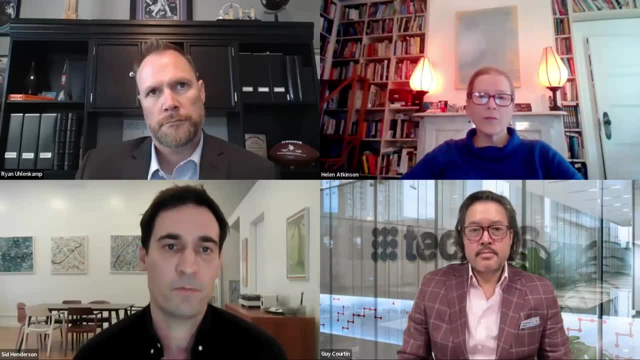 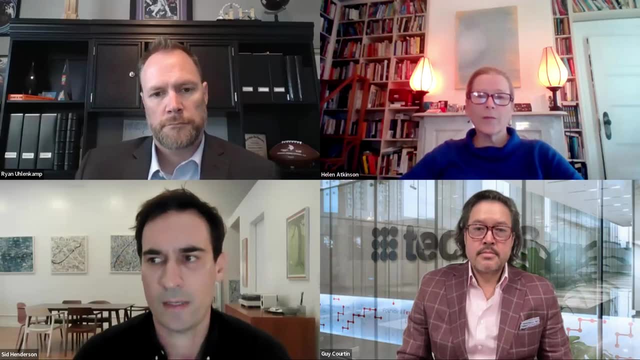 years, but you're optimizing for performance. On the other hand, if you're maybe a company and your operations that's growing quickly, or you have high forecasted growth, maybe you're not ready to make a large capex investment right now. 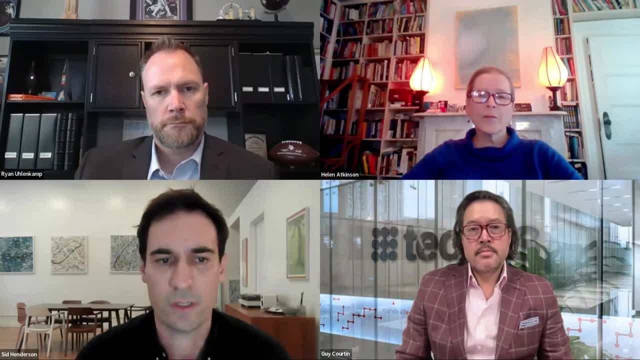 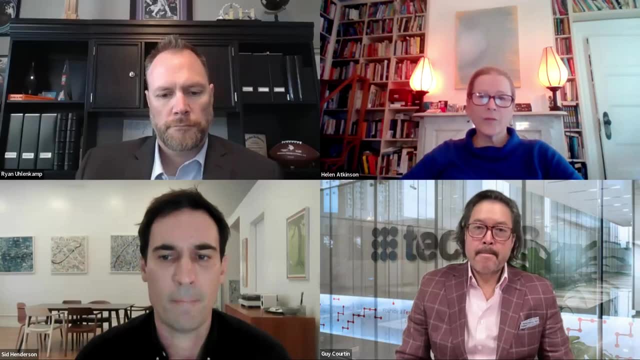 Maybe you have some uncertainty about what your future is going to look like in terms of your omni-channel distribution or just your needs in general. You're going to want to boost in your productivity and your performance, but maybe you don't want to take the risk of a more rigid shuttle system. 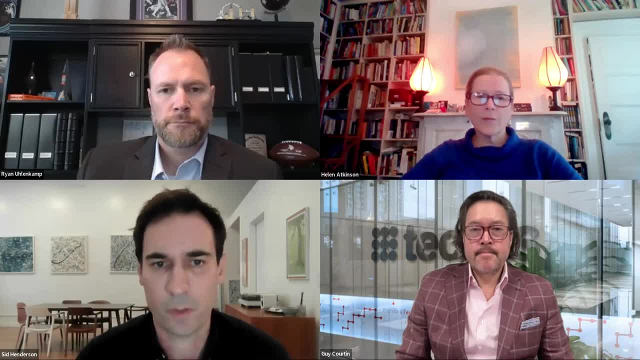 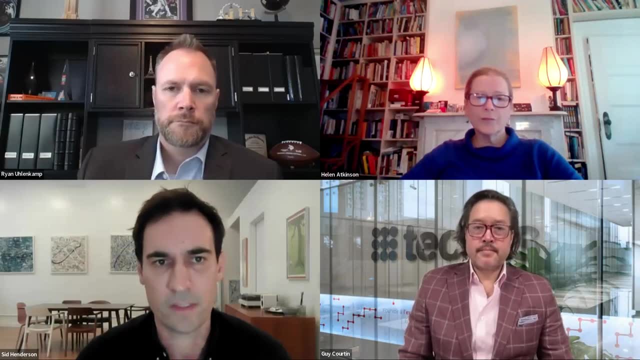 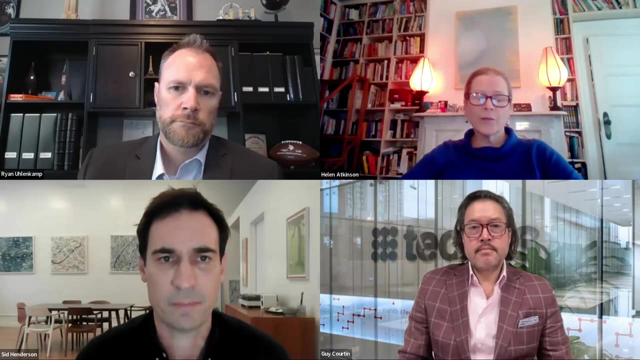 You want an AMR solution, Thomas mobile robot on their OPEX options. There's a lot of flexibility there. Yes, it comes with some limited performance, but that might be a great solution for you And for a lot of the companies that are experiencing high growth. but maybe 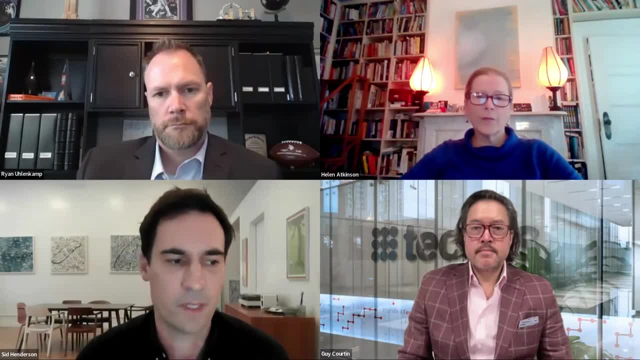 they're not at $2 billion a year annual revenue. that's going to be a great solution, But what we're also seeing now are a new generation of solutions, similar to Exotech, that are trying to optimize for the balance between high throughput and 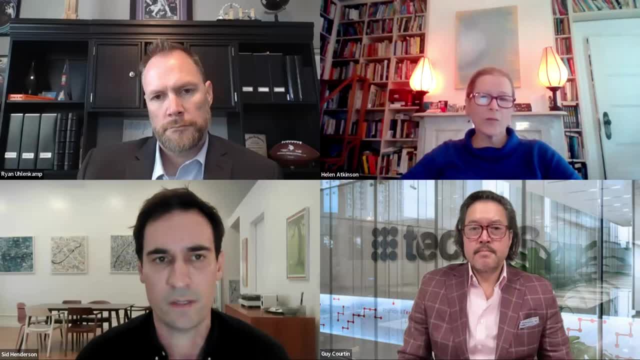 flexibility so that you get a system that is the right fit for your current operations, but we'll also have the flexibility to adjust as your company changes over the next decade. So, Sid, are we talking about robots that can perform different types of tasks, or just ones that can be moved to different parts of the warehouse? 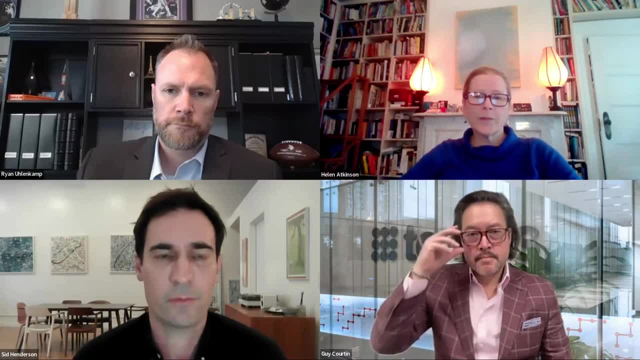 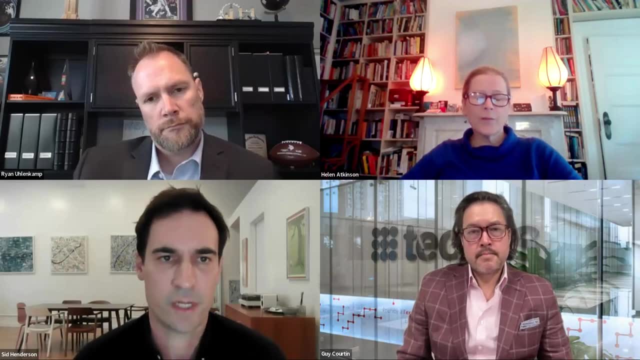 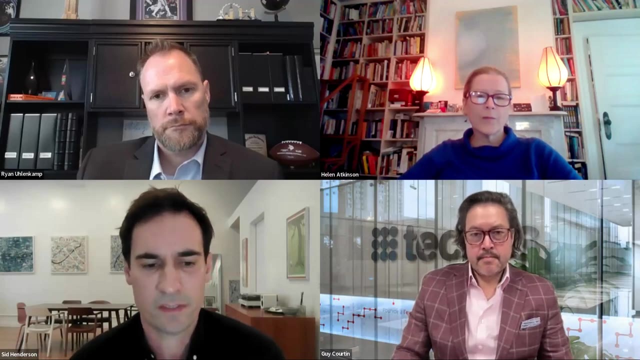 I think it's more. is your throughput or your throughput requirements going to be changing or um? are your, are your storage requirements changing? Um? all right, Do you need um? because the way this this can work is if you. 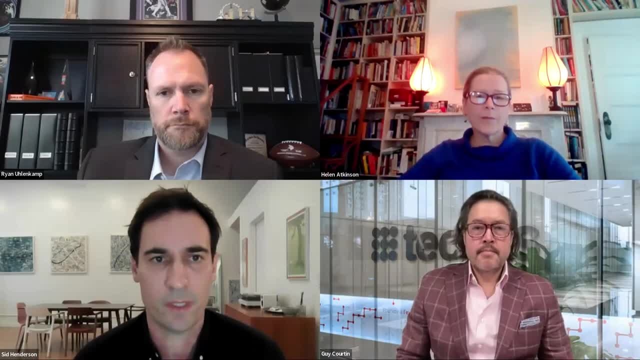 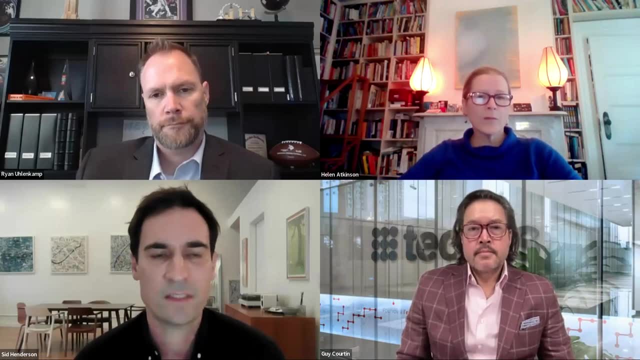 um, if you have a system where you can just add more robots to get more throughput, or you can add more racks to get more density and more storage without disrupting the operations, then that's a really flexible system that that can change and adapt with you over time. 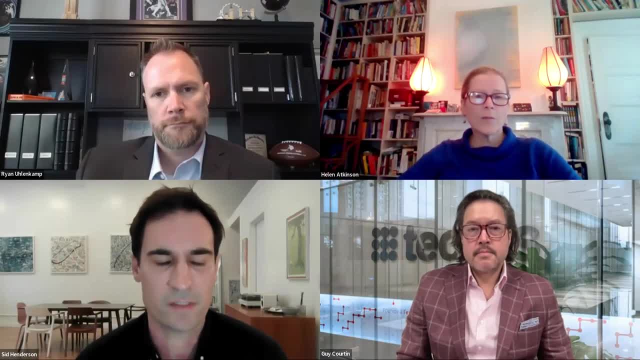 And in customers. a lot of customers are going to get a lot of value from that, because it really allows them to to optimize as time goes for their operations, Right, Yes, And of course, it's not just about robots, It's about racking and all sorts of other automation hardware. 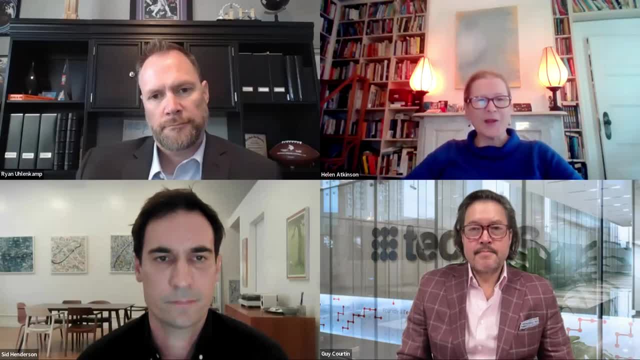 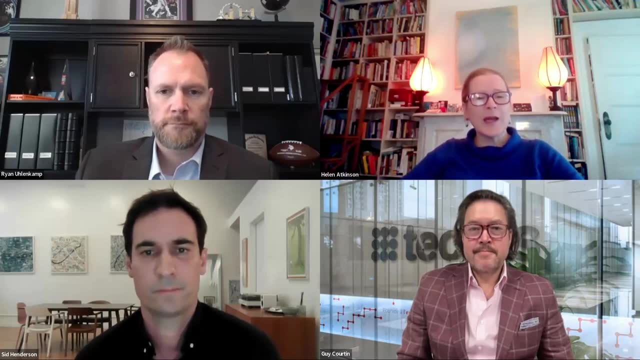 Thank you, Um, but automation is just one piece of the puzzle and human labor is still a much larger piece. Um, Ryan, how would you describe the relationship between labor management and the selection and deployment? Um, how would you describe the relationship between labor management and the selection and deployment of automation? 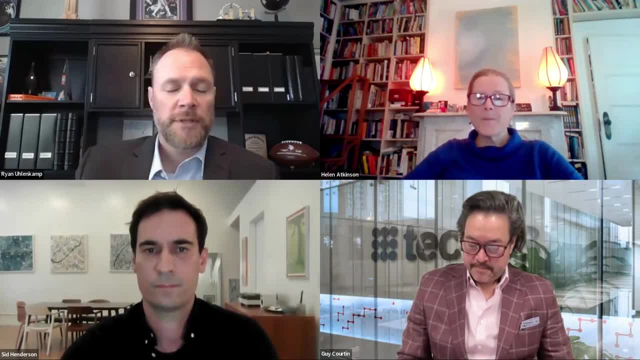 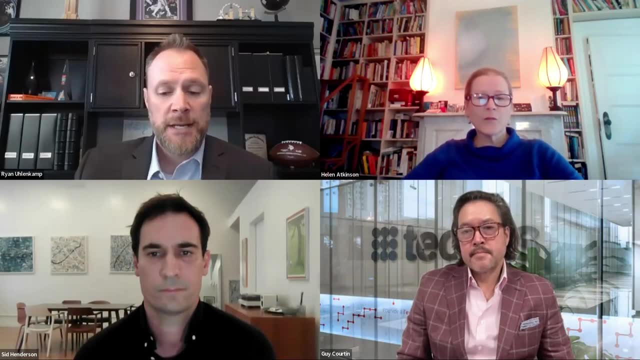 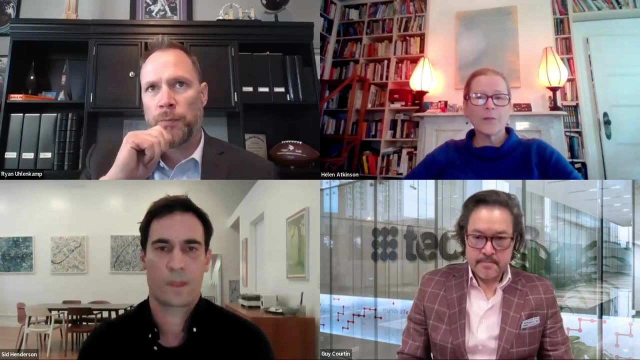 How do they work together? Yeah, I would Well, they're definitely complimentary. I actually would go as far as to say it's a symbiotic relationship. There's mutual benefit, um between automation, the human workforce. Um. automation has the ability to replace and take over some of the most physically challenging and monotonous tasks. 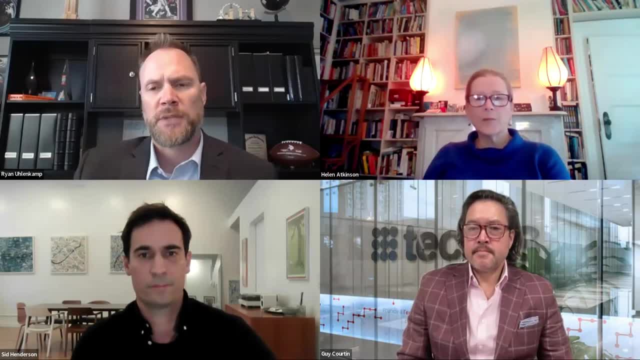 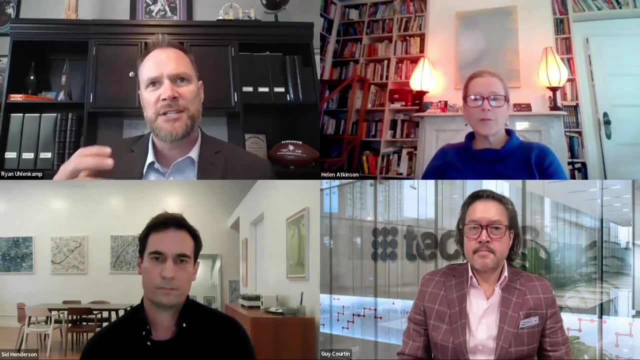 which are very hard roles to fill with humans. Um, so I think the right automation solution like Sid talked about- and I think a lot should go into identifying the right automation- but that can change the user experience in the warehouse right. 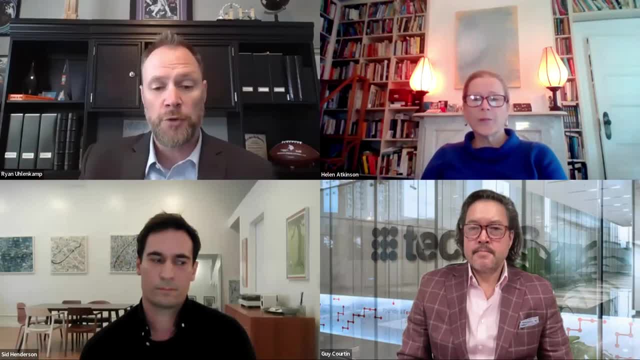 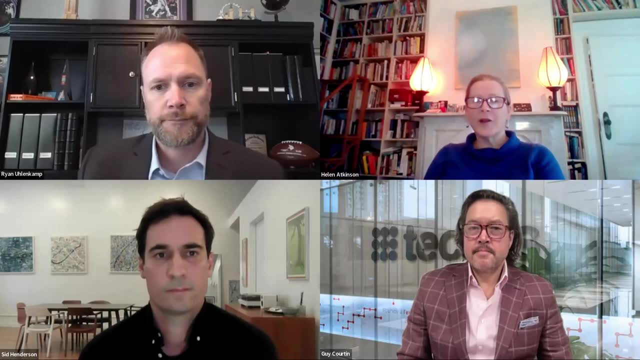 That completely redefines what work looks like for a human. Um, I was like he was saying: you know you're spending hours a day dealing with dunnage. You know who wants to do that. You can get a robot to do it. 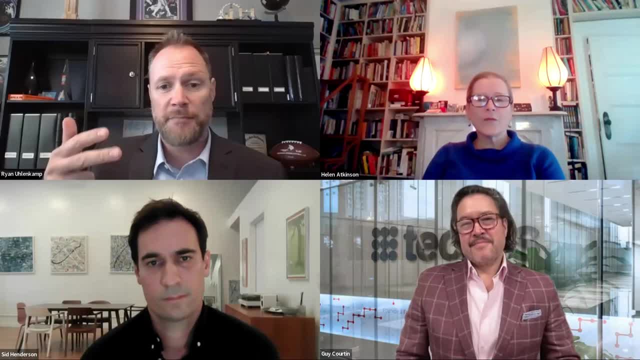 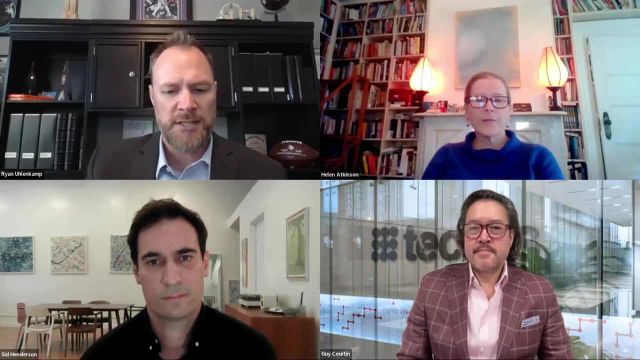 Yeah, heavy lifts, lot of bending, miles and miles and miles of walking like those are the things we start to eliminate. Um with an automation solution- And I don't think automation is- is about replacing jobs. It's about reducing those impacts. 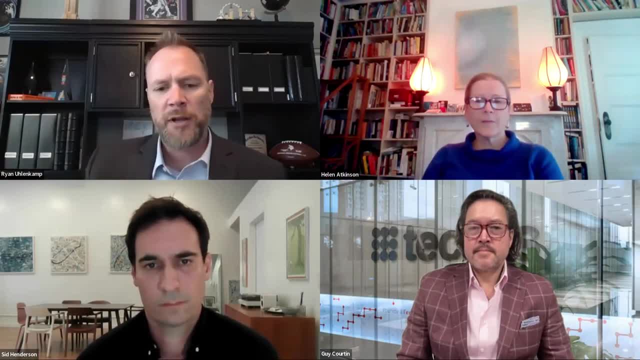 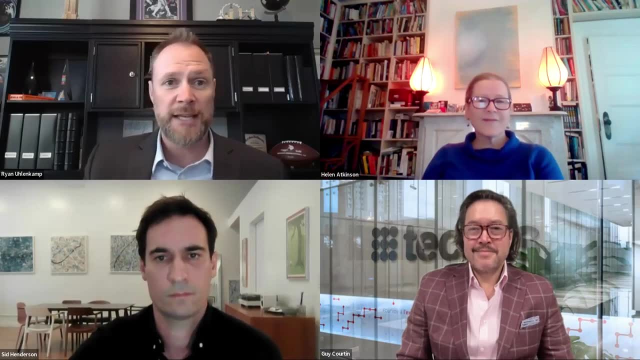 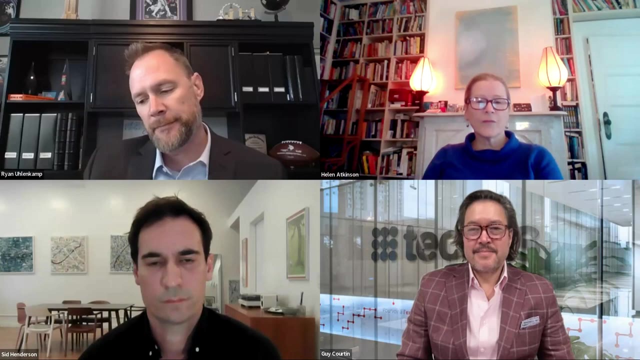 right Those burdened pieces of the work as well. as we've all seen how warehouses solved peak problems is mandatory overtime, long hours grind. like eight weeks of mandatory overtime Like these are grind. So I think that's the relief valve, along with resiliency and a ton of other. 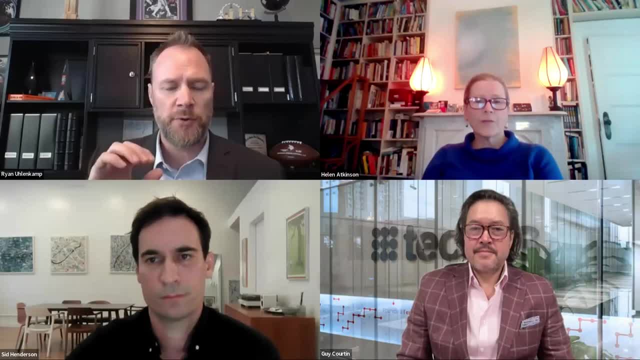 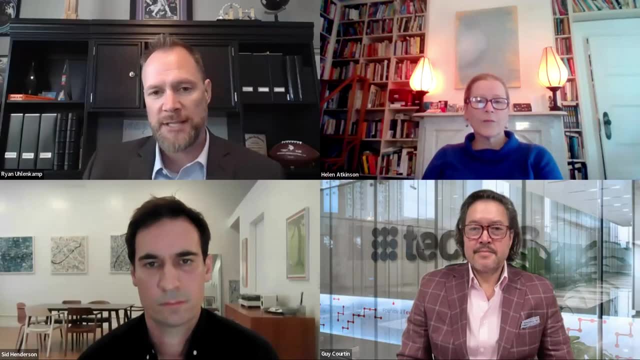 Uh, benefits there And I think it also allows the human workforce to focus on more meaningful and value added task and creative tasks than than the monotonous ones we talked about. I, I would stress, and I think he and said of both hit that earlier. 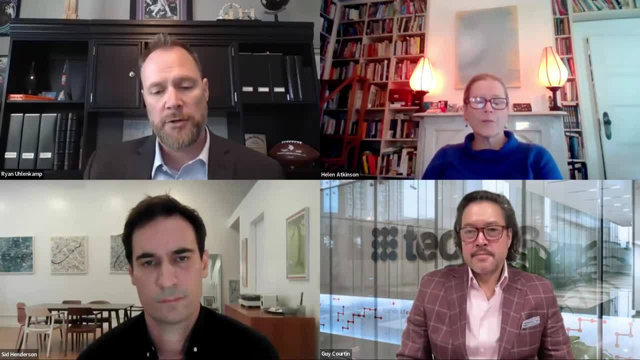 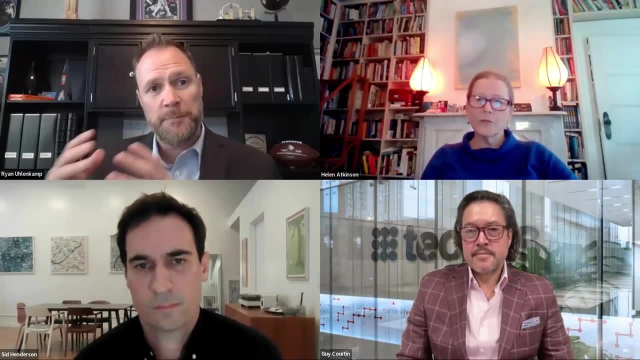 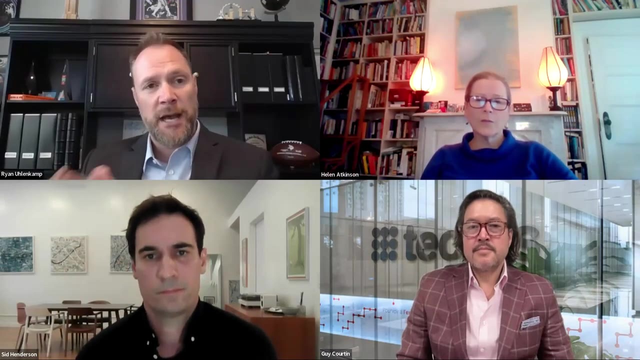 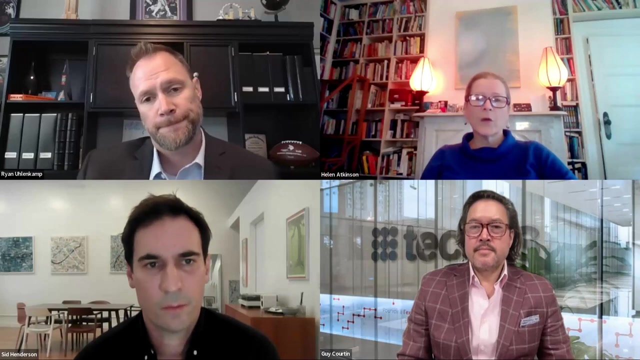 the to bring all of that together. you really need to make sure you pick the right solution, and I would. I would urge everybody to really think about the change management piece that goes into that. How am I communicating um the impact- The positive impact that an automation solution has, while I also look at the unlock and how I'm going to engage with my people? 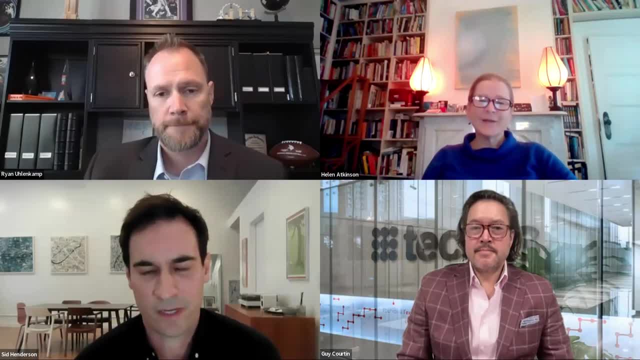 Right, Sure, Just to add on to Ryan's point. I mean, I, I, I so much agree with everything you're saying, and especially in the context of this new law in California, where fast food workers are going to be making $20 an hour. 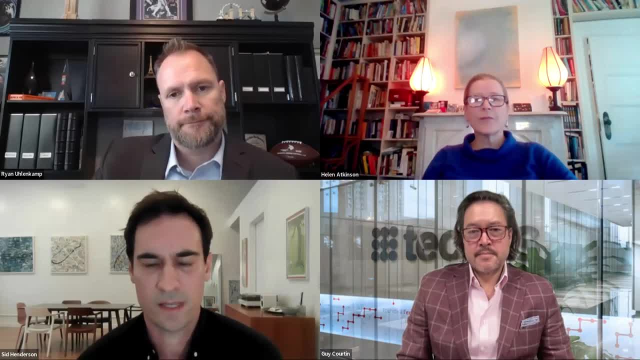 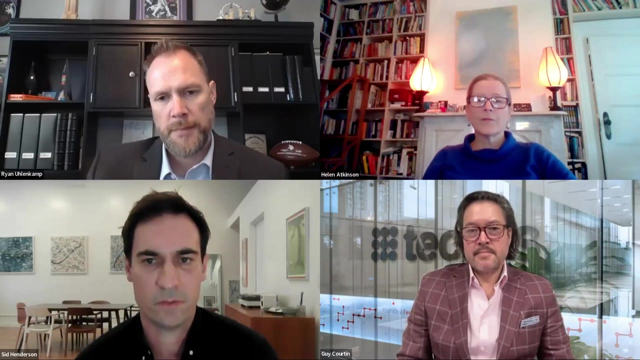 I think something that's going to come more and more into focus is: are we optimizing for Our labor forces happiness, that the workers happiness inside the warehouse? How can we do that? How can we have them prefer to work in the warehouse and not work in fast food? 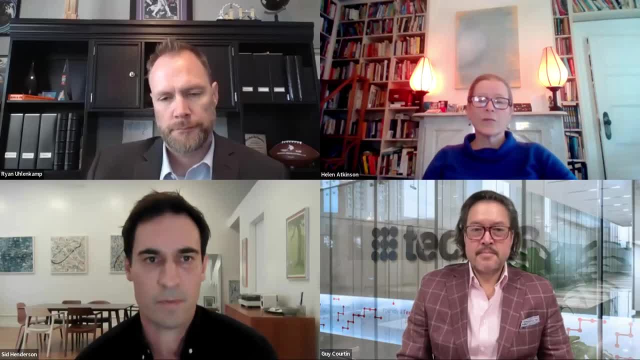 And automation is a great way of making those workers happier and making their days easier, And I think that's a really important thing for us to be thinking about now. Right, I've read several accounts of of uh, where has managers running events to sort of meet the robots? 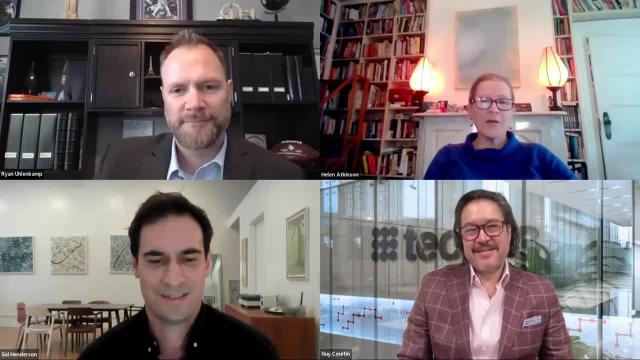 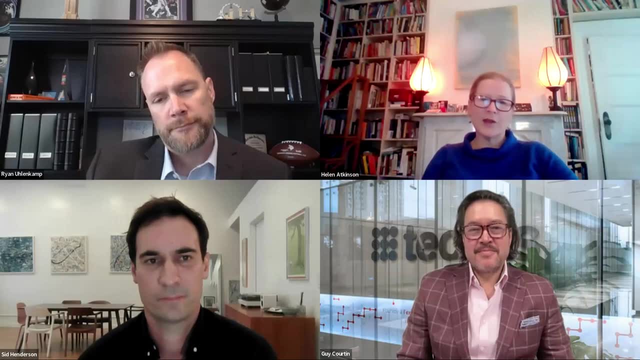 and even having robot naming competitions in the staff, which obviously really increases the sense of welcoming, and that the two elements are going to work together. Guy, do you have any particular insights in how to make sure that robots make people happier or automation makes people happier? 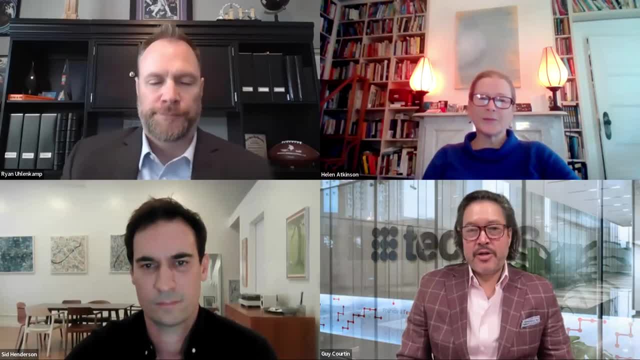 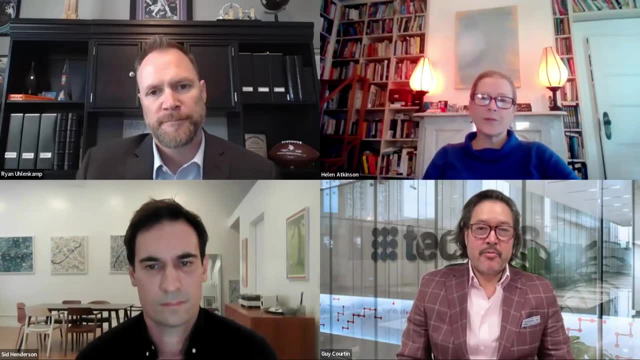 No, I agree. I think, Sid, you made a fantastic point sort of measuring labor's happiness in this equation. But yeah hell, I did see one robot the other day, a drone transporting beer around, So maybe that's one way to make people happy with robots. 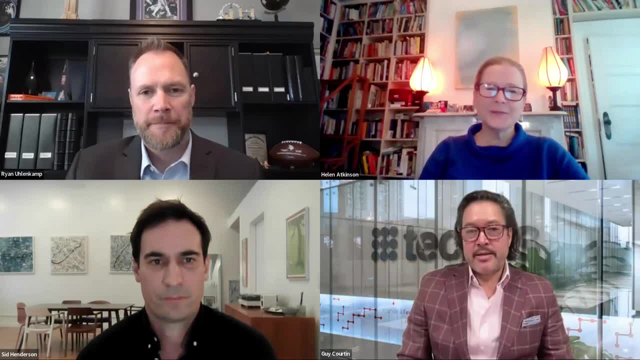 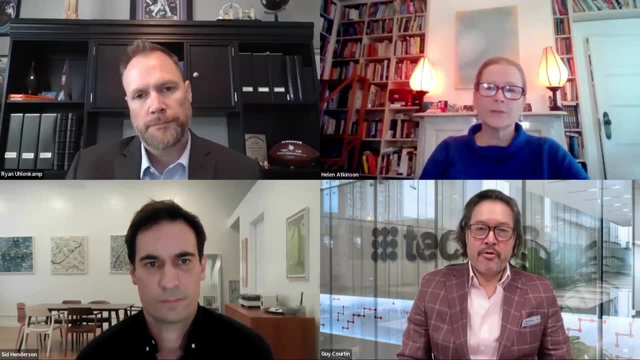 But I think part of it is- you're absolutely right- is both to what Ryan was saying and, I think, what Sid was saying about this happiness level. And I don't want to sound all rainbows and unicorns, but the reality is the robots. yes, they're there to do a job. 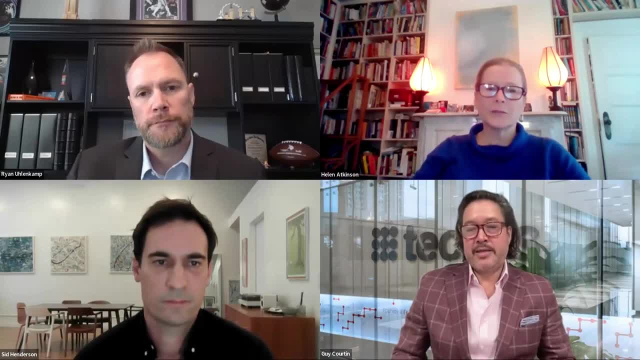 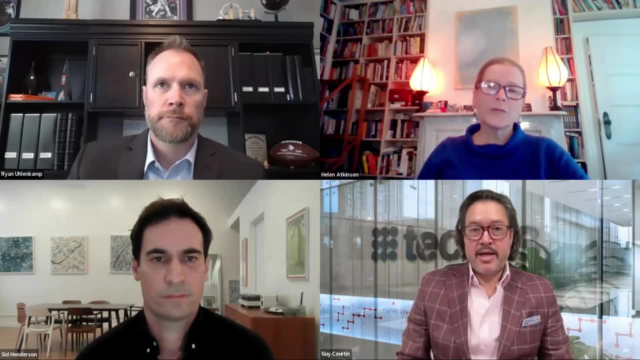 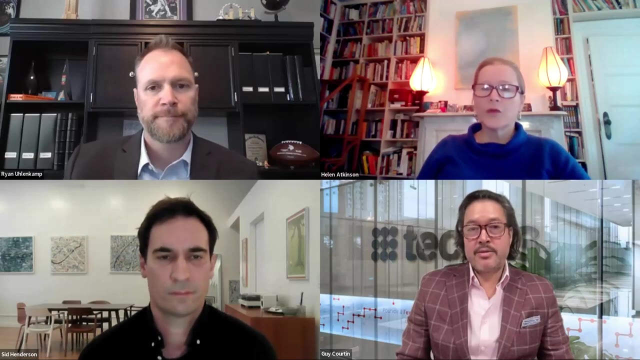 but they also add value to the experience. One of the last things I wanted to say is one of the lessons I saw. So, before coming to Texas, I've worked at Six Rivers during the pandemic And A during the pandemic, we saw robotics, or robots being able to keep labor distant. 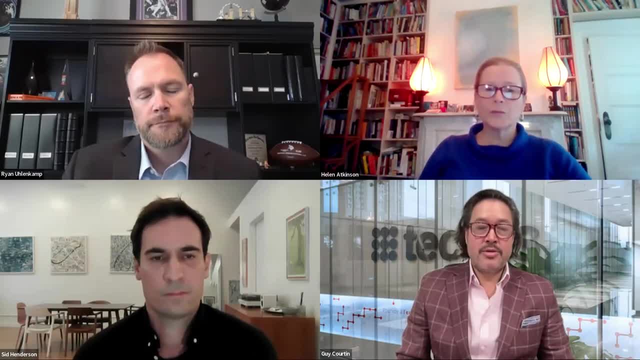 So there was that added value in terms of using the robot. But secondarily- and I'm going to bring this up and I know I'm going to roll my eyes when I say this- but the millennials when we look at this new workforce. 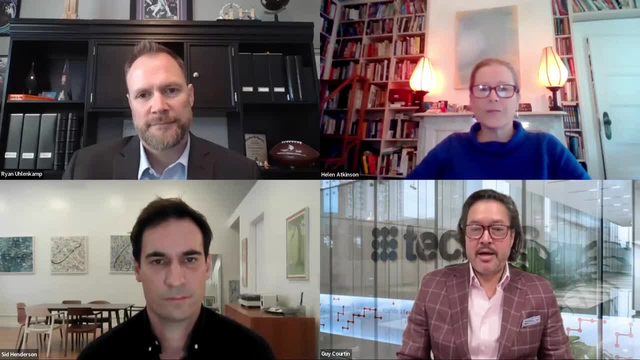 I think, Sid, you mentioned the workforce is aging, but we're also getting a new workforce coming in that guess what They're used to being on touchscreens and iPhones and iPads and Samsung devices, So to be able to go into a warehouse. 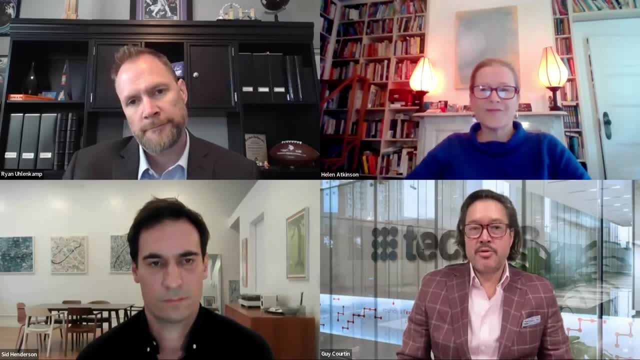 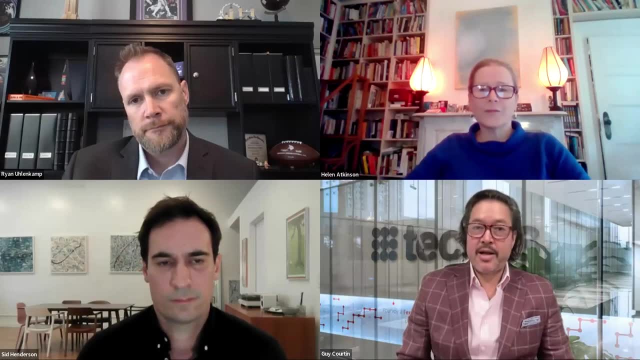 and work with a robot that mimics what they're used to and what they enjoy interfacing with, as opposed to working at a fast food restaurant or working at a warehouse, that you're still pushing that cart up and down the aisle and you're picking off a paper. 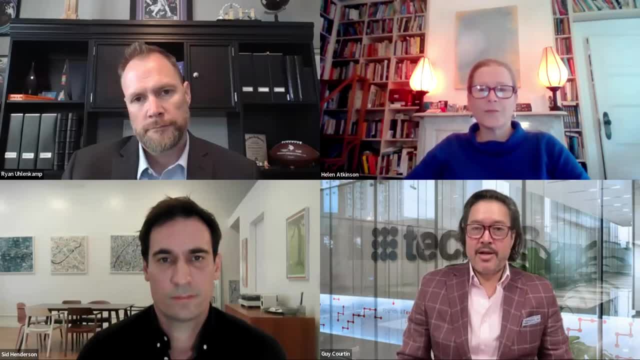 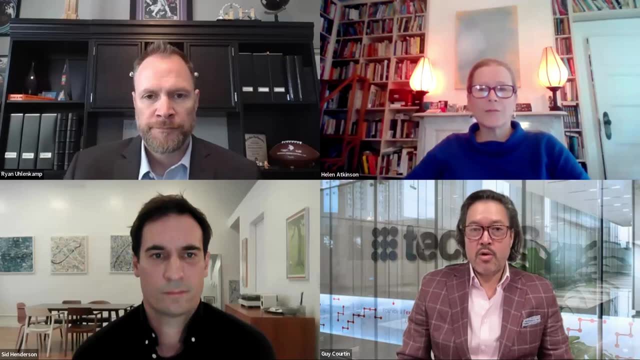 you tell me if I'm a 22-year-old coming out and I'm looking for a job and I've got two opportunities- or paying out the same amount of money, but I'm working in one warehouse where I work with this robot. that's cool. 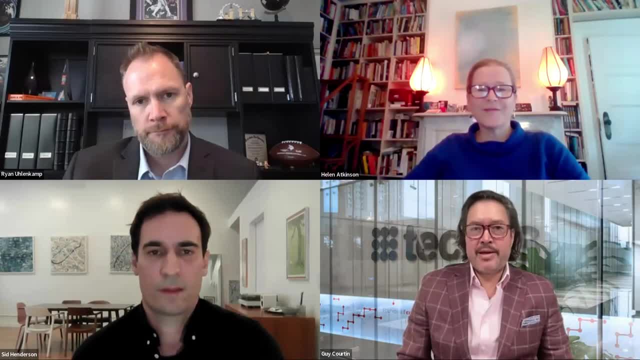 that has a touchscreen. I pick it up within five minutes. Why? Because I'm just used to that. Or it goes to other warehouse and they're like: oh yeah, you see that cart. Well, guess what? You're going to be pushing that all day. 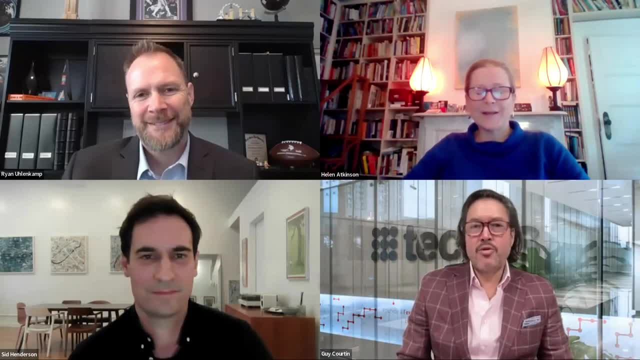 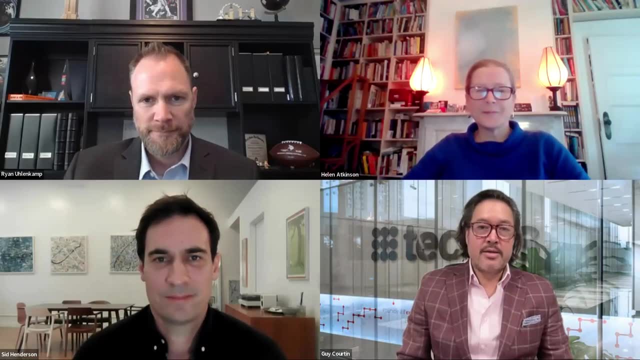 And by the time you're done picking each time, it's going to be about 200 pounds. So if you want to work out, yeah, go to that warehouse, But it gets old after a while. So I do think we're absolutely seeing. 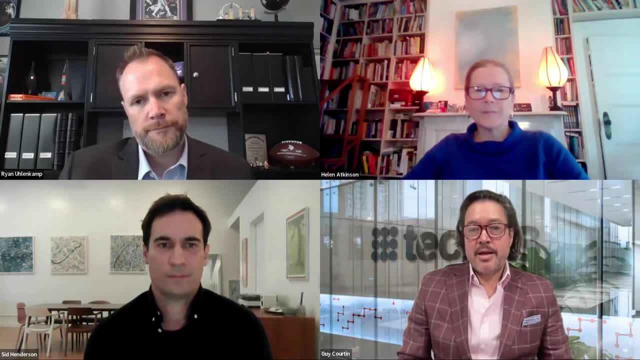 where a value out of the robotics coming in to complement the labor is to hit all the things we just talked about, And I think this sort of happiness of work quotient will certainly see robotics being a bigger part of that equation than, honestly, we thought was going to happen. 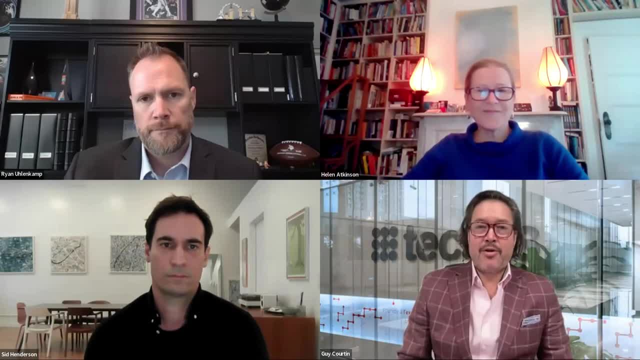 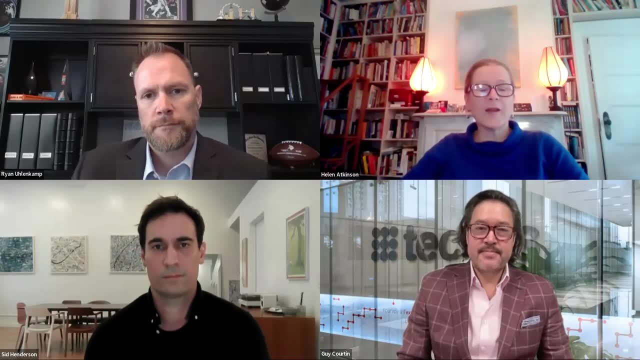 Like I said when I worked at Six River, we never thought that having a robot working with a robot because it was cool would be a big driver, but it turns out that it is Right. Yeah, That I think the cool tech factor is yeah. 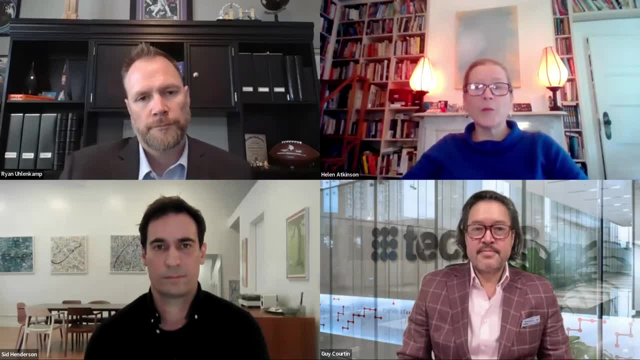 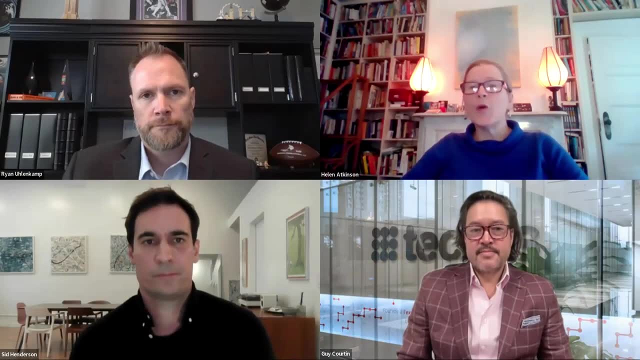 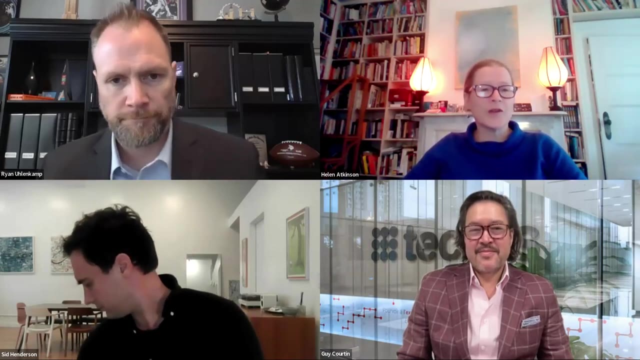 It's very important- and it speaks to an overall problem with the supply chain industry- that it's not super attractive or hasn't been super attractive. It's very old fashioned in most people's minds And I think this is really helping improve the overall impression of what it's like to work. 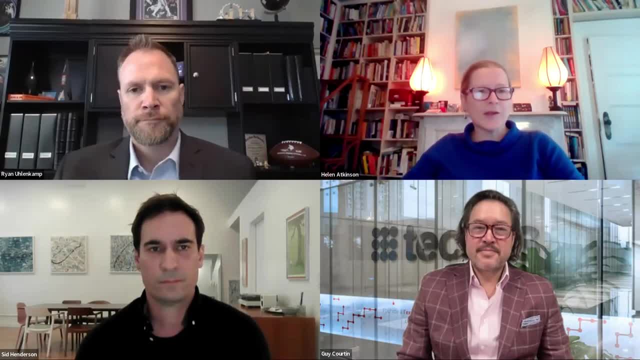 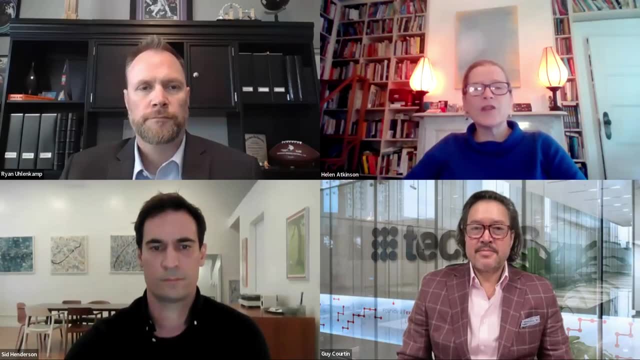 in supply chain jobs. Let's talk a little bit about cost, because the cost of automation seems to be growing. Are we seeing a shift from the original mindset of automate to save money, to automate to be more productive, with ROI coming from improving the operation and not from cutting staff? 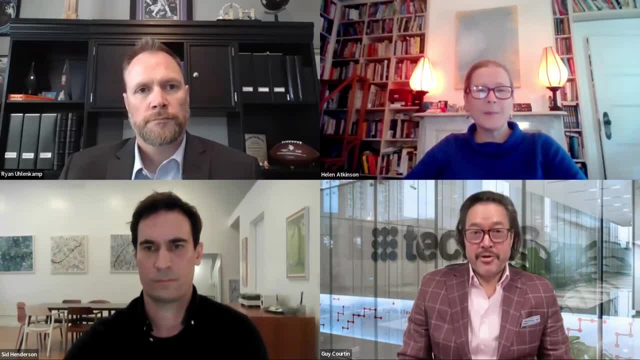 Guy, what do you have to say about that? Absolutely, I think that what I've seen more and more of- and this will take time to switch the mentality- is that our way of looking at ROI is starting to shift. exactly what you said, Helen: from a oh, 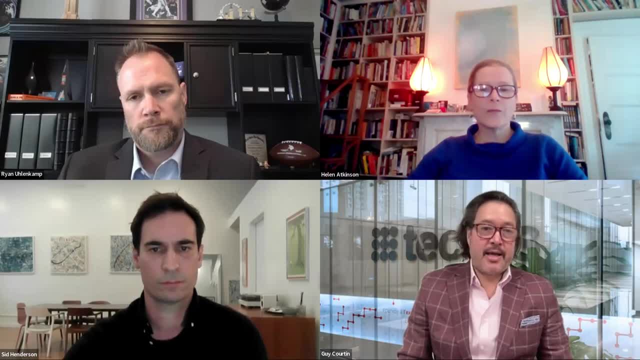 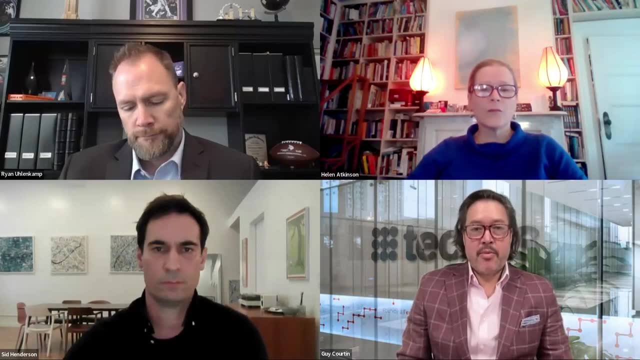 if I bring in X amount of robots, I save Y amount and I can cut Z amount of FTE. That's still going to be a factor And I certainly don't want to say that that is not going to be a part of the equation. 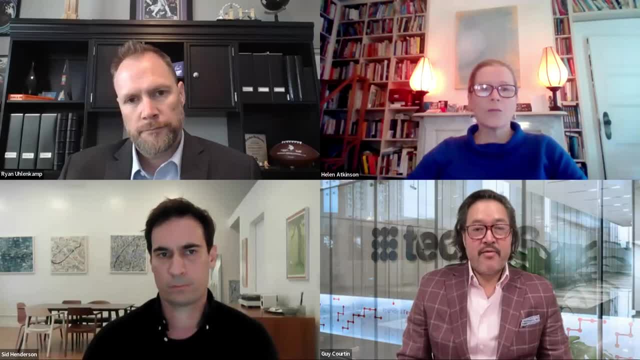 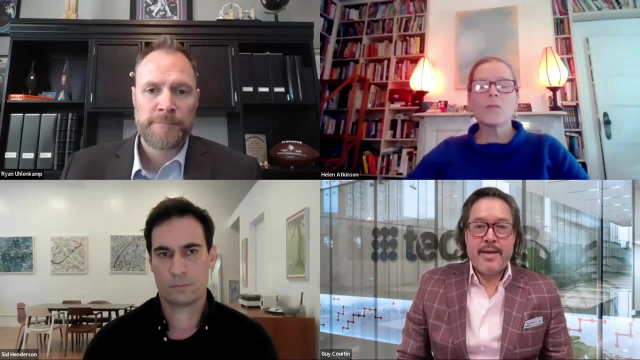 but I do believe that what we're seeing more and more of is that the savvy thinkers when it comes to automation are looking at what is more of the long-term viability of robotics, and how do we better, you know, measure what it's going to impact in terms of how I 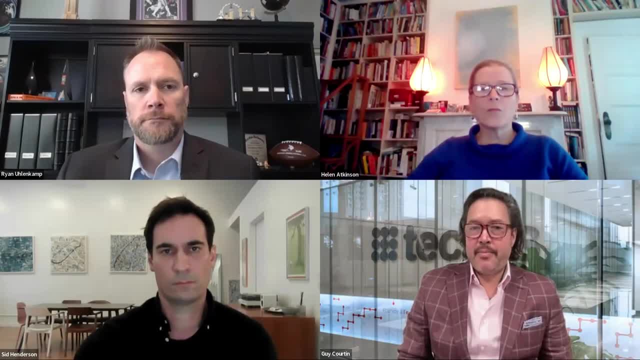 as a warehouse address my end customer's needs. Can I pick faster, Can I make orders more precise, Can I retain my labor, Can I open up new things I can do with my warehouse, because now I have automation. So I think those are all factors that are going. 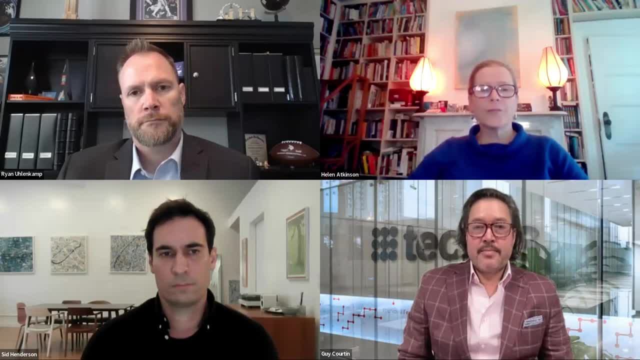 to the ROI calculation, I do think again, it's not the majority. I think it's still a small percentage of companies that are thinking this way and are able to express it. I think the challenge for the industry is: how do we come up with a more sophisticated ROI? 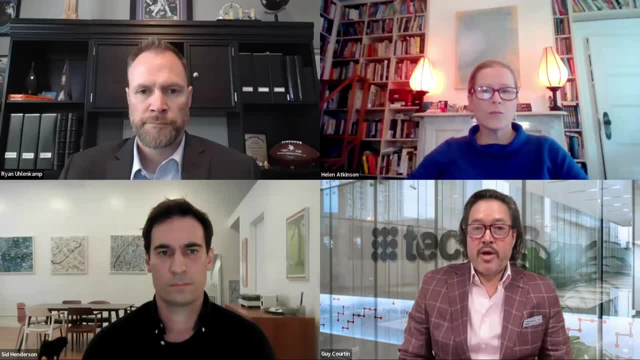 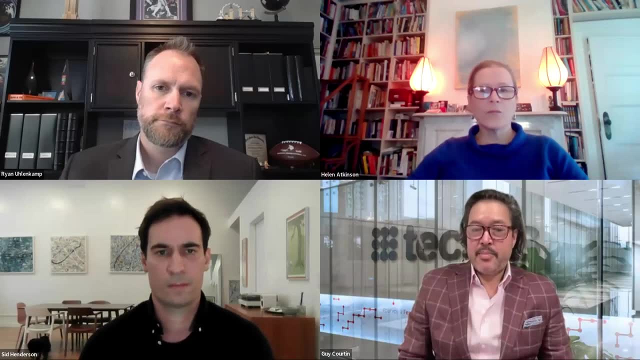 for these devices Because a simple equation of you know: bring in X, save you Y. therefore I do it. that's good, That's necessary, but that's not what I think is the long-term value prop of some of this automation. 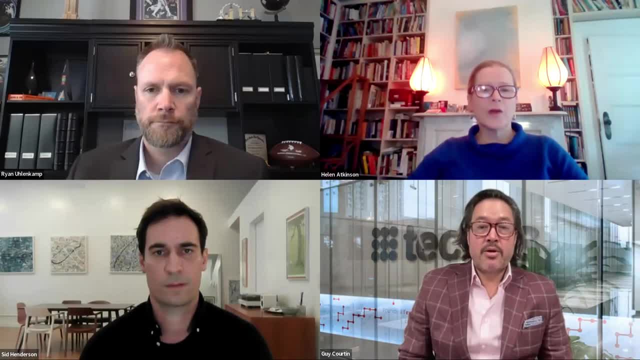 And I think again, that's a challenge on all of us, right? So how do we better create that vision, that model, that ROI equation, if you will, for people to invest in and to understand the long-term value of these devices? 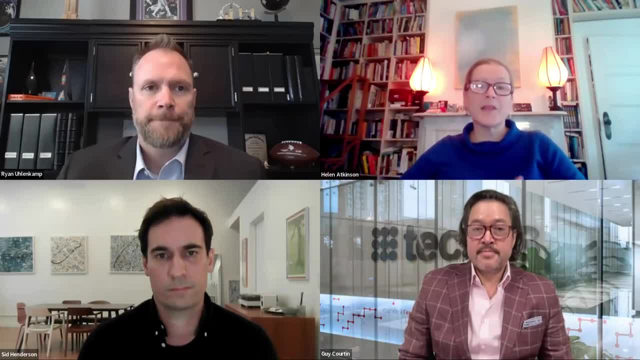 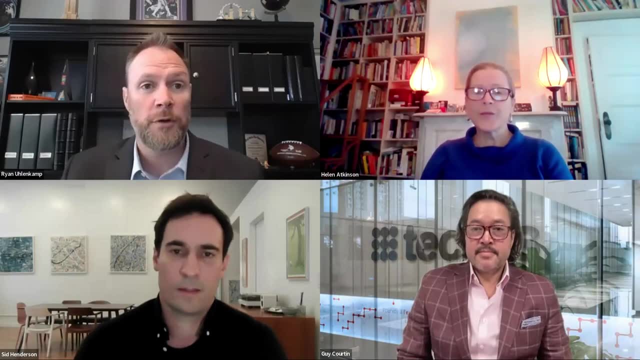 Right. so in other words, there are some soft benefits that are perhaps harder to measure, but should be in the factor. Yes, Ryan. Well, I was going to add one point or one word. I think resiliency is part of that play too. 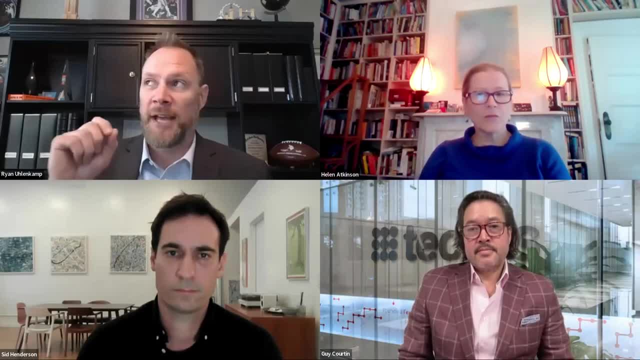 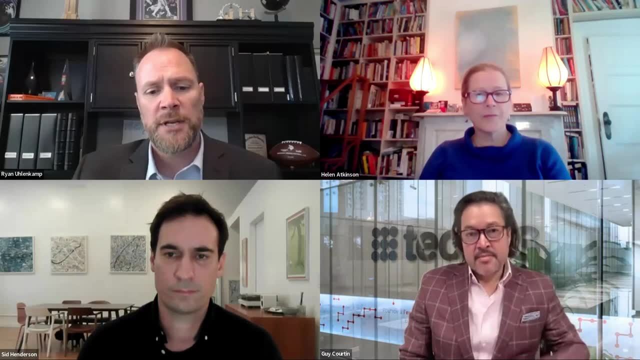 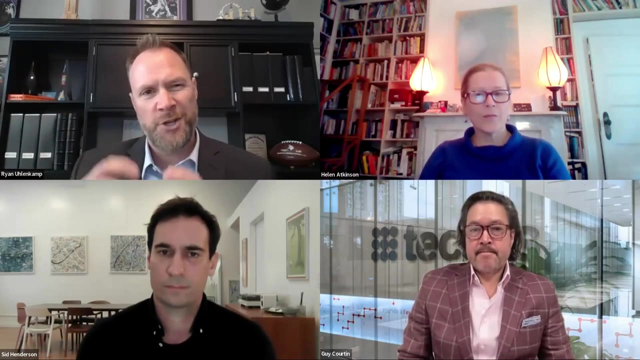 Like, automation is part of- not the but part of- because I'm big on the hybrid workforce and automation together. But I think automation is a key part to building up a more resilient supply chain And I think all of those things when you look at your ROI. 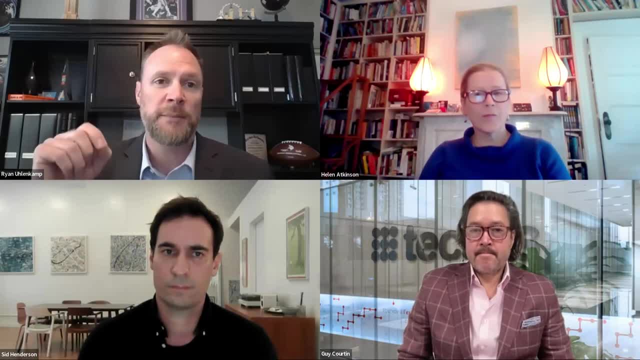 I think that pivots the way you look at that, If you look at how it can make you more resilient instead of direct return right away, more, how am I preventing for issues in the future? Yeah, that's great. And, Sid, do you have anything to add to that? 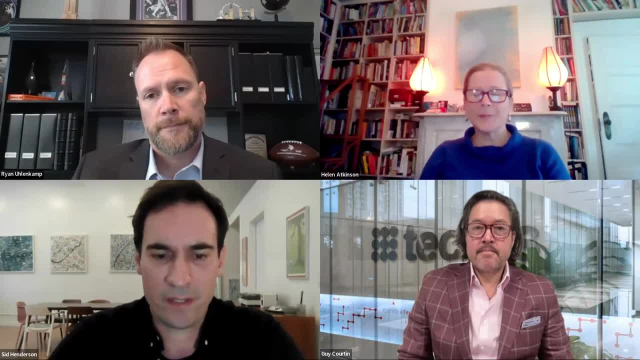 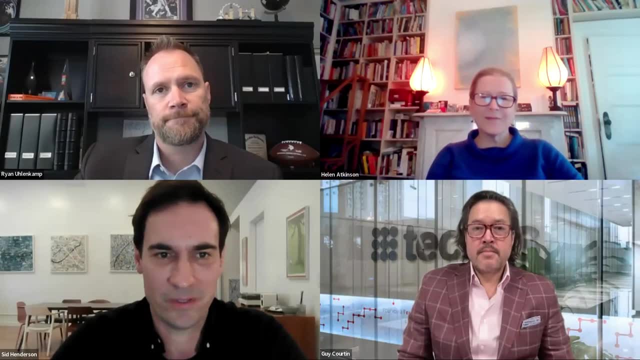 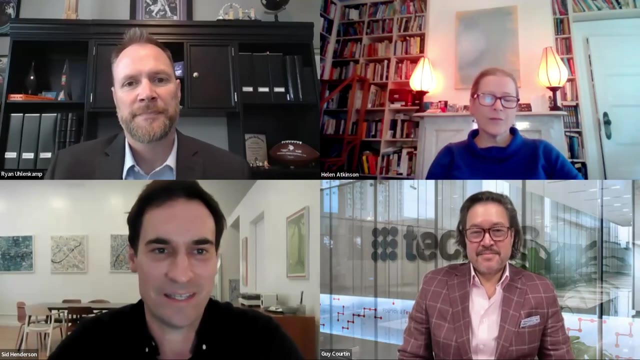 You know there are just so many benefits- And to automation, and it's always so important to decide how you want to look at the math, Like everything comes down to math And even for- yeah, even- for resiliency, like there's a math equation for that. 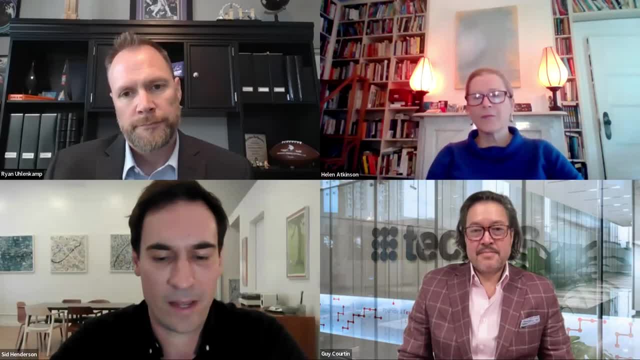 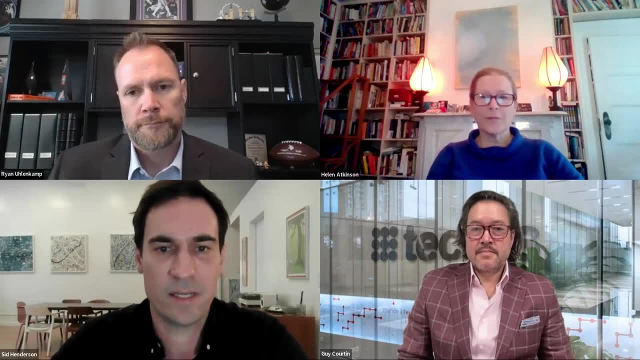 Are you measuring it And so you know when I'm thinking, when I'm talking about the ROI with potential ROI with customers, it's like, okay, let's get out a spreadsheet, Let's figure out where you want to go. 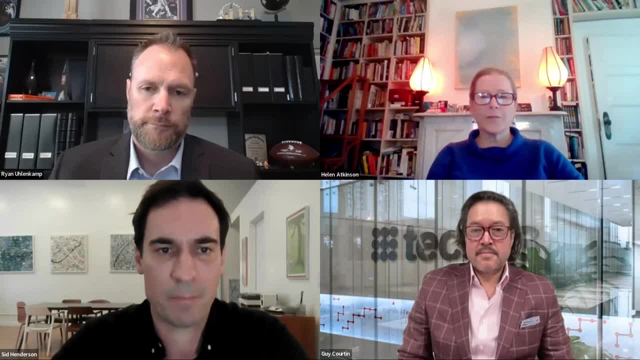 Let's figure out where you want to go, Find value And let's capture that value. And everybody has a different value function And it's just an important conversation to have with each project, with each customer Right. But I'm curious about what Guy was saying. 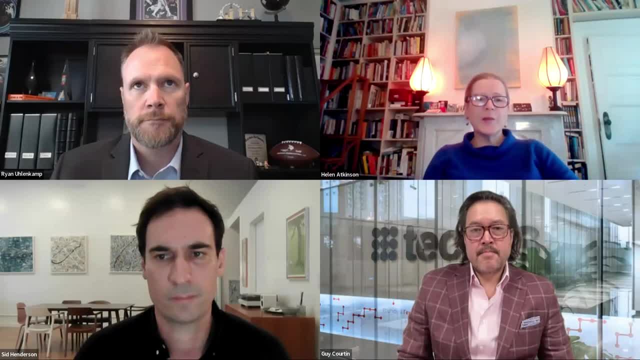 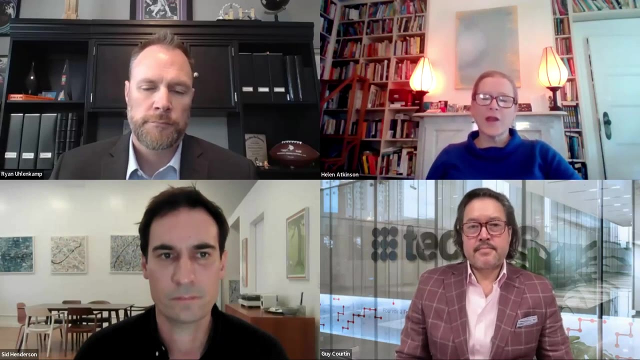 about sort of having to have a vision as well. Do you typically take potential customers to other customers' successful automated warehouses so that they can get a kind of wow moment? Or you know how, how do you encourage, how do you foster that sense? 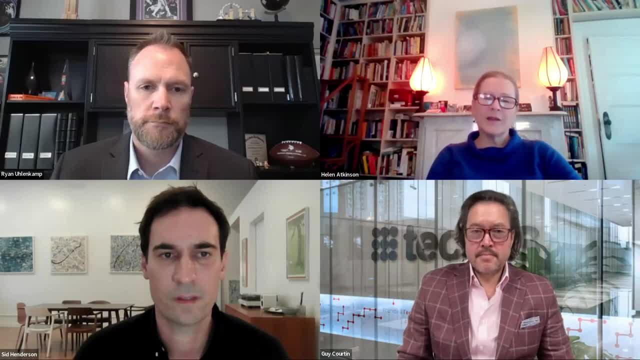 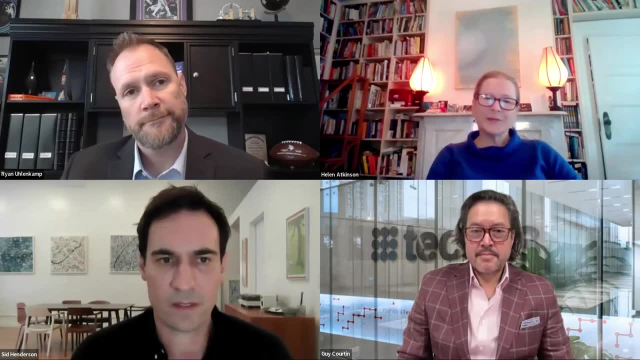 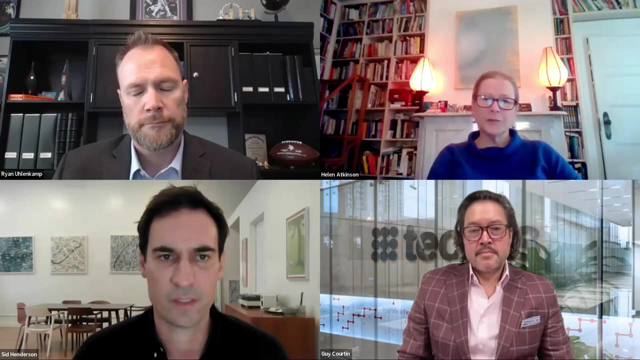 of vision when people are maybe just too focused on the math. Helen, that's for me. Yeah, sure, Sid. yeah Yeah, The customer visits are the most important thing, And we try to encourage those as much as we can. Not only is it a great way to see what your peers 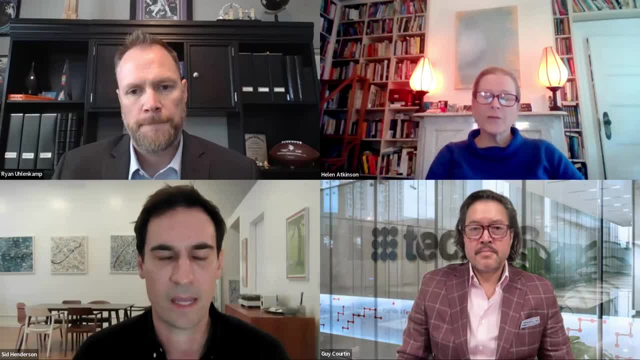 in the industry are doing and find out some areas for improvement. but it's the best way to talk to other customers who've installed the type of automation that you're interested in and asking them about the reliability, asking them about what the deployment was like. 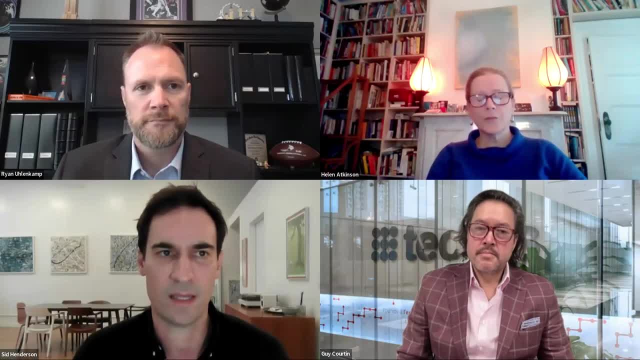 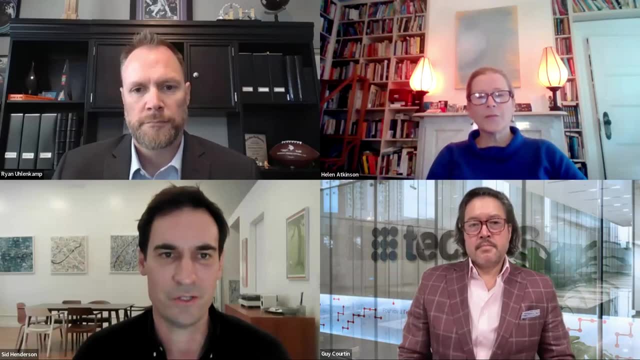 what that process was like. what are the unexpected headaches? What are the unexpected rewards? If you're hiring a new employee, you should be making three reference calls. If you're investing in automation for the next 10 years, maybe visit three sites. 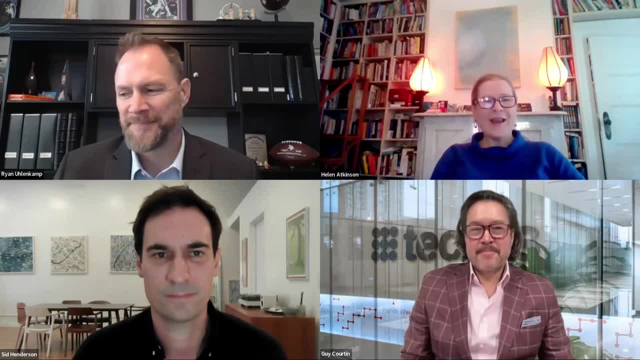 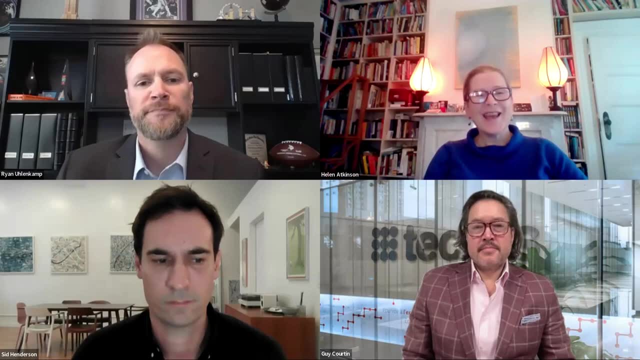 Yeah, that's a great tip, Thank you. So, Sid, there's another question for you. Let's talk a little bit about artificial intelligence. Where will we see AI working in combination with automation in the future, or is it already here? 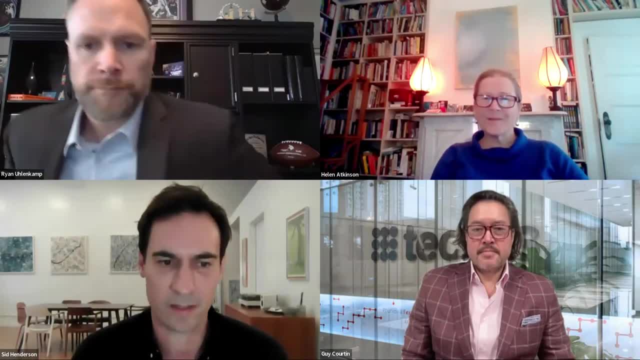 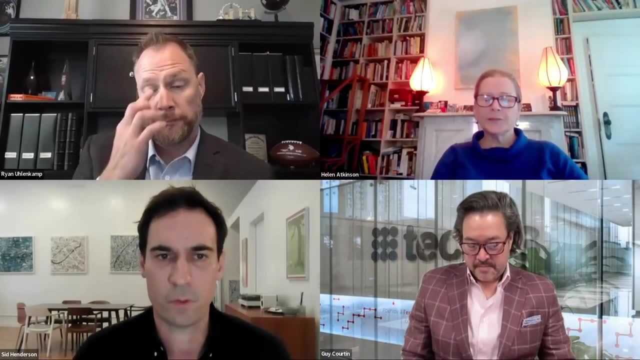 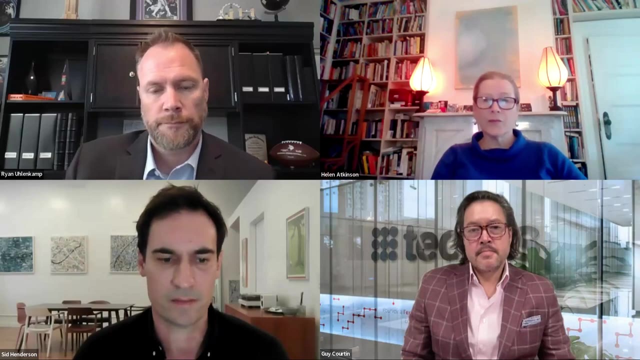 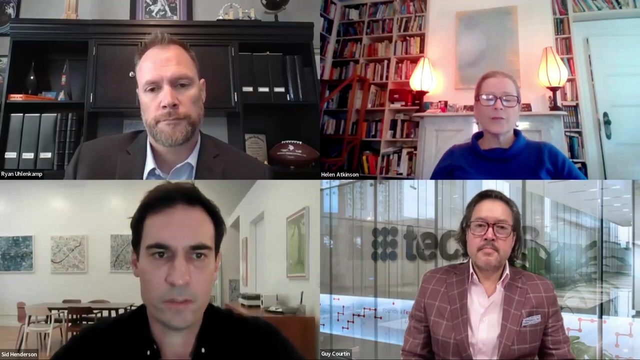 I'm a huge fan of AI and automation, specifically machine vision for robotic piece picking. I just think that's one of the coolest solutions that's newly available in warehouses. You know, I think that for the most part, the technology is ready for robotic piece picking. 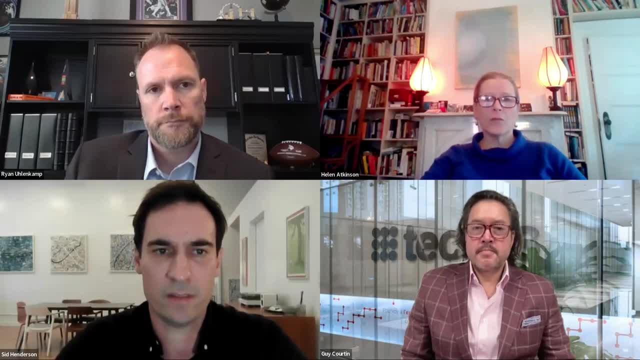 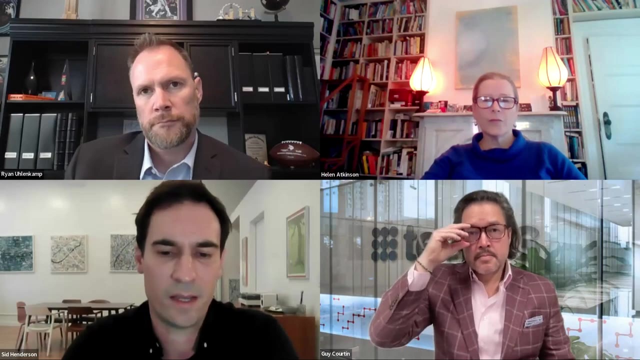 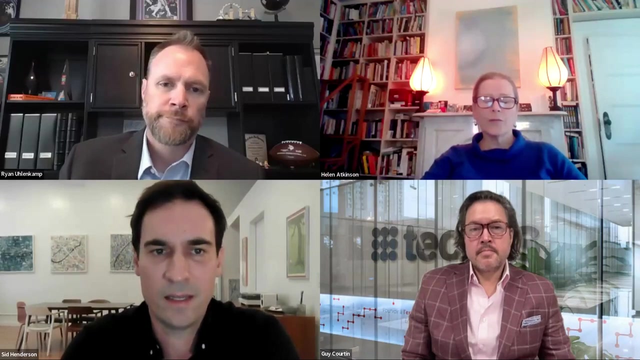 I think the real challenge is making sure the integration feels seamless, that it doesn't feel like there's a cost to figuring out how to integrate the AI into your warehouse. You know, something that's important to keep in mind is, even with all the amazing solutions, 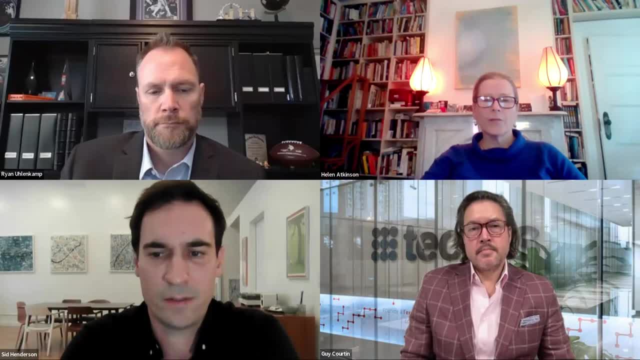 that have been available for automation. really sensitively is that you're not going to be able to do everything that I've been designing for you, And so you're just going to have to look at the data that you're using, and then you're going to be like 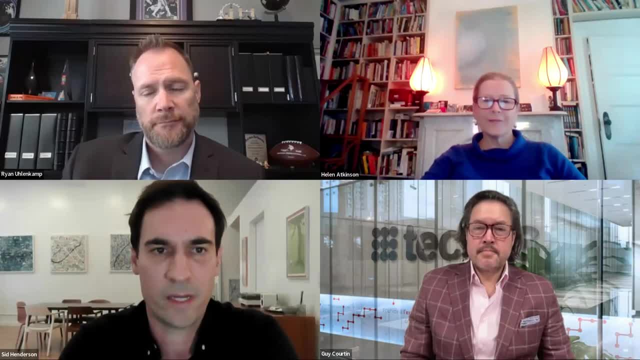 oh well, that's going to be mumble like no way, And you're going to be able to do that, And so, to me, I think that's a big part of the automation that we're working on. So, you know, I think we need to be thinking. 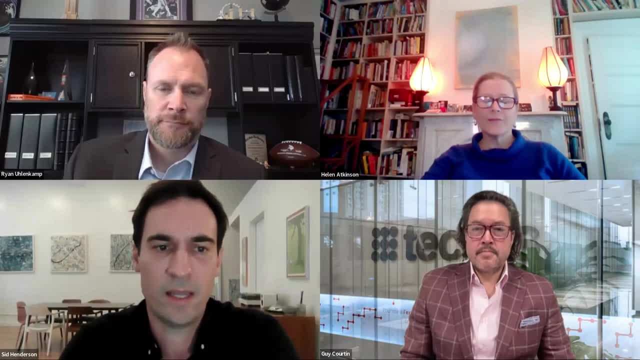 about where we are And I think our focuses are on how we can get people to understand automation and then also think about testing and trying to test robots based on the information that you're using, And also you know there's a lot of information out there, that's. 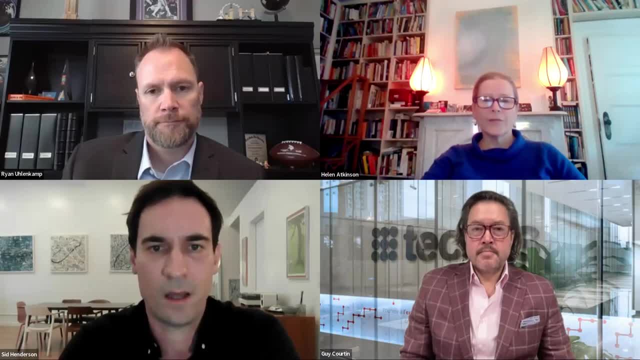 you know, I think we're going to need- because we need to get there- first We need to have the basic automation, the shuttle systems, the AMR solutions, all the ASRS options, and then we're gonna add on more AI after that. 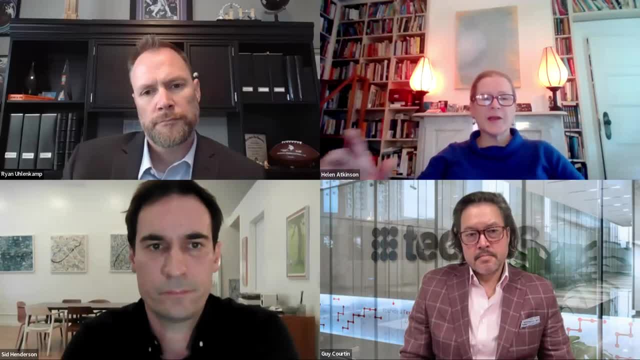 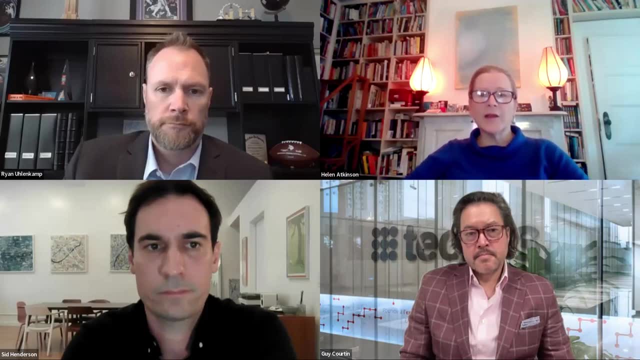 Right, but I'd be curious to know what each of you thinks about this. I think, from where I'm sitting, it feels like there's been a tipping point relatively recently, that I know it's taken a long time to embrace some very basic forms of automation. 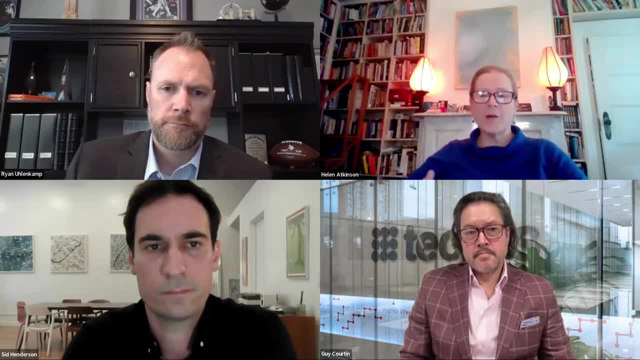 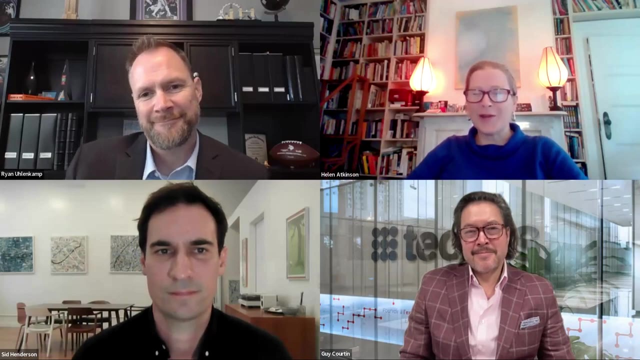 but it feels like there's a huge appetite for this now and that it's becoming going from being a competitive advantage to almost a must-have. or is that too optimistic? Am I being a journalist who's looking forward rather than being in the now? 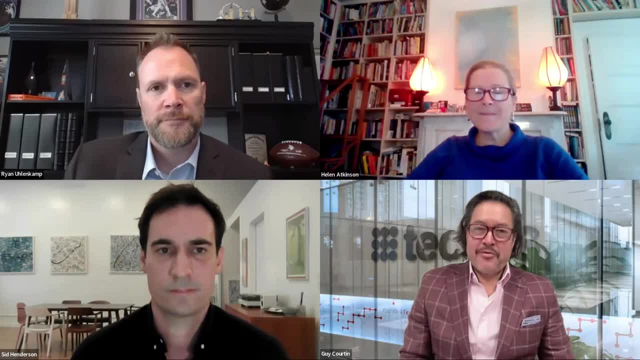 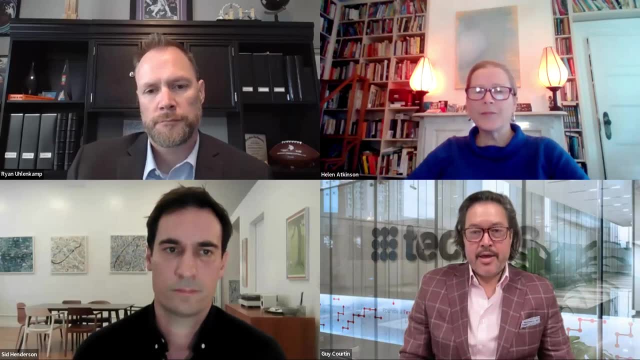 What do you think, Guy? I think it's a little of the above, Helen, I think part of it. if we take for sort of, if we decouple this right, we look at the heat, if you will right. 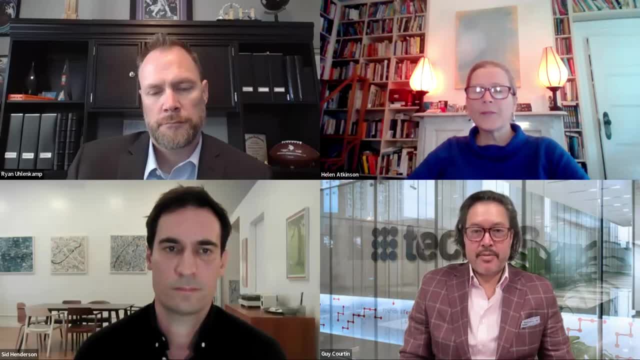 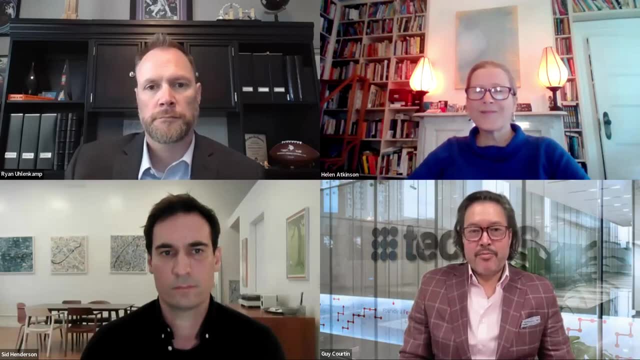 from a top of fold type discussion around AI, around robotics and automation. it's absolutely there, right? There's something there, but I'm gonna date myself here. You know, when I was in college and I studied computer science and it was last millennial, last millennium, right? 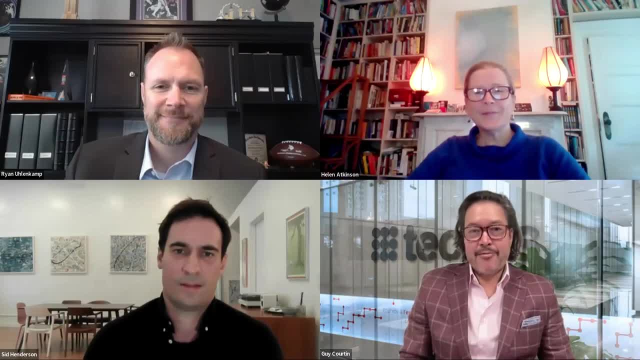 It was not in this century. I was already studying AI, right? I was reading books about AI and studying AI. So this notion of AI, it's like you know. it's like it's like you know. it's like you know, it's like. 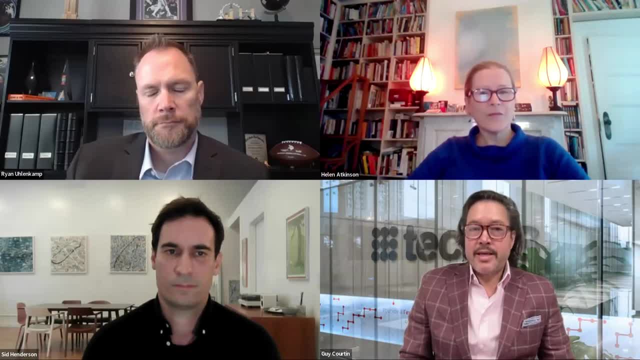 it has been around for a very long time. I think what we're seeing today is an explosion- This is true- An explosion of data. You know- you read statistics all the time- that mankind has created more data in the past, you know. 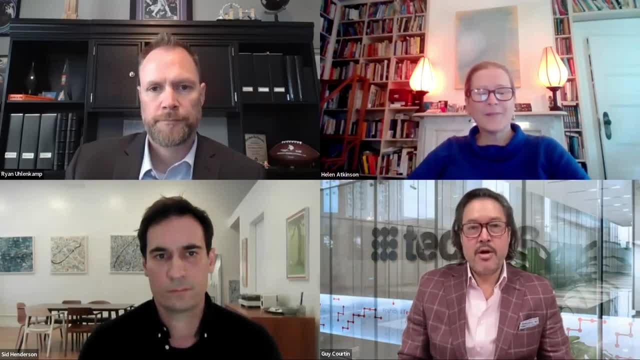 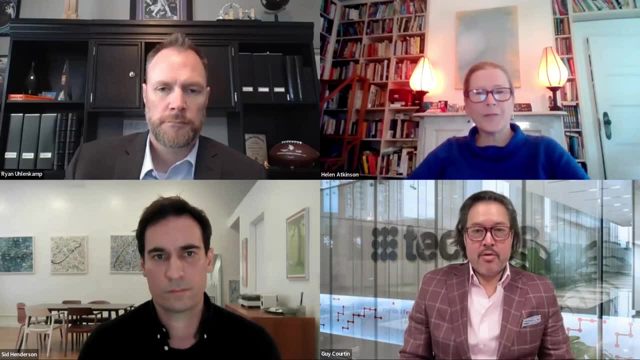 five years than we had in the past two million years. what have you? So the data is there, We have the computation. right now, because of computing and quantum computing And all this, we have an ability to crunch a course where we're getting all this excitement of. 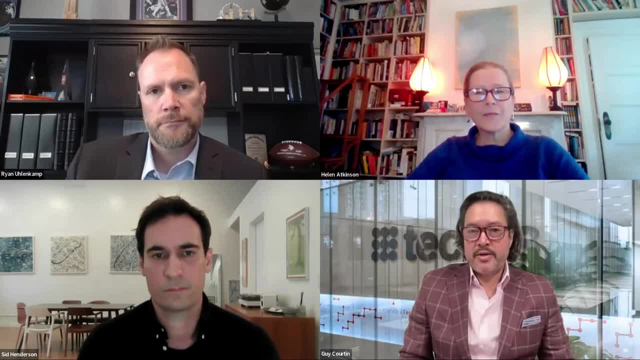 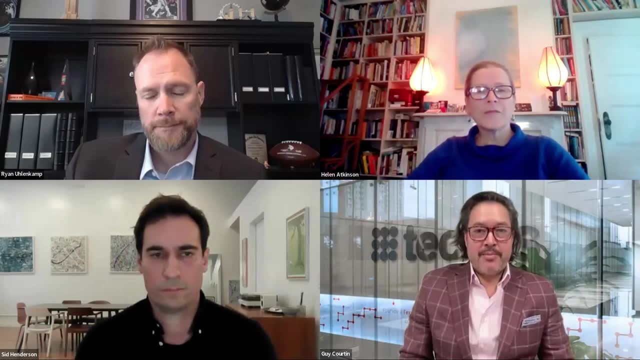 what is the art of the possible? What can we do with this? right To Sid's point right, We still need to be sober with this. The reality of the adoption rate of other technologies is still far behind what we assume, One of the things I always remind myself. 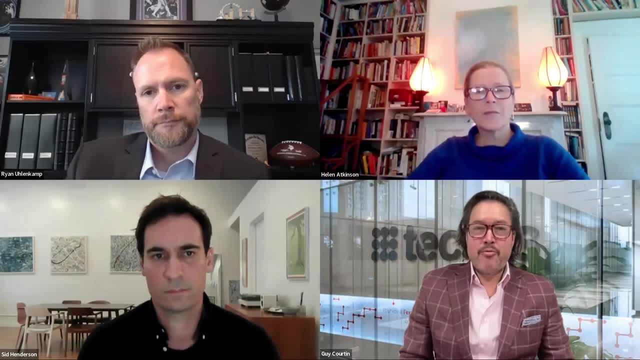 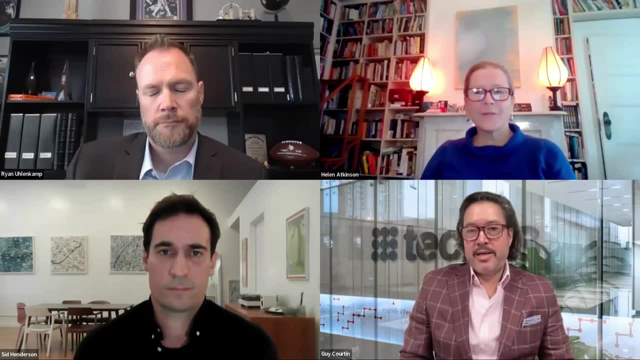 and I'm sure all of us on this call do is. you know we live and breathe this right. We just take for granted things like robotics and AI and computing. You know I go talk to folks in retail space and distribution. 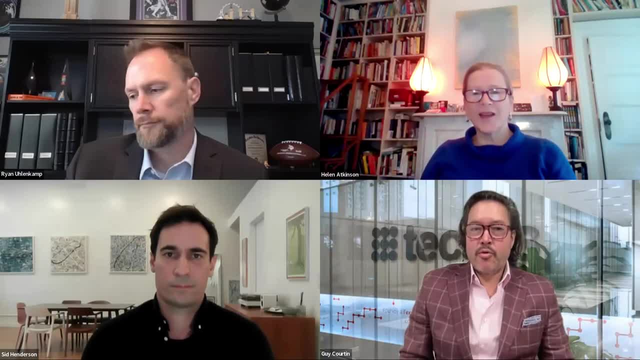 They're looking for healthcare and all this. and guess what? They've got a day job And they're not, you know, worried so much with regard to technology. They're looking for us to help them. So we have to realize there's still a chasm. 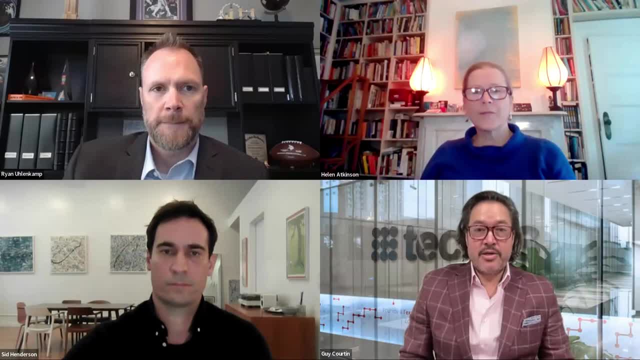 between where people are ready to adopt and ready to leverage with what we as pundits are talking and speaking and interested in Now. I do think that there's going to be a continued push of adoption towards this because of the need for it. 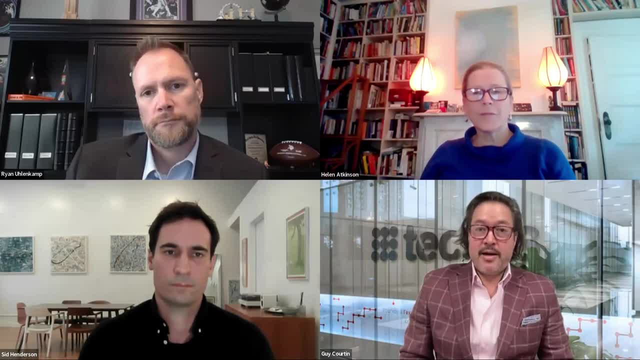 But I would. my caution is: I think AI has been around for a long time. I think it's it. there's great opportunities. I think there's great opportunities. I think there's a great future with AI. but I would just sort of pump the brakes at times to say: 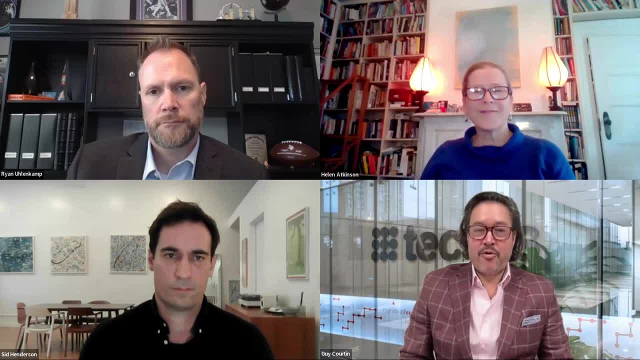 you know old fuddy-duddies like me, we've been doing AI for a while, So it's not something that just came up in the past five years. Sure, no, I mean spell check is, you know, auto-correct is AI, and we've had that for, you know, a while. 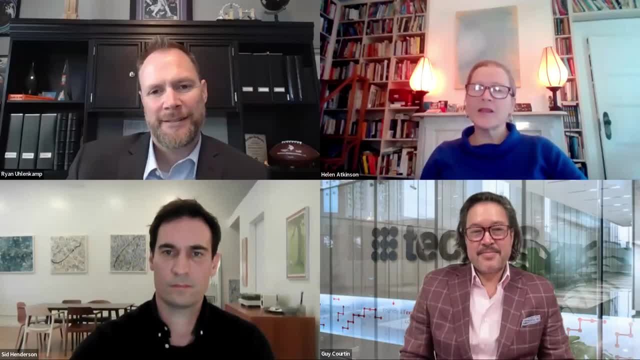 But just to be clear, what I was talking about was because I thought what Sid said was very interesting, that you sort of can't have a useful adoption of AI until you have a wider adoption of automation, and that there's been a slow adoption. 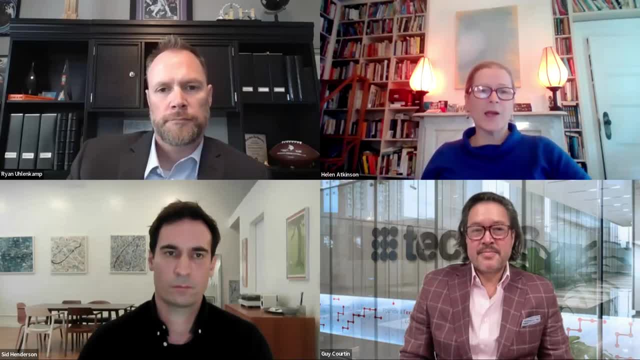 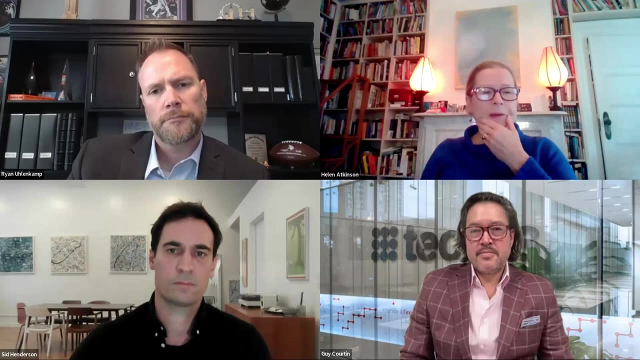 But it feels to me like automation, particularly, is really having its moment, particularly with all the sort of pressures in the market that we discuss. I just want to move along here. Ryan, same question, but in relation to labor management. we just heard about AI in automation. 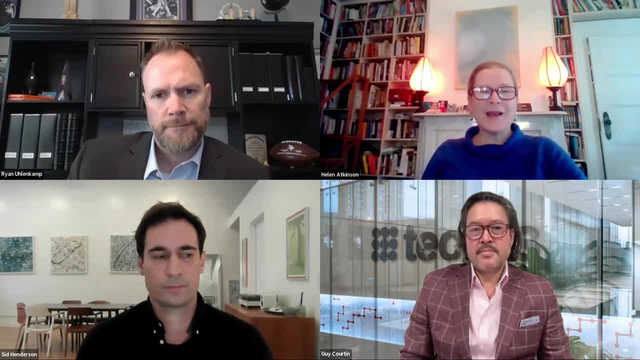 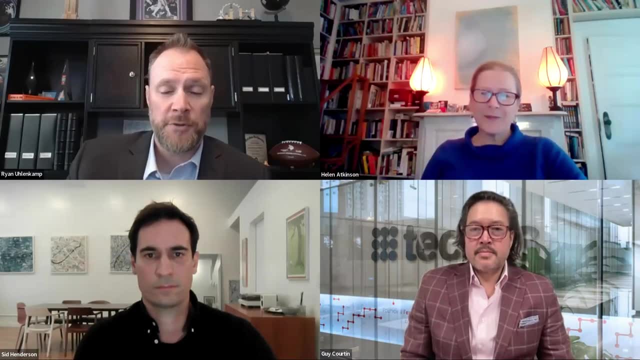 but how about in labor management? How is it going to be? how's machine learning going to be used to optimize labor? Yeah, I think there's a big opportunity for AI ML ingestion in labor management solutions and systems, and we've already started. 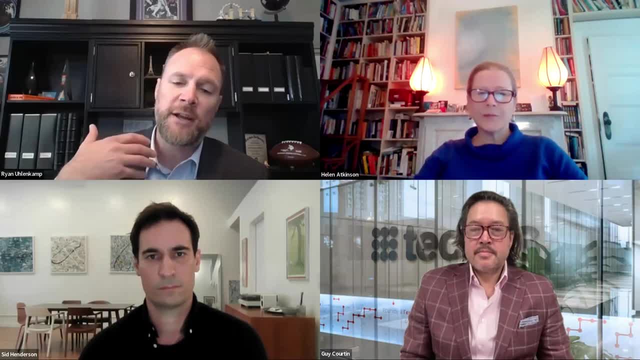 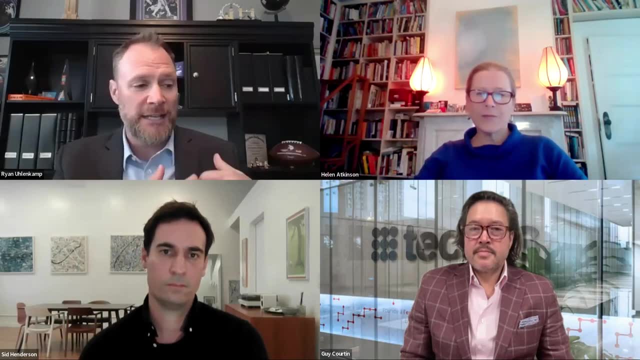 with our solution at Longo. We've started leveraging it in our labor planning tool. So, when you think about all the compute and all the trends and all the data, you have, like you said, this massive amount of data that we can reflect on. 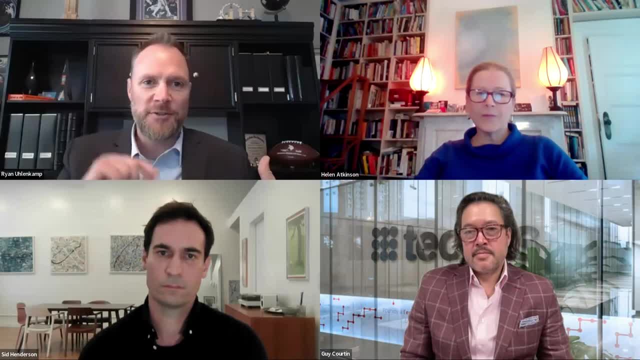 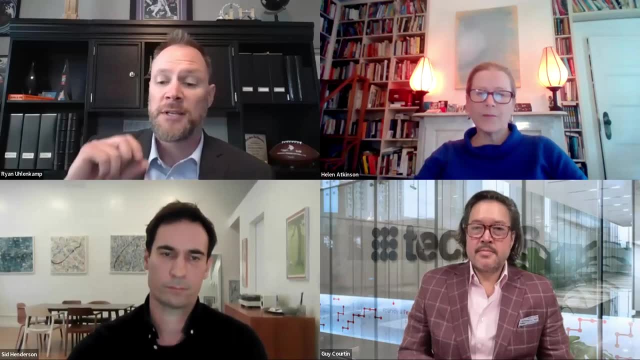 and use to start thinking about: well, what if I had done this or put staff this way, and continuously learning so we can get smarter and start to start our day with the right staffing, the right people? A lot of times, most warehouse managers tell you 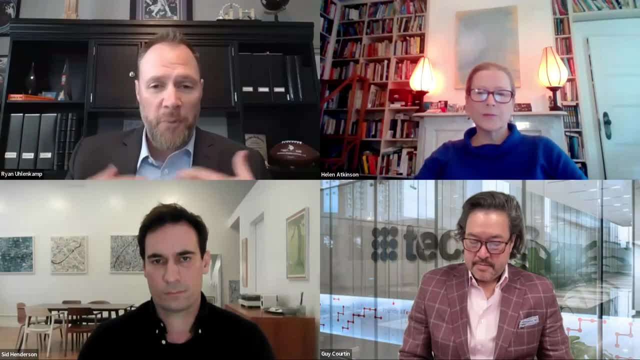 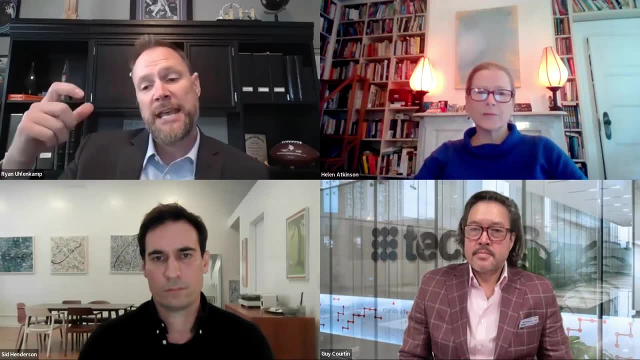 that their work comes in. they know the volume, but when it starts hitting is when they get a feel and they start adjusting people. I think so you can, on the front end, get better that intraday piece. I think there's a lot of opportunity. 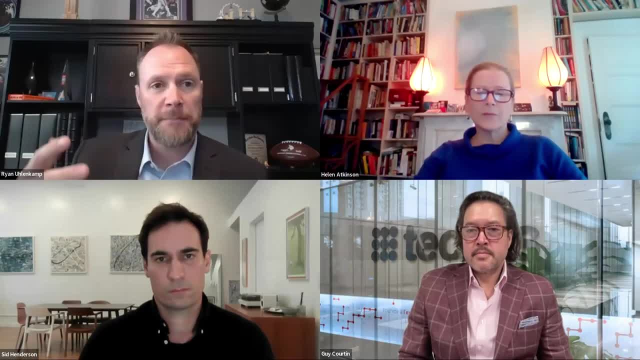 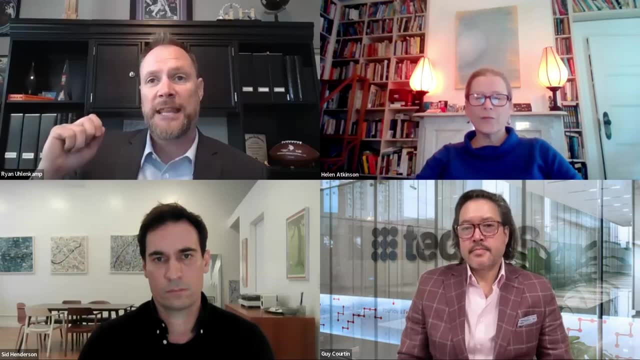 there as well. If you think about, I have a pick mod. I can look at certain jobs. maybe I can start to identify when congestion is physically starting to happen or learning, and then reallocate work in the queue to relieve that without any interaction, right. 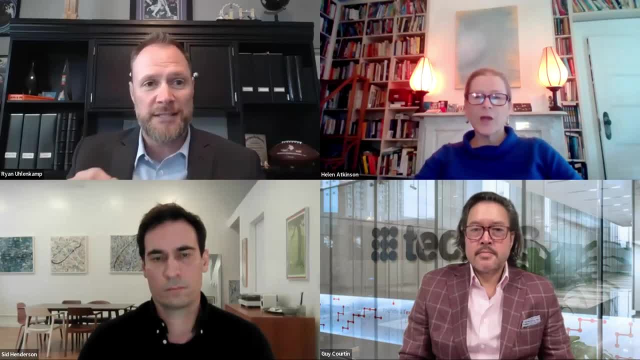 Right now, a lot of managers- that's what they're doing- is trying to watch an operation and make decisions. I think AI ML can do that. There's a machine scale to those computes, or even if you're somebody who has targets or labor standards. 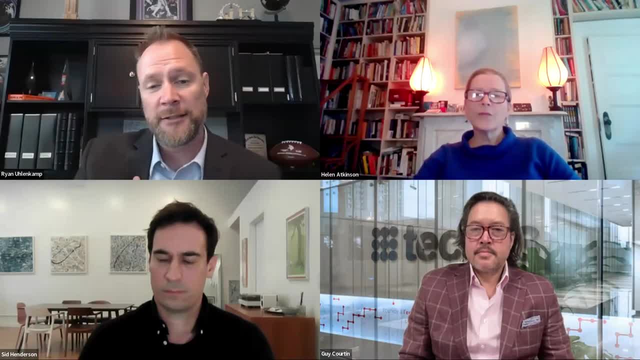 standards one of the things that always comes up if I work in Atlanta on a hot summer day. oh my gosh, this is a very different work environment, right, than what maybe a standard was based on, And I'm going to get all industrial engineering on you because that's my background. 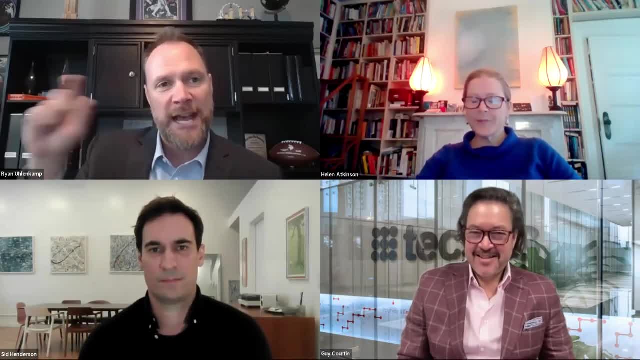 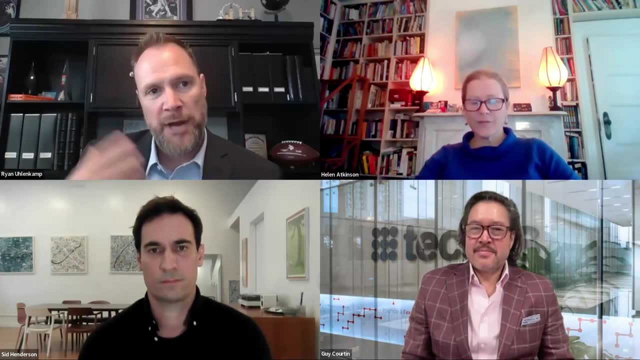 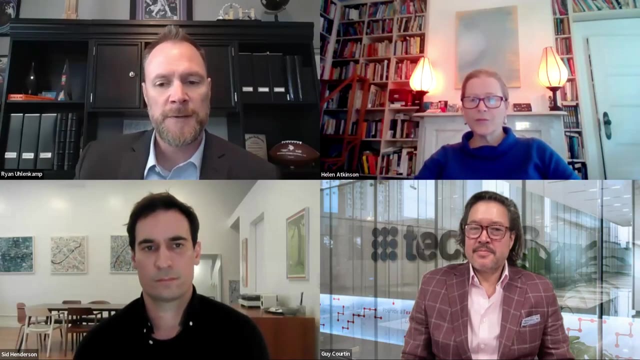 But my personal fatigue and delay allowances is sort of a static number historically. What if I could look at the weather and dynamically adjust that for that day, as those are happening? So there's a lot of opportunity, I think, to let technology start to do that crunch and calculation. 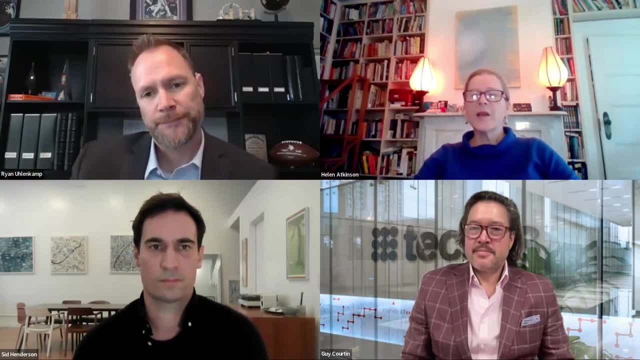 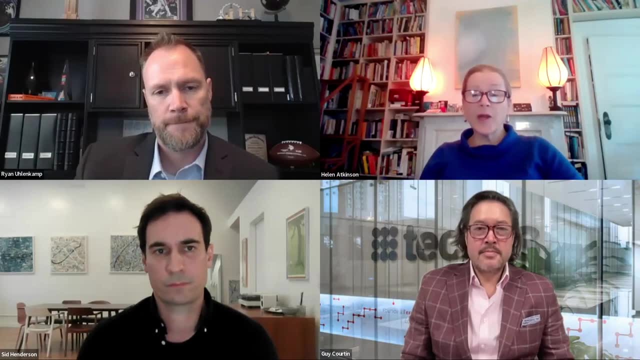 the things that's really hard for us to stay on top of Right. That's really interesting. So AI and machine learning be useful, not just for sort of selecting employees and vetting them, but also for managing them and deploying them in more efficient ways. Is that right? 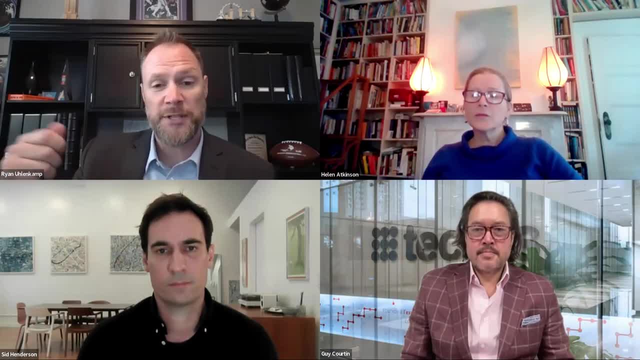 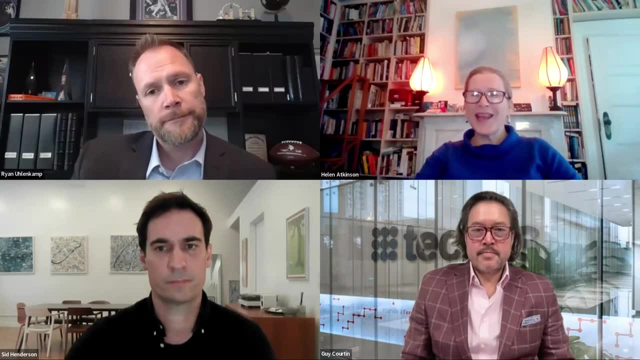 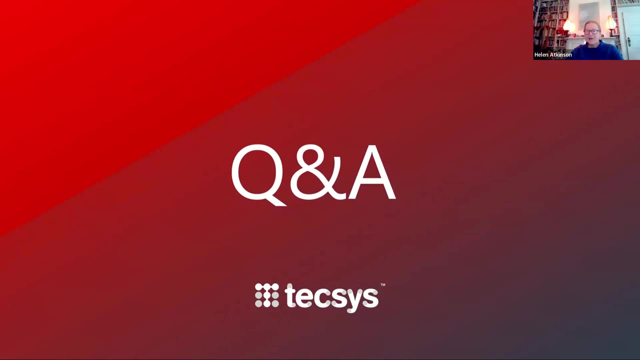 Correct. And going back to the comment, improving the user experience on the floor, Yeah, Wonderful, Thank you. Well, I'd like to move into our Q&A session now. Here are some questions from our lovely audience. I'm just going to take a look at what we have. 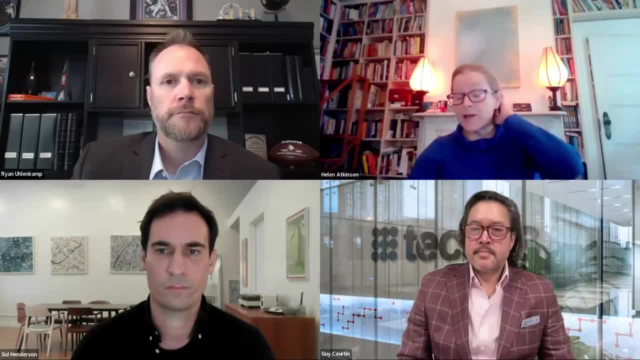 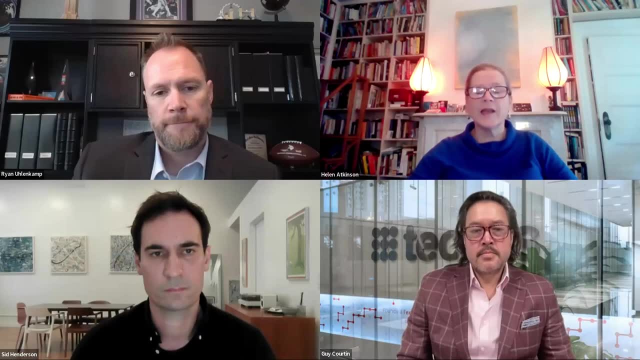 Oh, I have an interesting question here about language barriers. that, particularly in terms of training, I mean. obviously, America being the melting pot that it is, we have people who speak many different languages. How does automation help with reducing training time, particularly in the sense of making instructions more easily understood? 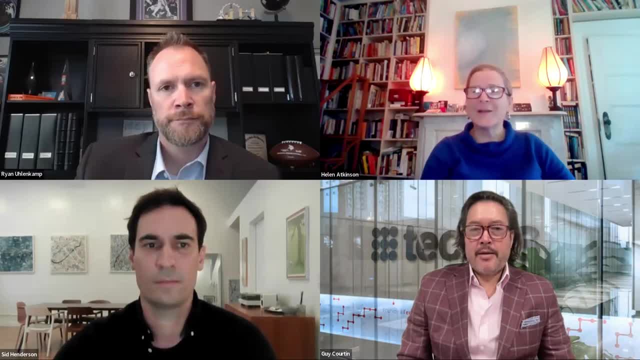 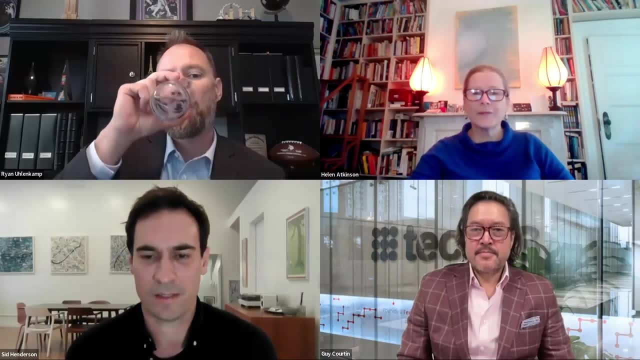 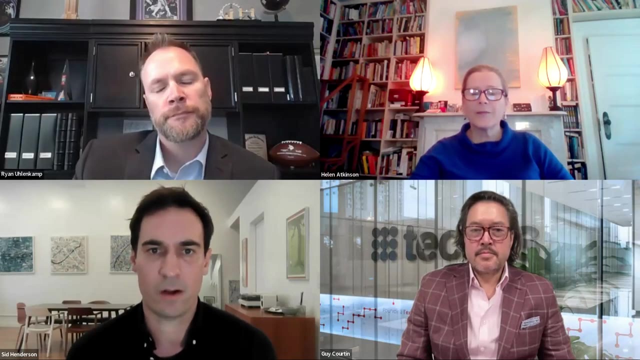 I'm trying to think, Sid or Guy, you can talk to that. Go ahead, Sid. I'm sure there are a million different answers for this, but for ExoTech, we, it is something we think about, We've put a lot of thought into And our interfaces. 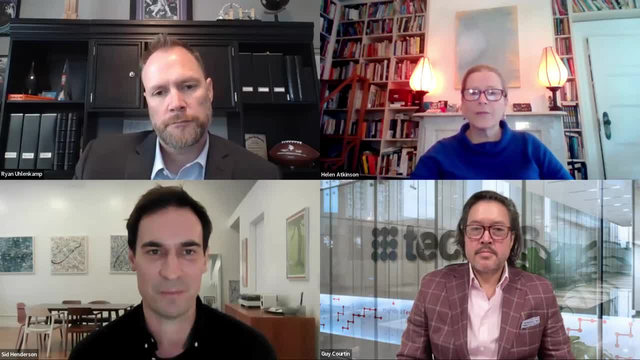 it's pretty basic, I guess. at the same time, Simple is good, But we have different language options. It's a very visual interface, And so pictures are worth a thousand words, But then we also just make sure that we have the flexibility in terms of different languages. So our systems are. 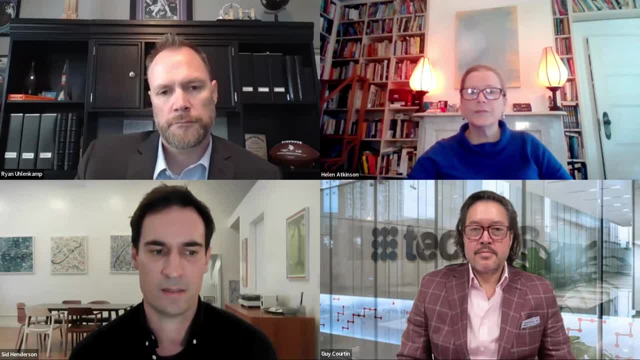 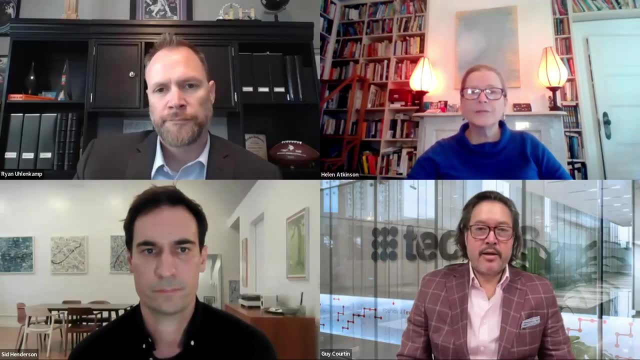 very simple for the operators and language barriers really shouldn't be an issue. yeah, just to build on what sid said: you know real quick. you know when i six river, the same thing. uh, our amrs, you know you would come up, you would badge in, it would identify you and identify your. 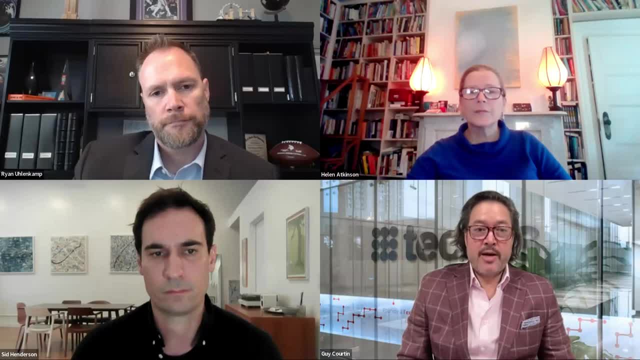 your language of choice and then the screen would bring up that language. so to the question about training, ease of use: a lot of visual cues, but also you know that that customizable from a communication language perspective, i think, the robotics, uh, and back to the ai and deep you. 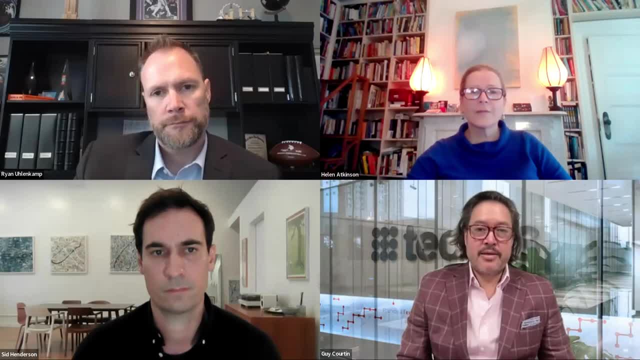 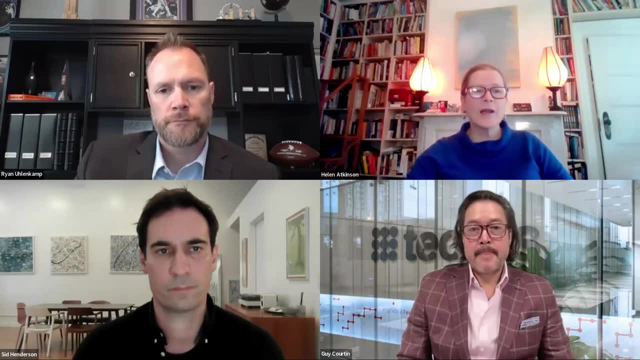 know machine learning and all this. that's where there's tremendous opportunity to leverage, you know that- that machine, so to speak, uh to help with training. fantastic, thank you. we're getting some great questions here. let me remind you, uh, we we very much want to invite your questions. 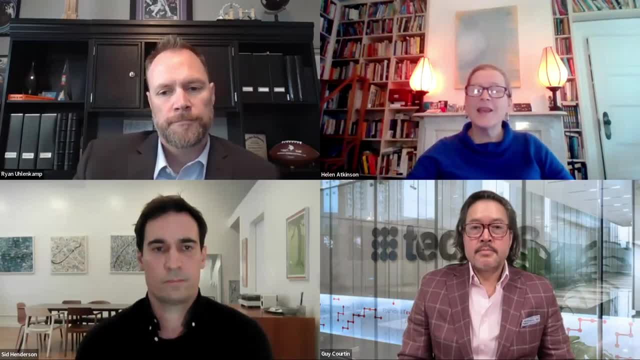 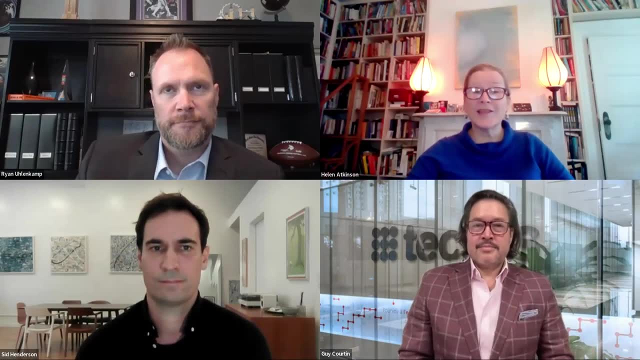 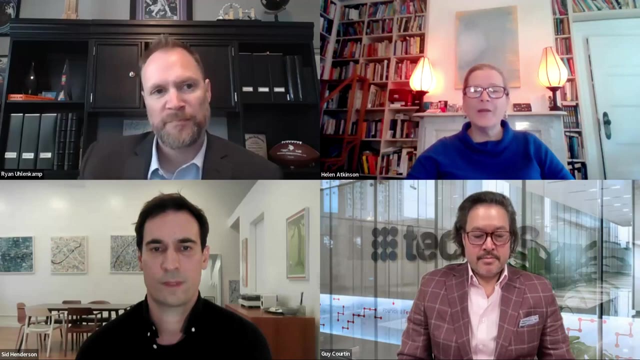 please submit your questions using the tab at the bottom of your screen, and we won't be using people's titles or company names, so feel free to ask anything you like, and if you don't see your question answered during the webinar, please be assured the texas team will reach out to you offline. um, i have a question here about uh roi and inflation. 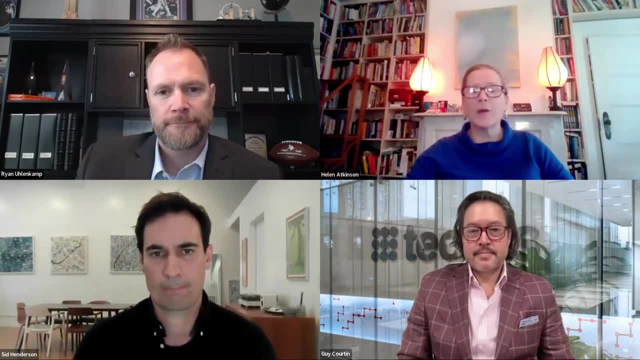 and i was wondering, uh, if you could talk about how. i mean, obviously we're in a period of highest inflation in decades. how does that uh play into the decision? say, for example, putting in a cube density solution that could perhaps reduce major capital investments for the size of a new structure. that's probably one for you. 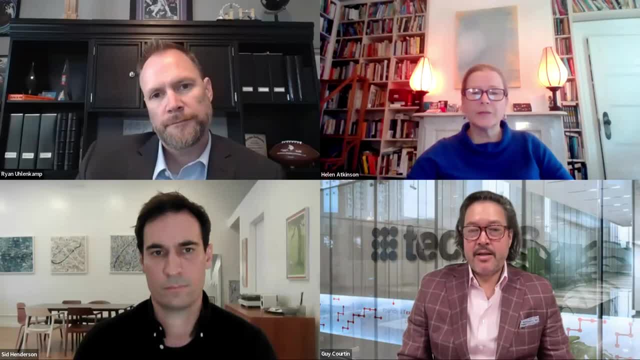 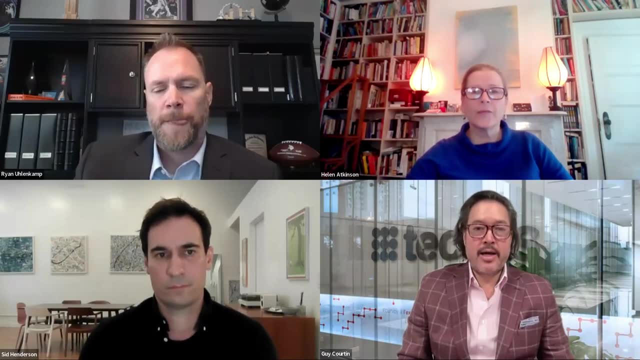 yeah, no, that's a. that's a good one. i i think it's a. it's a valid discussion point. now, when it comes to looking at, you know, macroeconomic factors like inflation into the rroi calculator. i do believe it's one of those where, if and when, you're looking to make an automation investment. 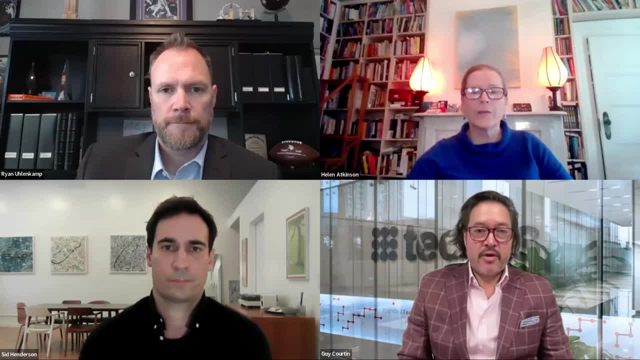 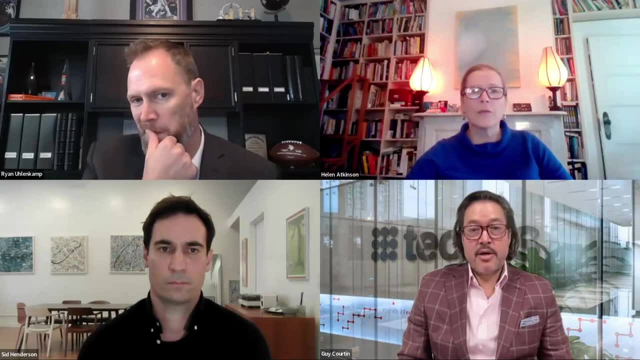 is to work with whomever you're you're selecting, and then you, if you're a consultant, to calculate that in, and part of that calculation, i do think, also falls into: is this a capital expenditure? is this, uh, you know, a rental model, so to speak, a sas model, because that also could defer some of the costs? 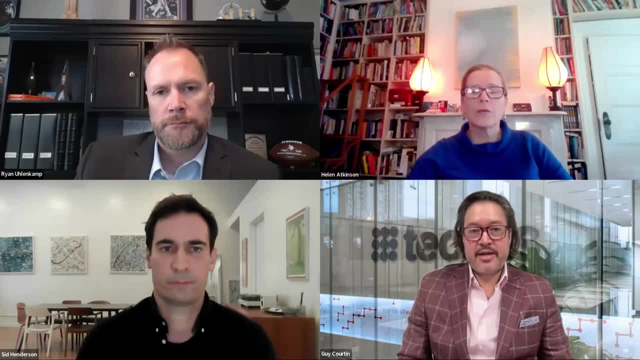 and get around some of the inflation- you know inflation issues- we have today. i will say this, though you know, one of the one of the macroeconomic aspects we have seen with regards to this is, you know, some automation. uh, it is capital intensive, so you're going to be paying more for. 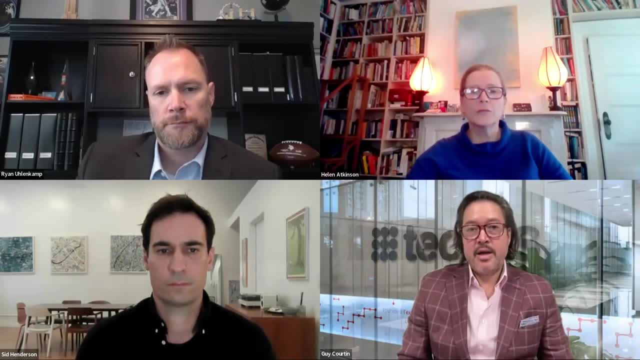 commodities such as steel and rubber and glass and all this while, as others, if you're just getting a mobile robot, you're gonna be paying more on a rental service. so i think that inflation question is is unfortunately wearing its ugly head in the past few years because of the trickle down effect it also had on the price of commodities. 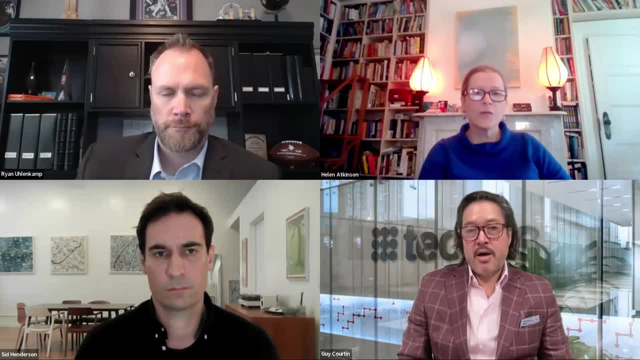 again, such as steel and rubber and plastic and all this when it comes to putting your, your robotic structure, in there. so you know there's no easy answer. i think that's really something that you have to consider with the vendor you're looking or with the model you're building. 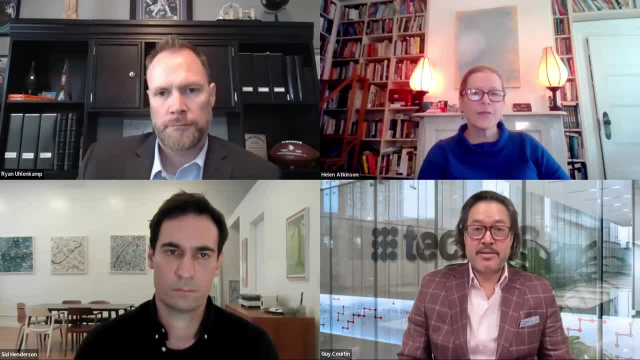 but also thinking about how it might impact other aspects of that robotics supply chain as well. Right, Yeah, yeah, That's a great point, Guy. Thank you, Sid. here's a question for you. We mentioned earlier- you mentioned earlier- that you want to. 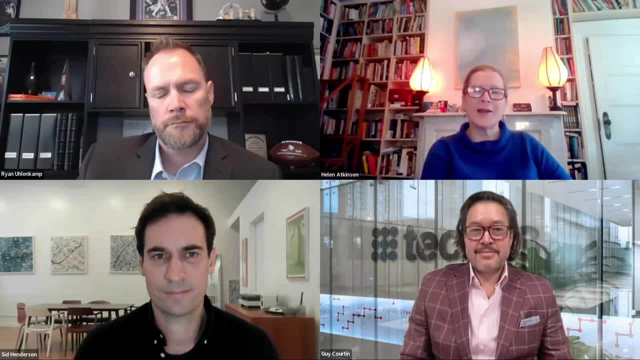 or I think it might have been Guy- that it's a good idea, if you're going to spend $10 million on an automation solution, to visit three sites where it's already happening. And the question from the audience is: how do you find those three sites? 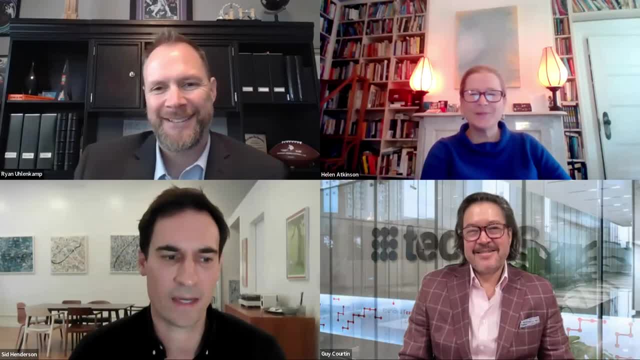 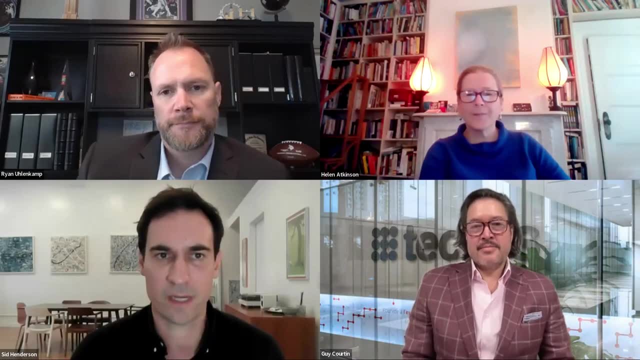 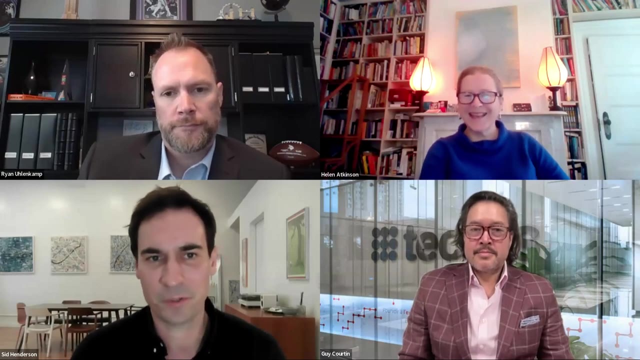 I like that question. So at Exotech we have a lot of sites globally that we're proud to show off to prospective customers. Next year we're also rolling out something we're calling ExoTours, the Exotech World Tour. 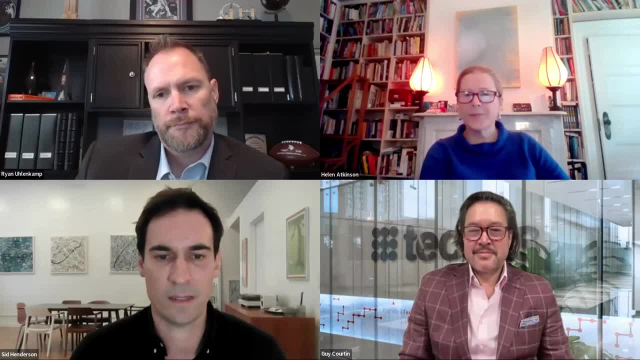 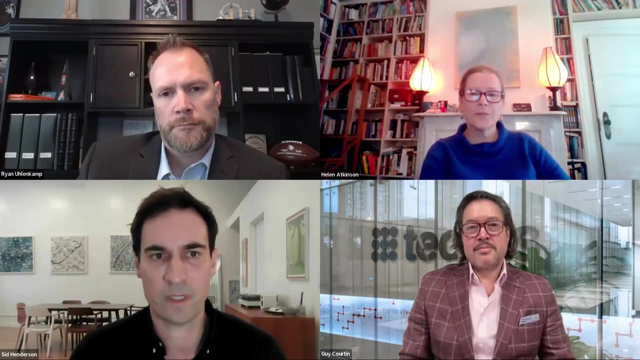 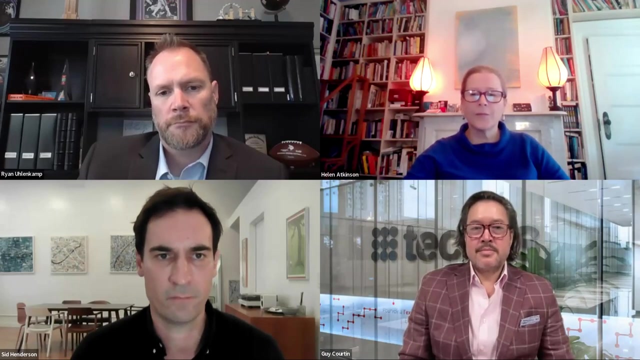 where, every month, we're going to be opening invitations for our customers to come meet with us in a different city at a different customer site, And I think that's expected to be something that different customers at different part of their customer journeys will feel happy to join us for. 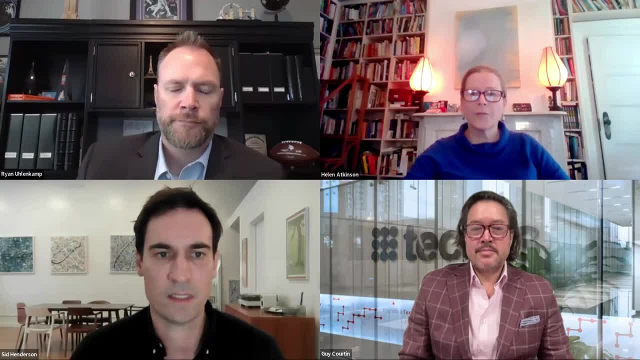 But yeah, it is so important to see different types of warehouses, even for the same solution provider. A lot of our warehouses look very, very different from each other and you learn a lot with each visit. Right, I want the T-shirt from the tour. 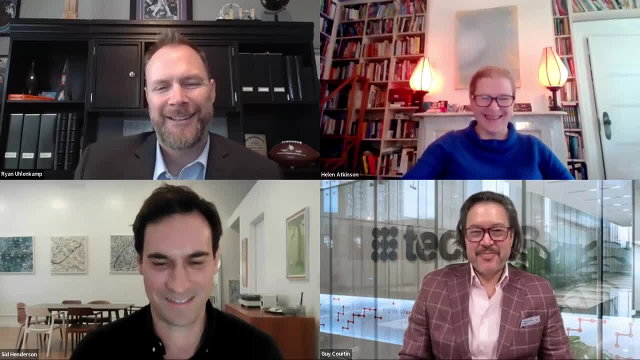 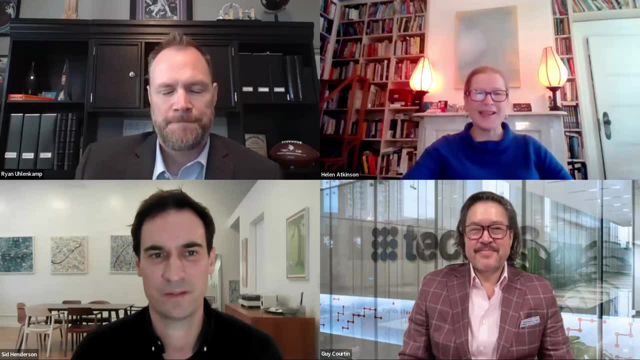 I was about to say, I look forward to that tour T-shirt. It'll be epic, Trust me, Fantastic, And I seriously I would like to come on some of those site visits too. That would be great. I'd love to have you on. 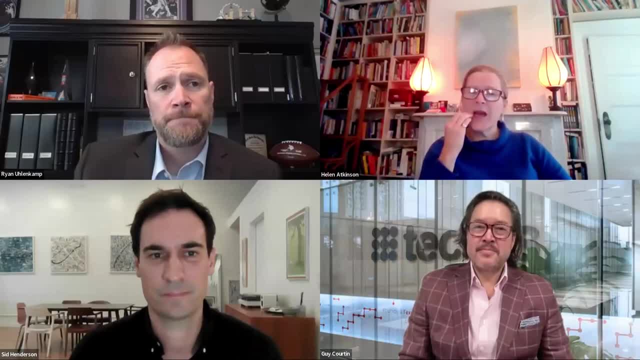 Thank you, Ryan. here's a question for you: What are some of the modalities of human to machine interaction that you are seeing right now? specifically, do you see voice as a useful mode? Sorry, I mean sorry, that's partly labor. 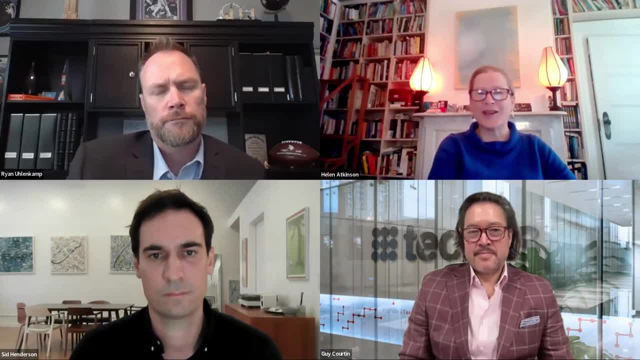 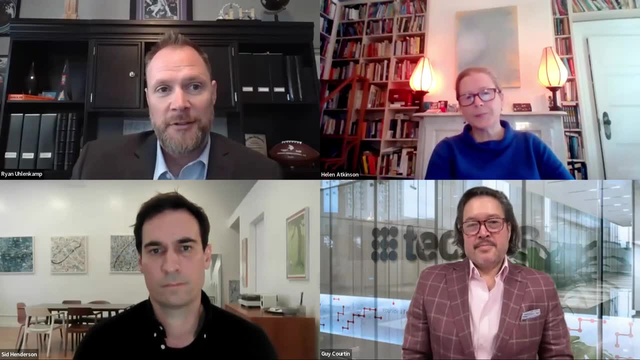 but it's partly automation. So, Ryan, start off and then we can hear from me instead. Yeah, I think you're seeing a combination of voice. So what I? when I think of voice, I think of the old vocal act, not old. 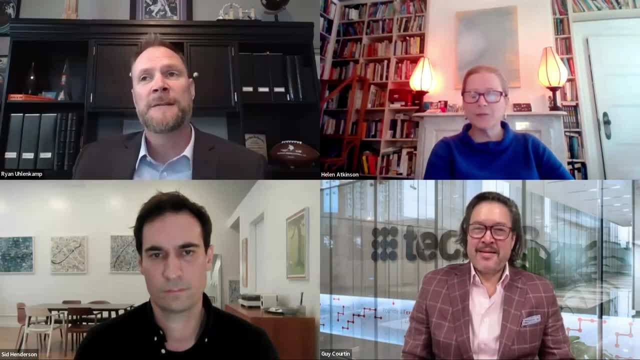 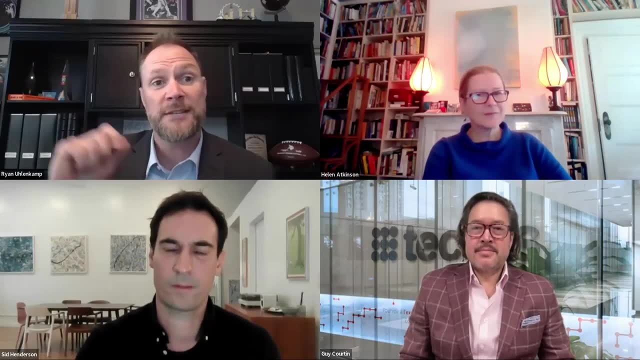 but I mean vocal act solution, voice pick solutions that free up the hands right. I've been to more warehouses lately that have sort of a merge of voice and a scale. So I think voice is a play, I think voice with automation 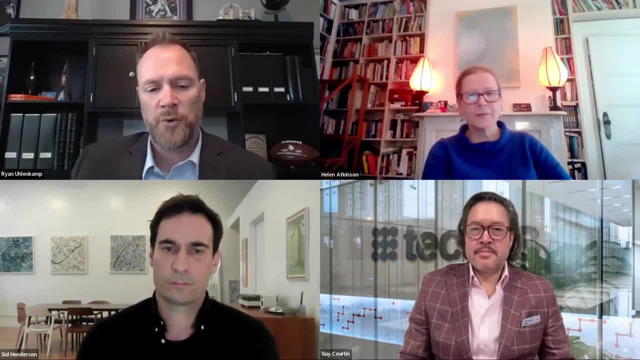 I think it's going to get. it's always. how do I improve that user experience? How do I free the hands up to do the work right? So I think voice is a play. I think voice with automation is a play when you start. 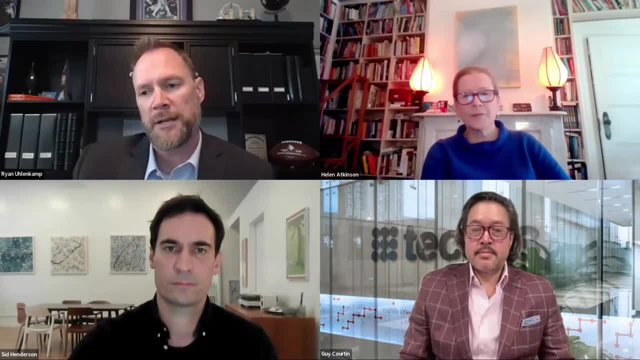 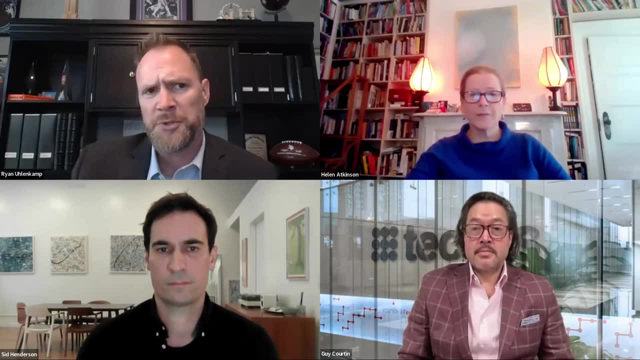 There's that nuance then, to make sure, with language barriers, but obviously that's come a long, long way from when we first started doing voice technology. I think there's a. I think those, those will definitely come together for sure. Yeah. 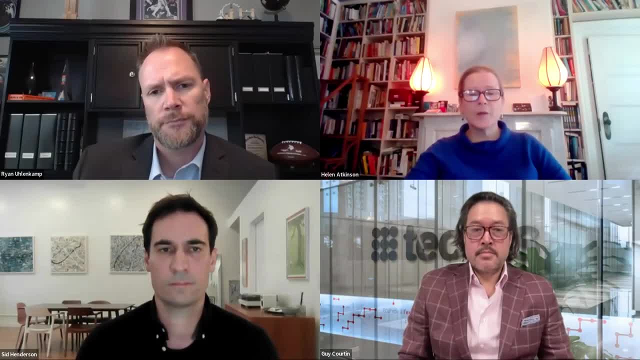 Yeah, Yeah, Yeah, Yeah, Yeah, Yeah. Fantastic Sid. what do you see is is voice still at a useful mode? You know I I'm going to defer to Ryan on that because it's not- it's not part of my wheelhouse as much. 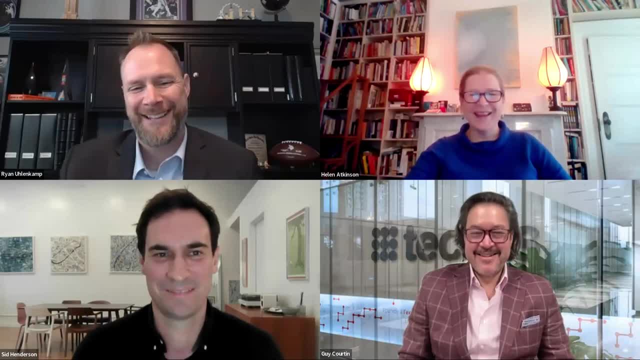 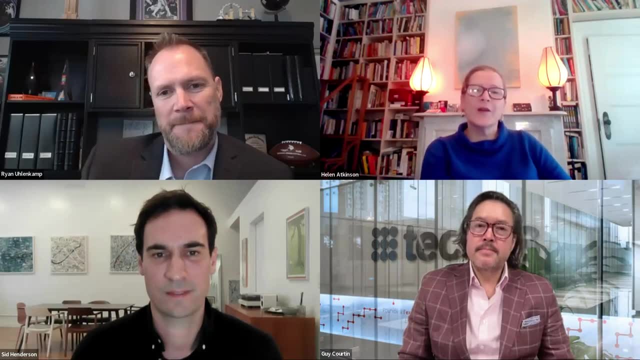 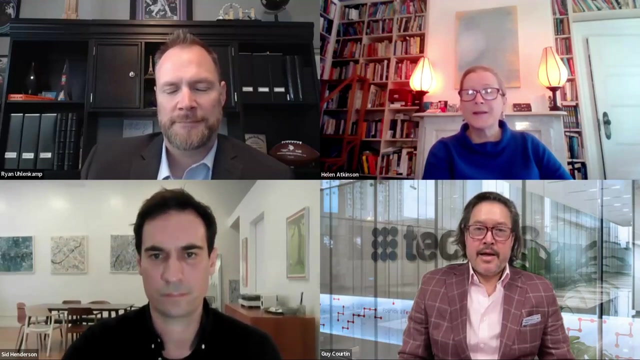 So I'm I like his answer. Okay, Thank you. So here's an interesting question. Automated automation streamlines processes and sometimes limits flexibility. What's your take on this, and what practices ensure flexibility with automation? I can take a first pass to that. 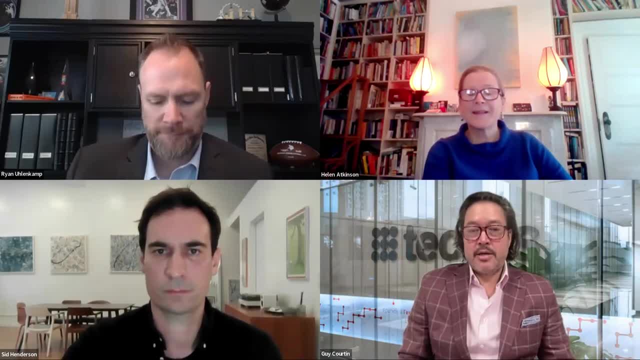 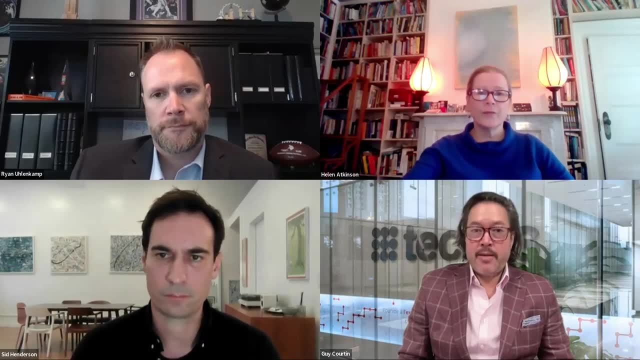 I I think this begets a larger question around automation, and where is sort of the line being drawn in terms of does automation keep, keep labor also, sometimes maybe even more into a, a sort of a lane, and all you do is this? I think that goes back to the question of 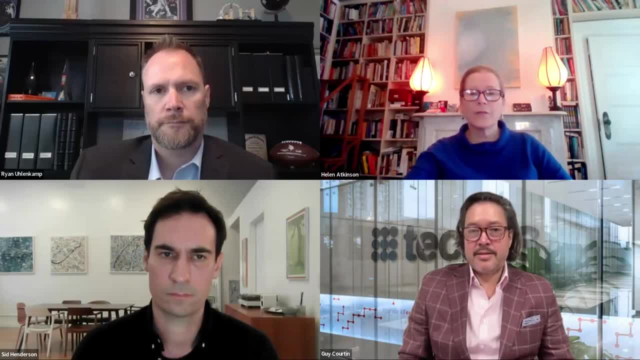 all the different flavors of automation, Right, Whether we- we talked about this in the beginning, about you. look at your warehouse, right. There are dozens, if not hundreds, of use cases in your warehouse where automation can play a role And within that there's going to be different vendors and different types of automation. 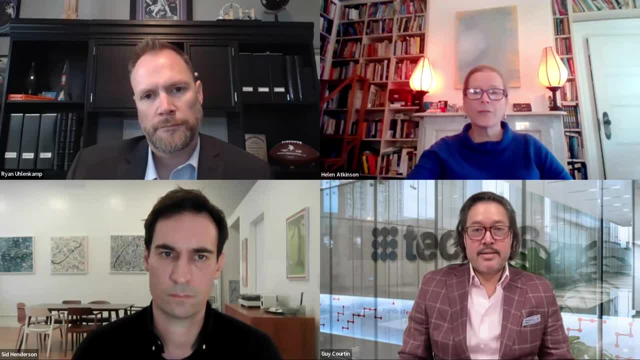 But I think the question is right. I think there's there's something to be considered. when it's, you know, do I take a certain type of automation And is that, well it may, on the surface, solve a problem? Does it actually limit some of the flexibility I have? 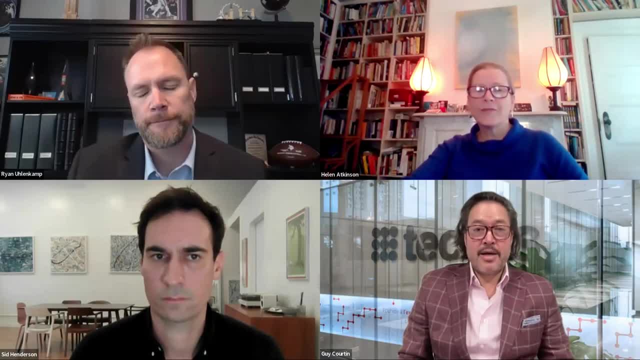 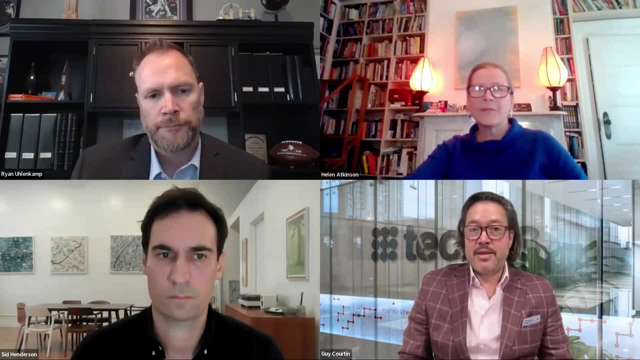 Or do I have the ability to do other things with my labor within that warehouse? And you know, I don't think there's there's a simple answer to that. I think that is a case by case situation, but it is absolutely something that anyone 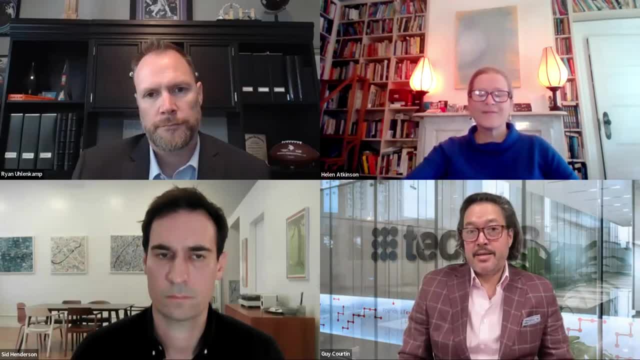 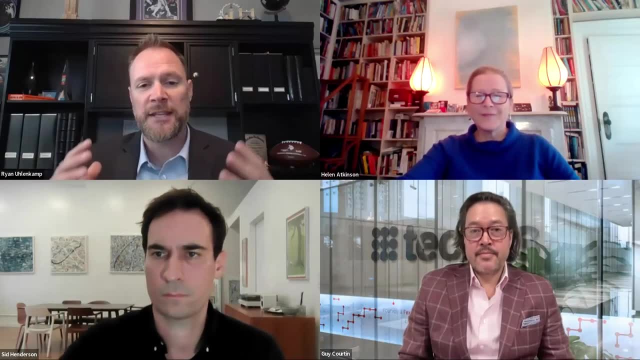 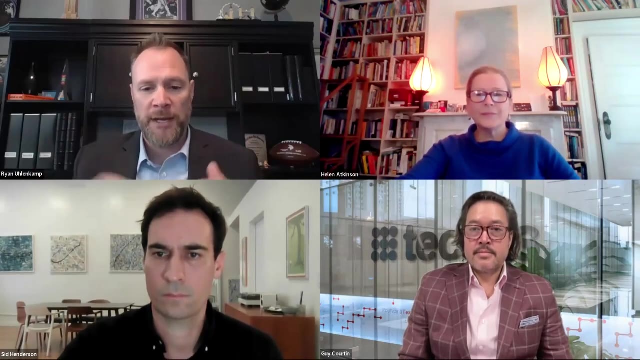 who's looking at automation has to take into consideration, because it's an unintended consequence that certainly could rear its ugly head. That's why I'm so big when I say hybrid, because I do think you need the consideration of both. right, How can I? you said it earlier, Guy. how am I planning for the future? 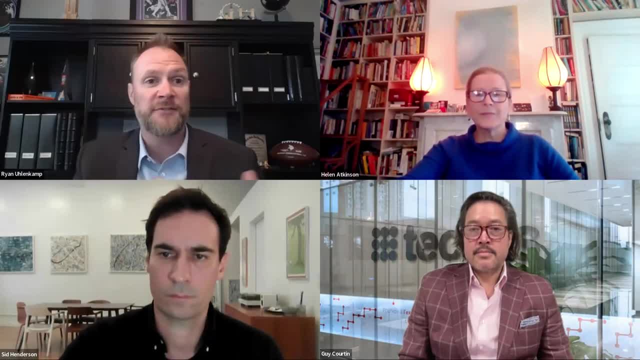 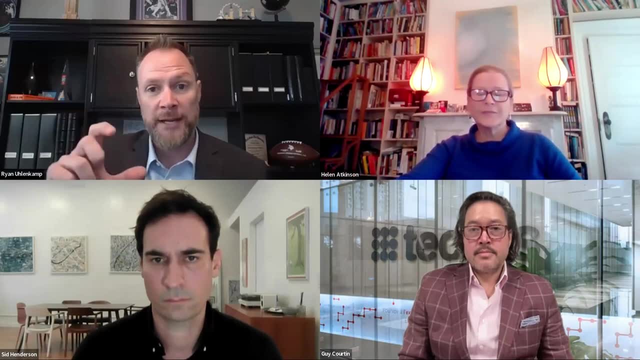 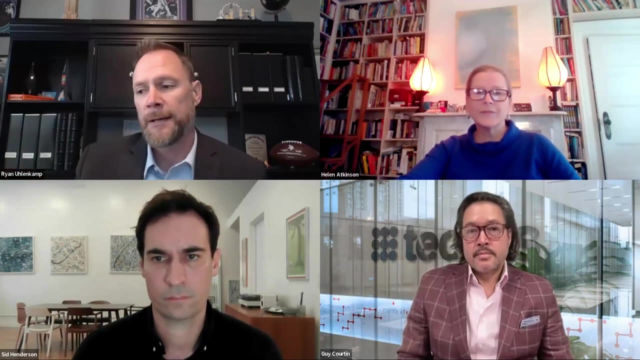 Right. How am I planning for the future Is: how am I planning for my warehouse to be resilient If something happens? how do I flex? So there is so much. I think that needs to go into selecting the right solution, and that solution needs to to take into consideration all those elements we've been talking about. 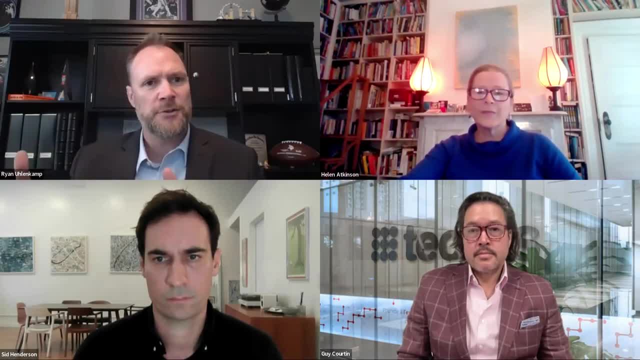 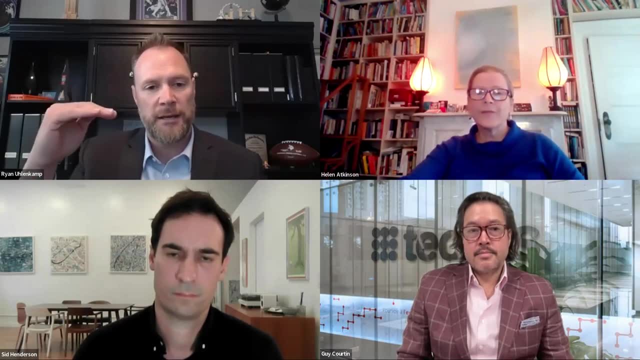 How? how do I make sure it's not a limiting factor in an area that's critically important to me? And if it is, how am I working around that? Because I only get so much scale right In an ASRS. I can do what it can do, which is fantastic, and it gives me consolidation. 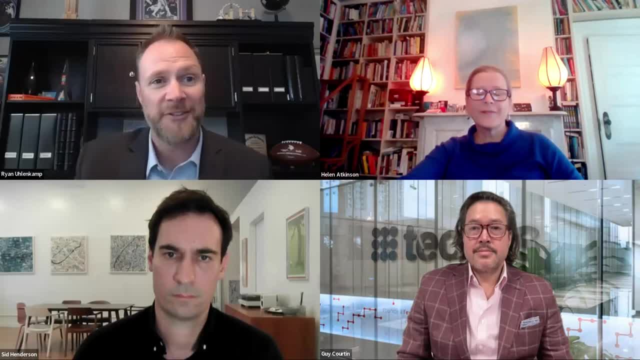 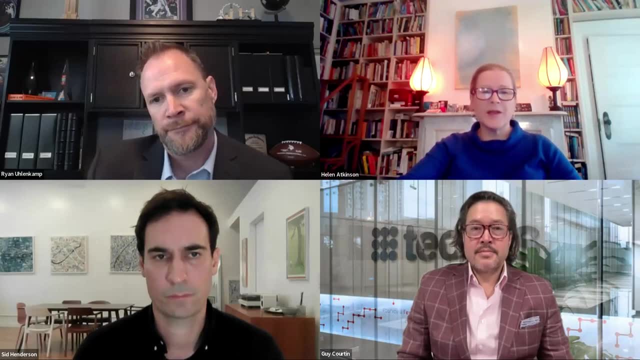 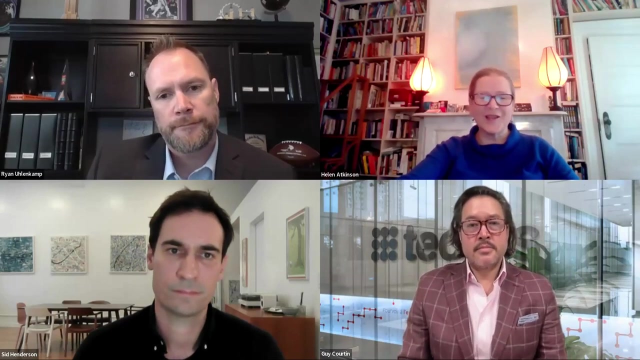 But what happens when I have a scenario where I have to get more right? Right, That's very interesting, And I you know, obviously, it seems to me that in many situations, automation increases flexibility- Fantastic, Yeah. So it seems like a lot of robots and automation technologies do the same thing to the to. 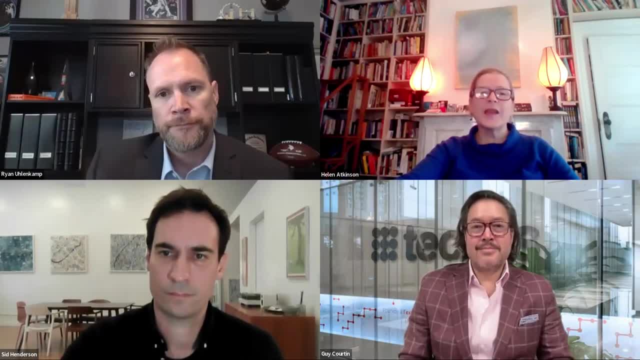 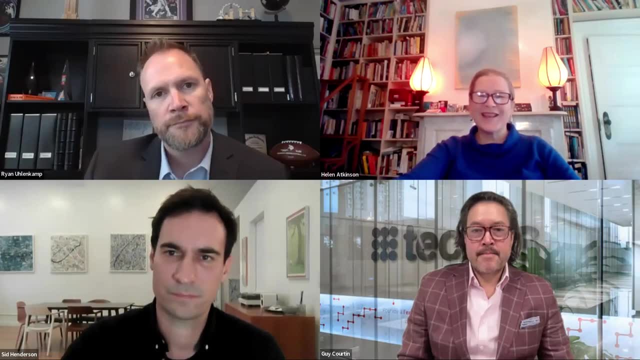 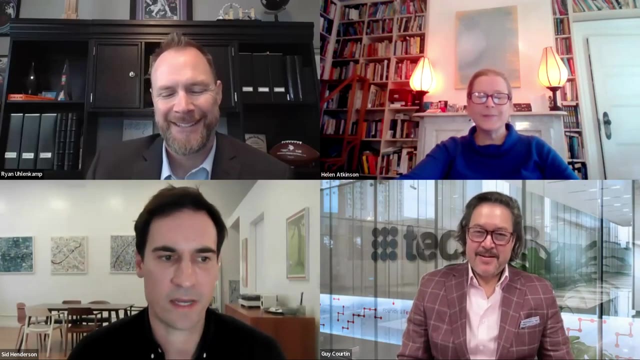 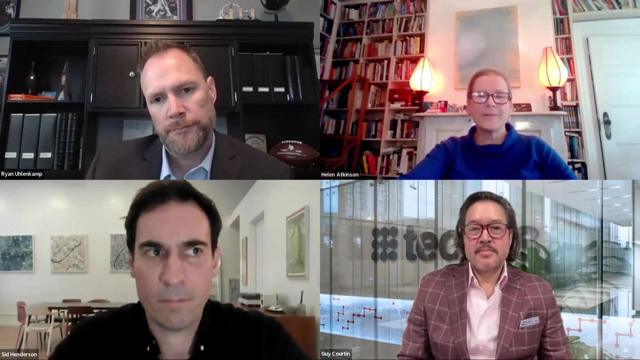 the naked eye, They might all look very similar. What are some of the key differentiators in the different technologies, Sid, maybe you can talk to that. That's a big question, You know. for us at Exotech we are trying to offer a solution that that really maximizes. 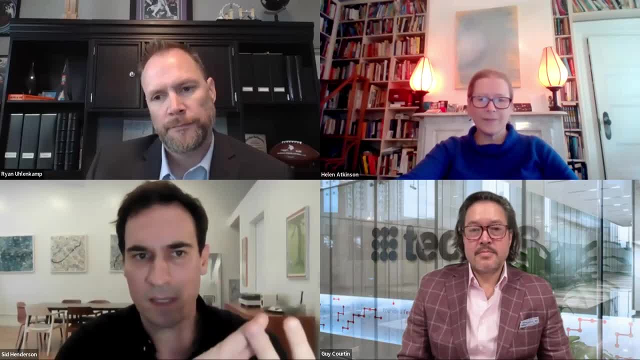 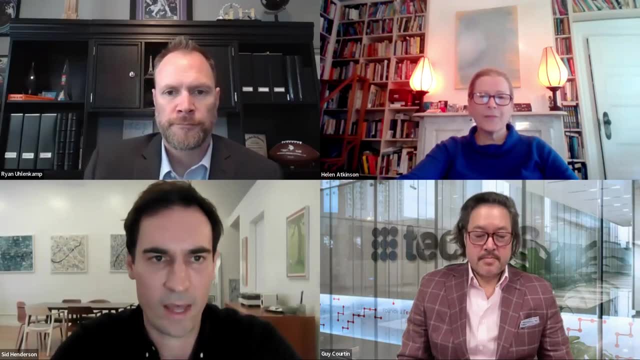 three things: Throughput, Density, Flexibility And throughput in terms of we have very fast robots and move in 3D and move at four meters per second. We can add more robots if we need more speed, more picking stations if we need more throughput. 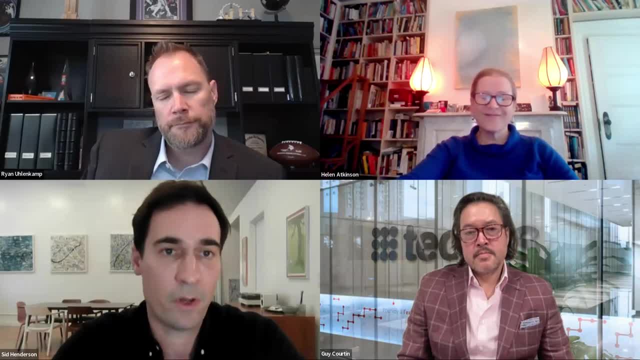 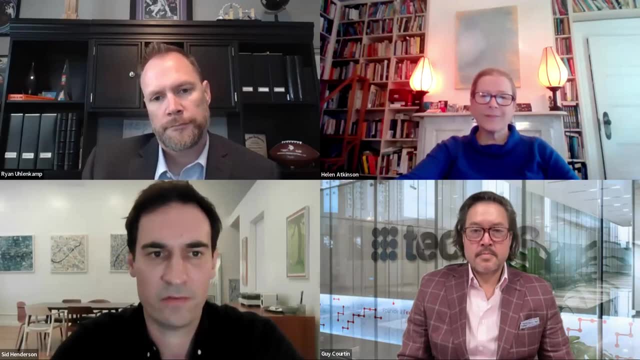 Our racks go up 39 feet, So you can really fill up a warehouse. And then flexibility just in terms of being able to add more robots, more racks as the demands change, But at the same time we have a lot of flexibility. 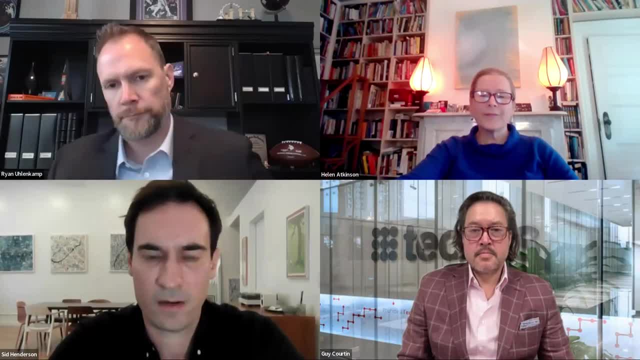 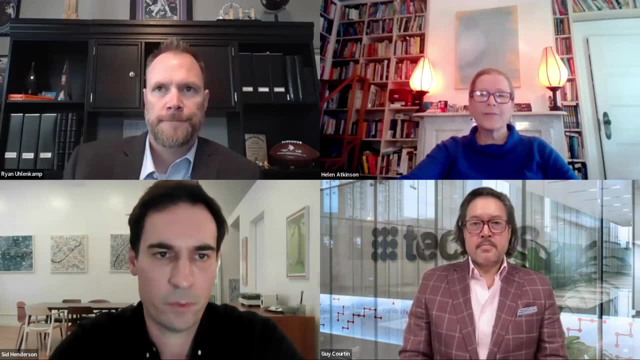 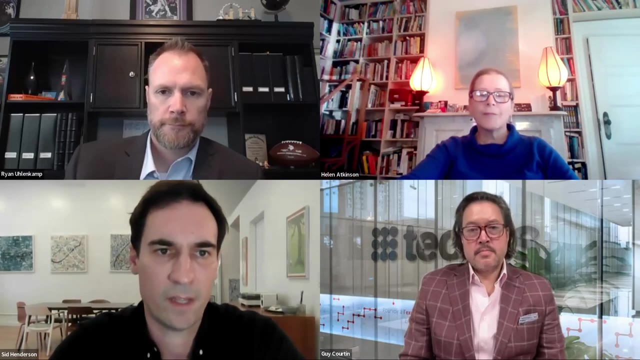 Yeah, So you know, different solutions have a lot of different strengths and different customers have different needs, So it's also super important to talk with a company like Texas, who can help you assess all the different technologies that are available and find the right one for you. 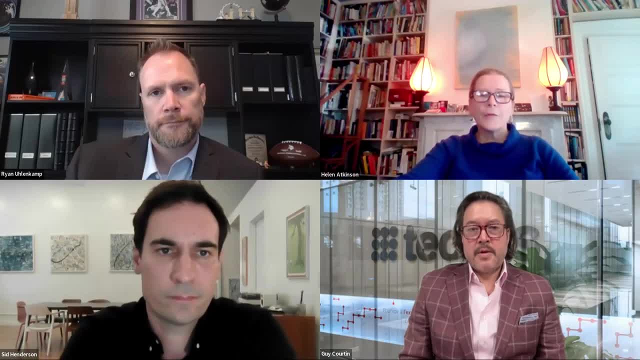 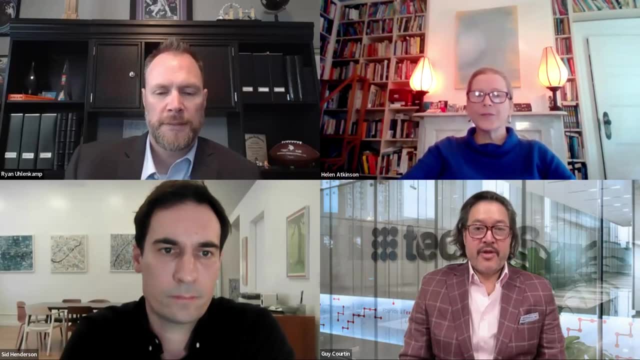 Yeah, All right, That's great. Yeah, Sorry, Just one way I build out what Sid said is: you know you need to look at what are your drivers- Flexibility. I think what Sid said throughput right. Those are all key aspects. 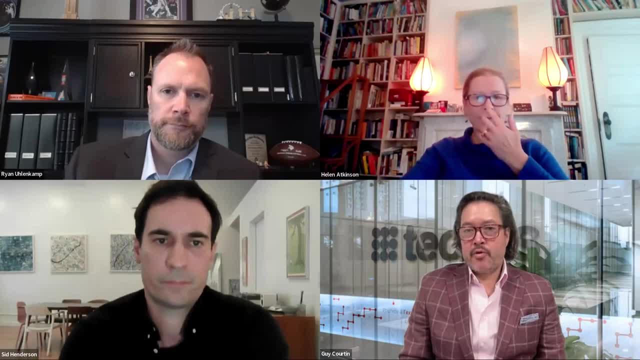 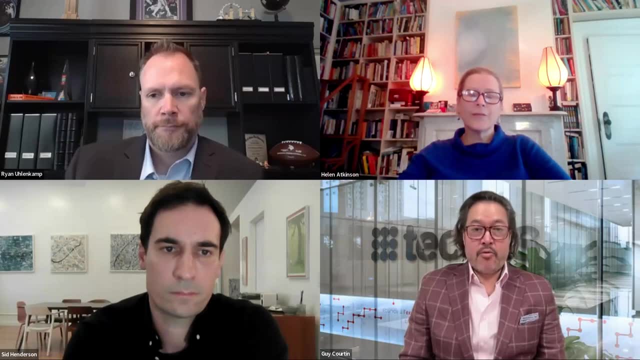 I would also say one aspect to look at is you know greenfield versus brownfield, right? Are you putting in a system into a pre-existing warehouse where you already have racking and space constraints, Or are you going in with a fresh slate right? 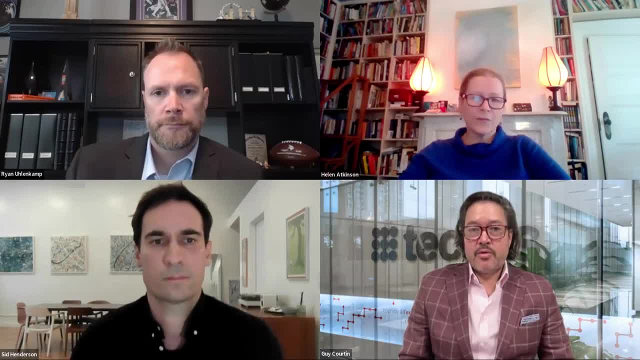 A brand new warehouse And that's also going to help you understand. you know what type of automation you want to go with And, to your point, I think you know. the challenge is that there's a you know for you know. 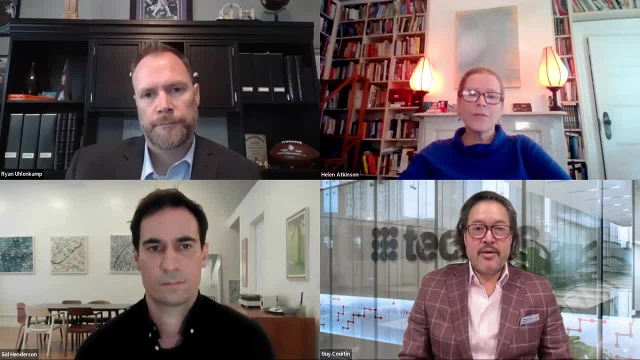 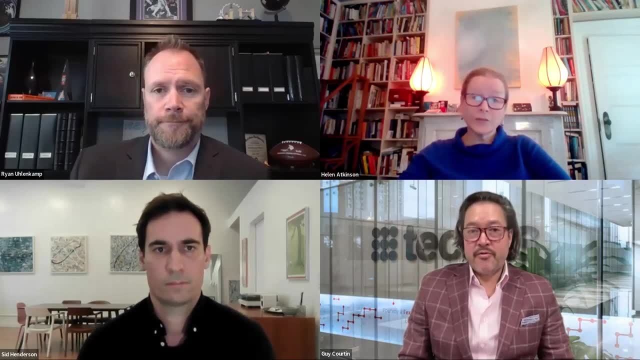 I think you know the challenge is that there's a. you know there's a. you know there's a challenge is that there's a. you know a last count: I saw there's close to 700 different automation OEMs out there offering a whole host of different types of robotics. 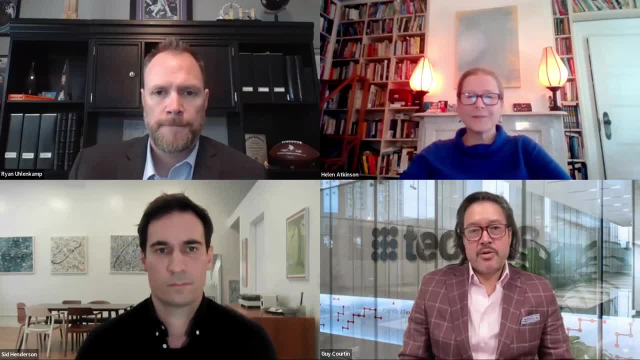 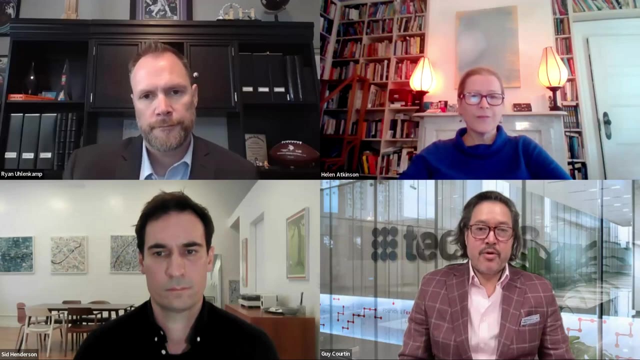 So, while the surface they might look kind of the same, a lot of them are doing a very precise or specific job within your warehouse. You know, Sid's solution is doing something that's very different than a fetch robot doing dung removal. So that's the other challenge is to, you know, dive in deeper with the automation. 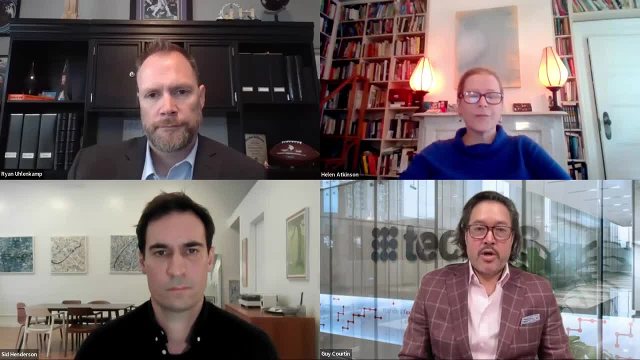 And then, you know, the second challenge is to understand the implications of that automation and what kind of solutions that you are going to be using. So one of the things that we've done over the last few weeks- you know we've been working- 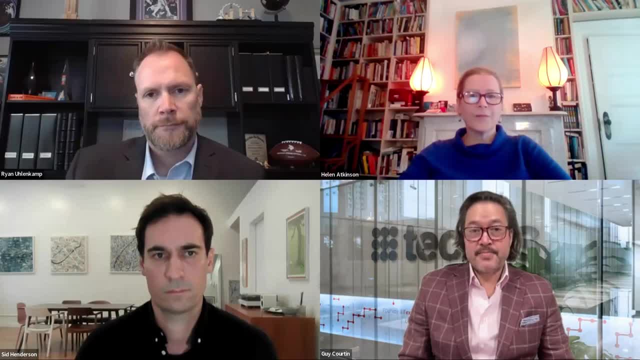 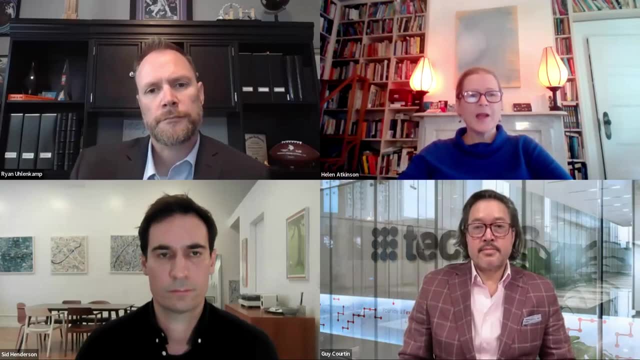 with a large group of players to understand what is it that they're servicing. What are you trying to do it back to Sid's point. you know, think about flexibility, think about throughput, think about what your long term plan is, because those are going. 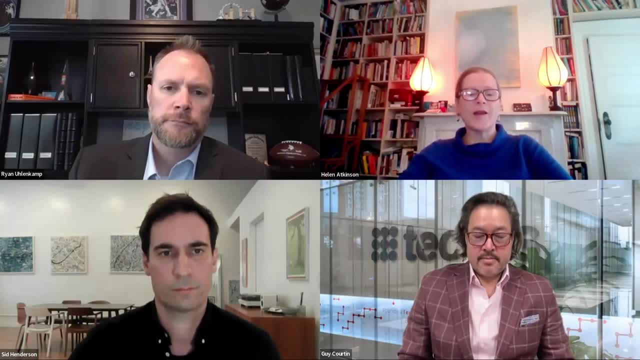 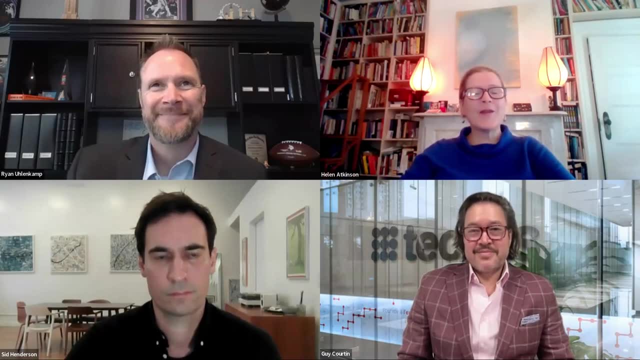 to be big drivers to that investment Right. So I just wanted to touch briefly on another issue of complexity, which is that you bundling automation with warehouse management systems, or should do? What are the advantages of a best of breed WMS versus a bundled solution, Ryan? 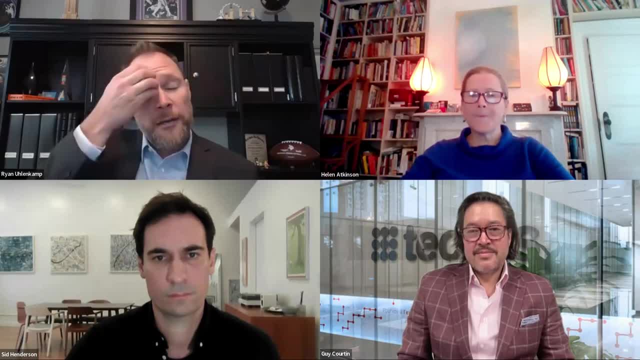 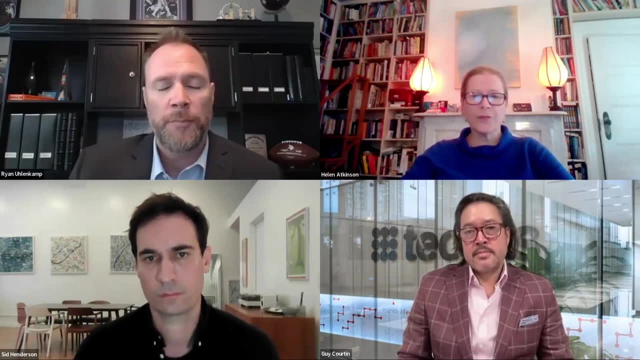 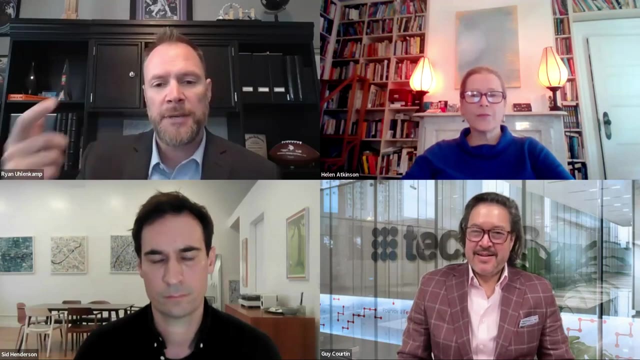 I think that's one for you. I think in any solution, selection, flexibility and scalability are key, right? So what? I keep going back. you keep hearing Guy and Sid say the same thing. right, You have to pick the right solution for you, So bundles can be. 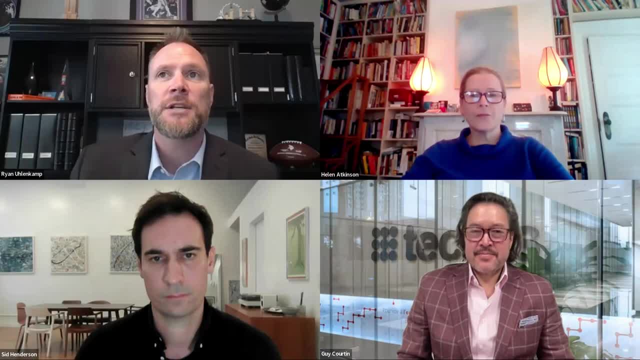 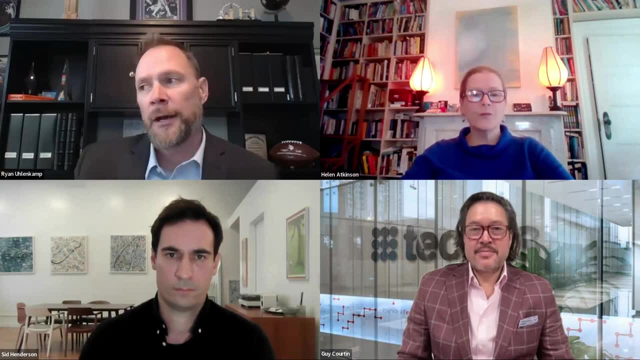 great and platforms are great and that streamlines integration. But a six-person cross-stock facility is very different than a thousand-person e-com facility. Honestly, a lot of customers don't have single WMS platforms either. right, They've grown through acquisition, So I may have a tier one over here. I have a homegrown over here, So I think whether 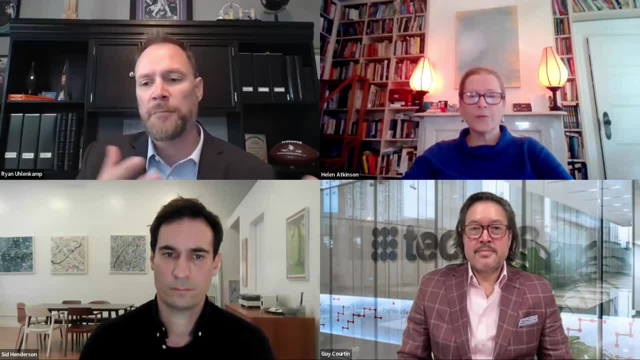 it's automation, labor management, any type of solution. when I have multiple, I have to have a way to bring all of that together, And I think that's one of the things that I think is really important. And I think that's one of the things that I think is really important, And I think that's. 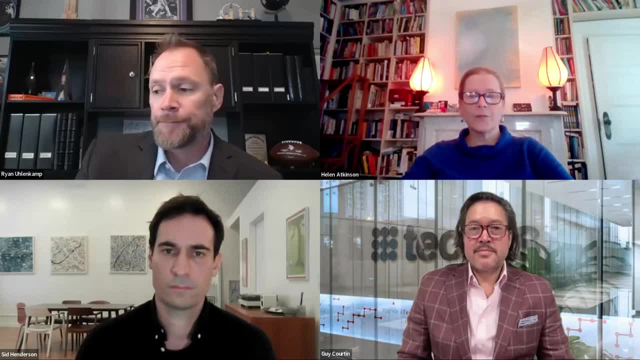 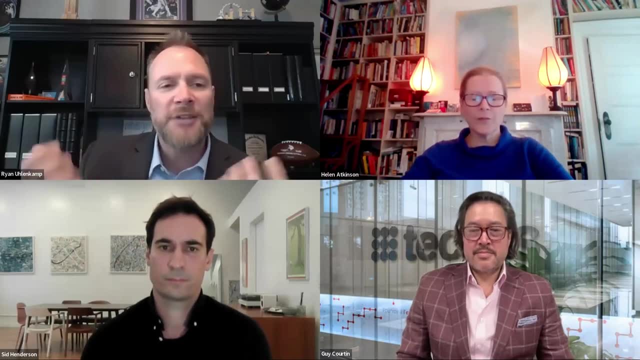 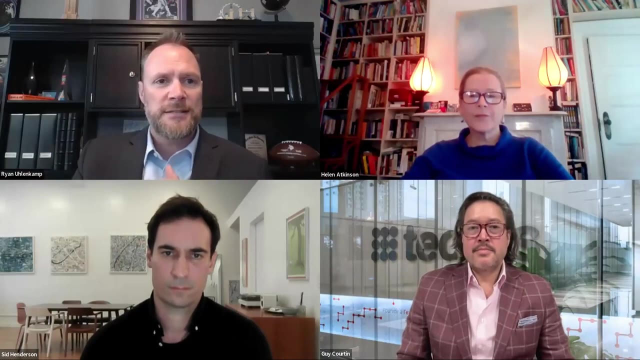 a lot of value in leveraging a best-of-breed solution in that instance where that's API-driven and easy to integrate with and can communicate and bring a similar cohesive experience across these whole systems- And we're talking WMS, but I mean think of ERPs and time and 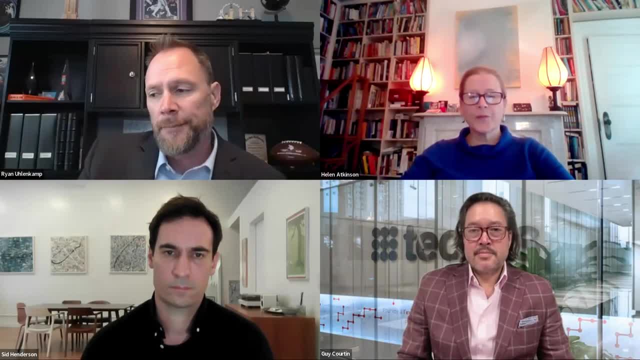 attendance and all of these that we want to start to feed into. The more you branch that out, the more systems you touch. Platforms are great- I'm not denying it- And if it fits for you, but I think there is a value for. 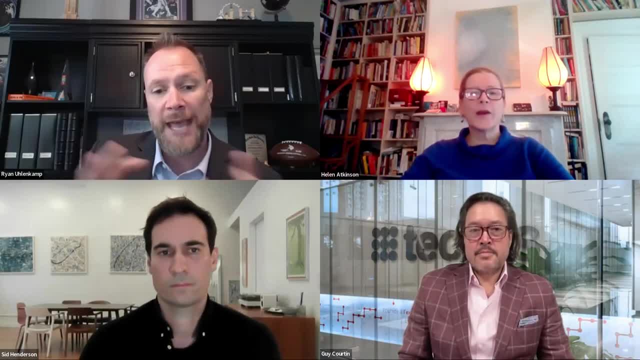 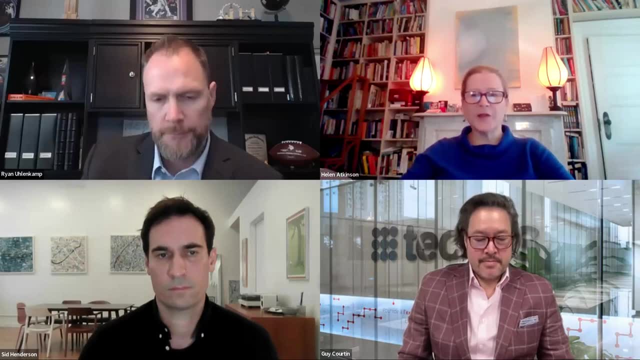 flexibility, scalability and a best-of-breed solution for that kind of scenario. And this very much speaks to the issue of data and the enormous amount of data that there is to manage. Wonderful, This is all great, but we're running out of time. 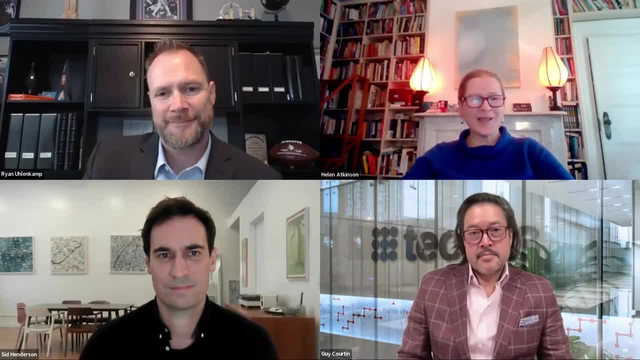 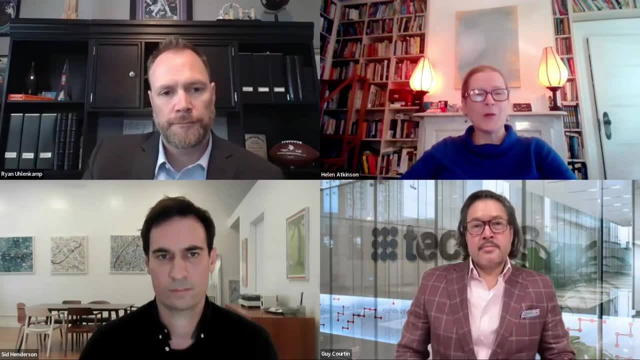 We're running out of time. We have time for just one last question, And I'm going to pitch this to Guy from Texas. Guy, if the warehouse of the future will be a combination of human labor and multiple types of automation, 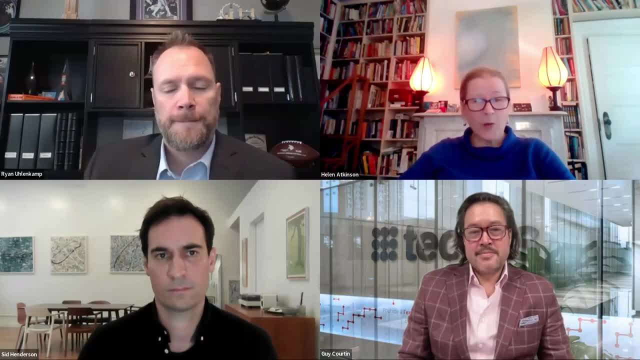 how do we ensure that not only does the human element work in tandem with automation, but that the different types of automation play nice with each other as well? Yes, play nice in the sandbox, right as we tell our kindergartners to do. 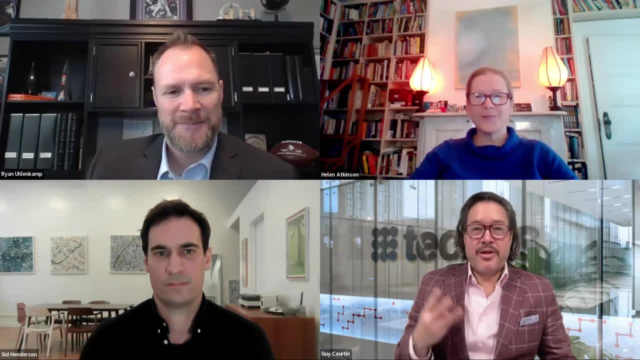 Alan, that's the million billion-dollar question. So I think there's going to be sort of three things people should think about. One: interoperability, And what does that mean? What does it mean to you? What does it mean to you? What does it mean to you? 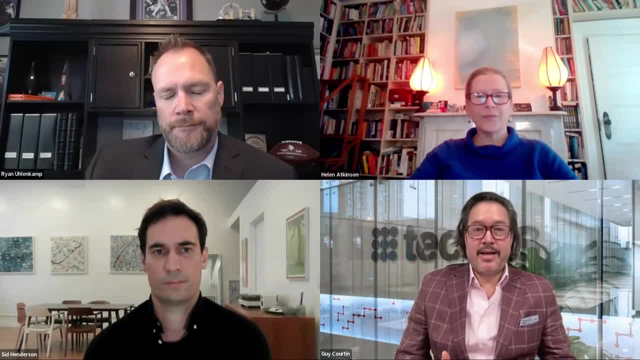 How do we get all these robotic systems to play nice in the sandbox? right, That is going to be key Two. it's going to be around the labor division between automation and the humans. Humans are still going to do things much better than any robot can, And robots are going to do. 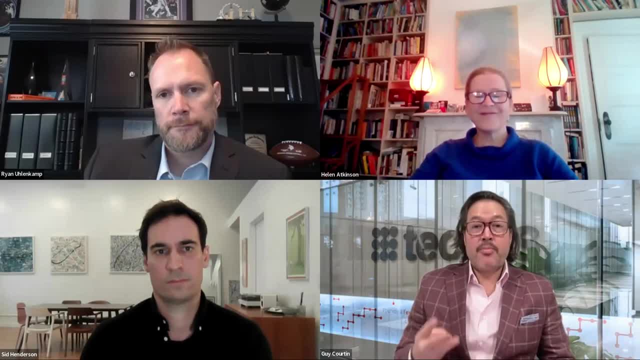 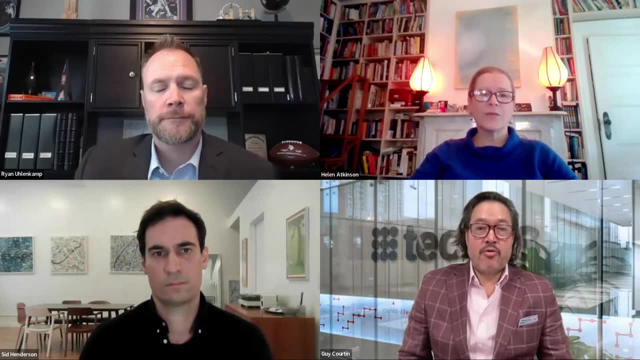 things that we, as humans, don't want to do anymore. And the third part- I think we've touched upon it during this and I think Rai talked about it- is really this change management right. How does that impact your overall business, Not just in the warehouse, but your logistics, your 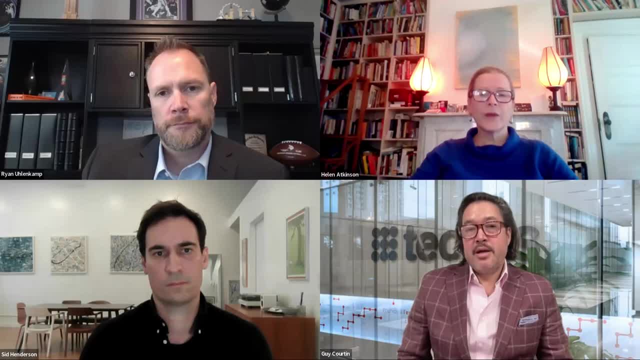 fulfillment, your supply chain, everything outside the warehouse. So for me, when we look at it, to make sure that as we move forward we all play nice in the sandbox, we take advantage of the robotics that we work well in the warehouse, we've got to focus on those three. 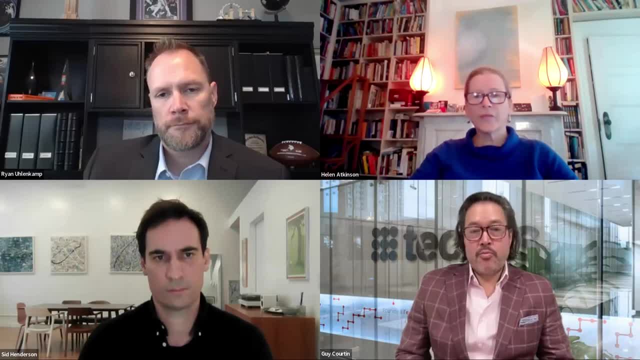 things right: Interoperability, the division between human and robotic labor and the change management that's going to have to come, regardless of what path you go down, Right? Thank you, Guy. That was a great answer. I'm afraid that's all we have time for. Thank you. 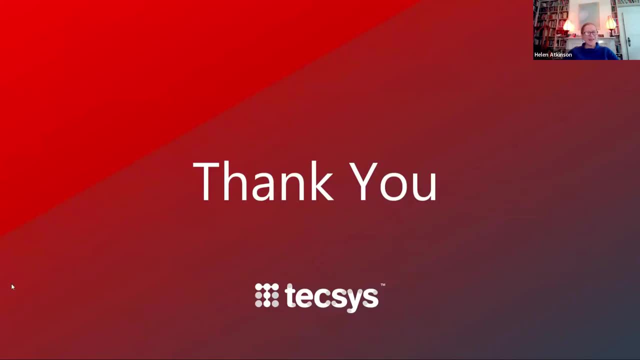 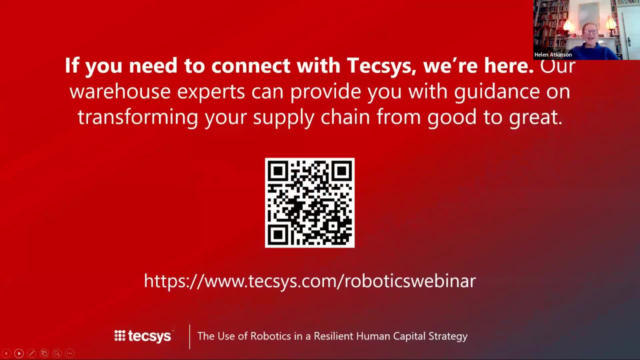 so much. Thank you so much to Guy from Texas, Sid from Exotech and Ryan from Longbow Advantage, And a special thanks to you, the audience, for participating. I think we've learned a lot about how to make sure humans and machines can work together for better outcomes. We had a lot. 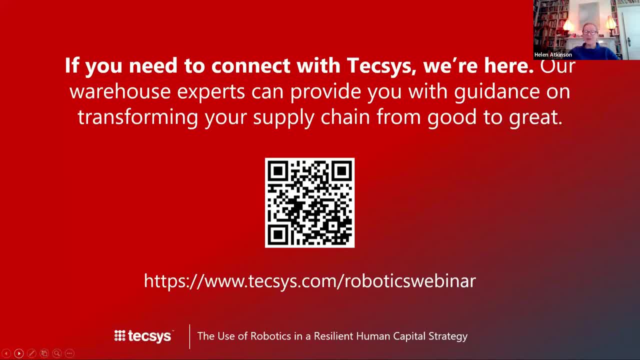 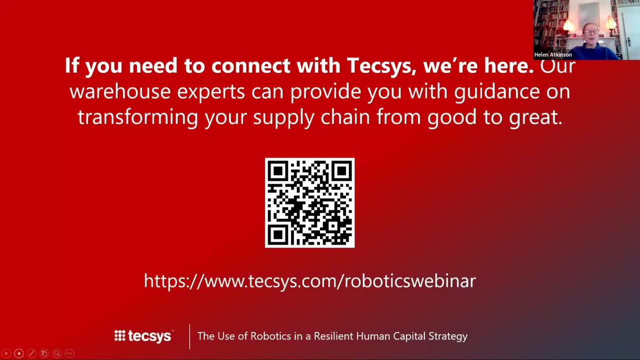 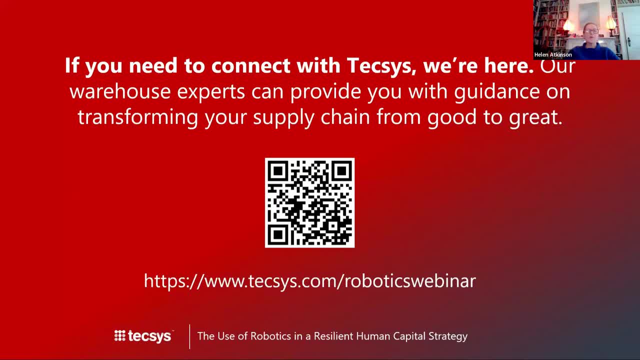 and a Texas blog I want you to chew on there, As well as a link to view the webinar on demand, which you can share with anyone, And there will also, of course, be contact information for Texas. Thank you so much to everyone for your participation. Stay safe. Stay happy And enjoy the rest of your day.